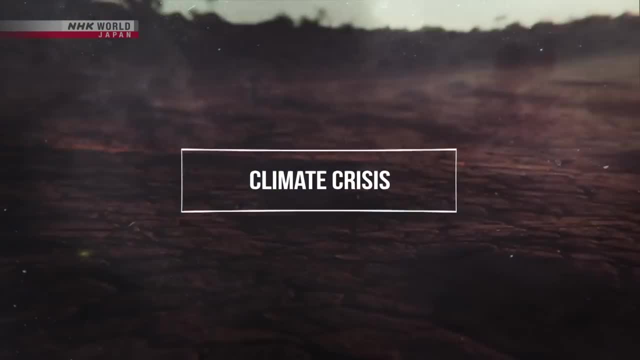 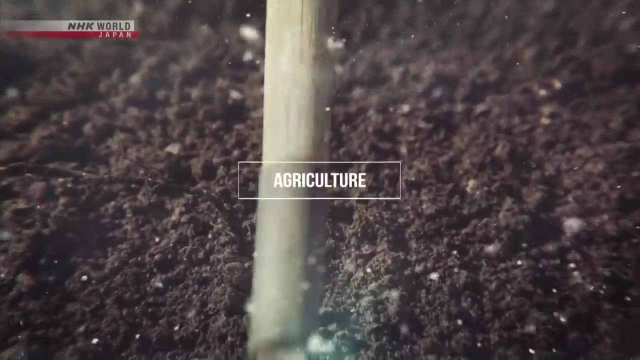 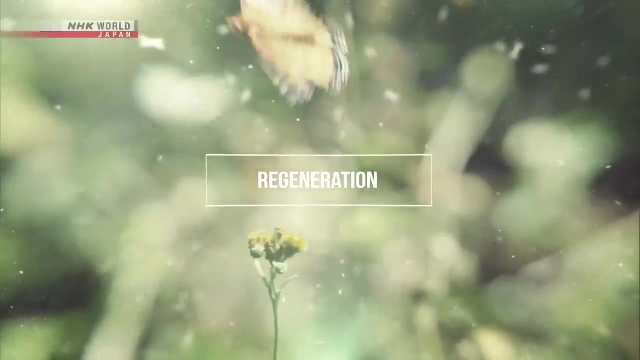 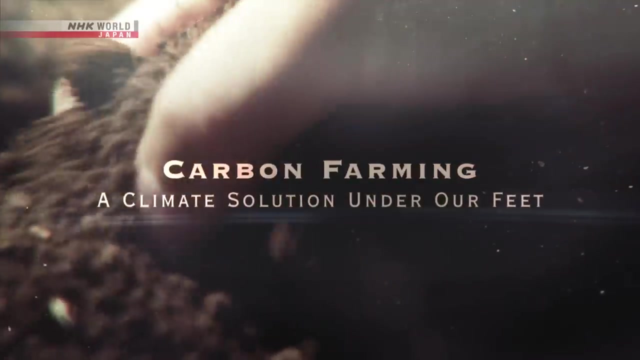 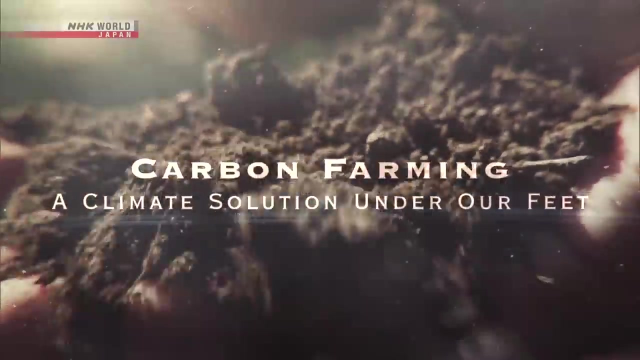 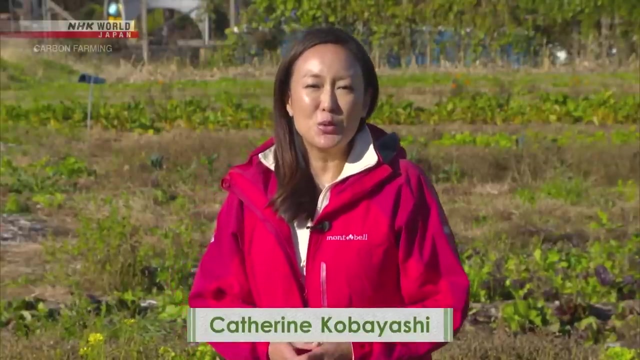 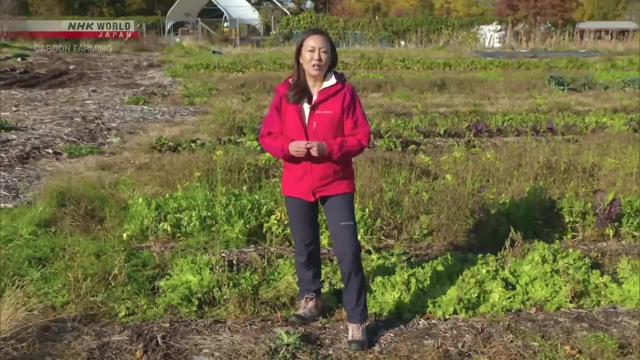 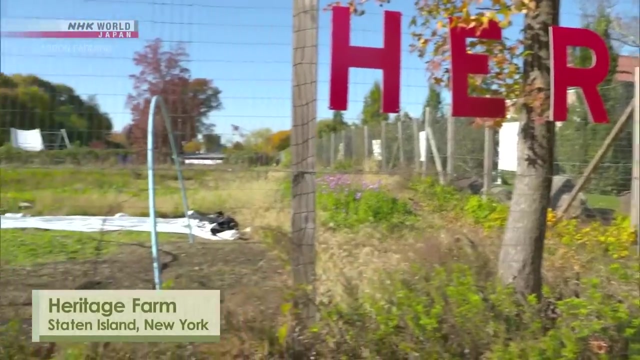 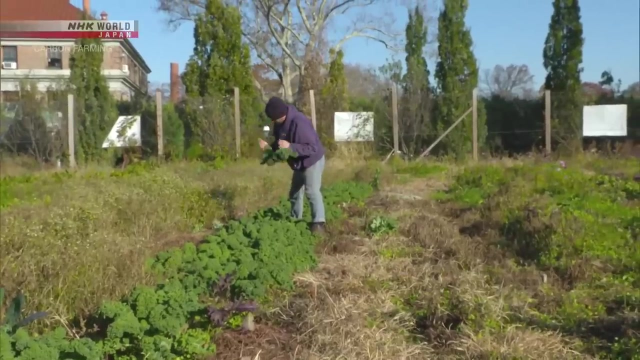 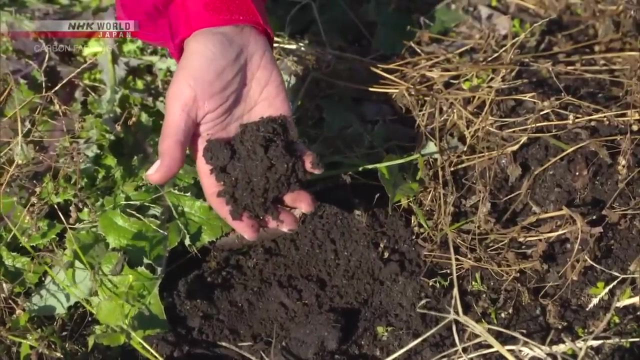 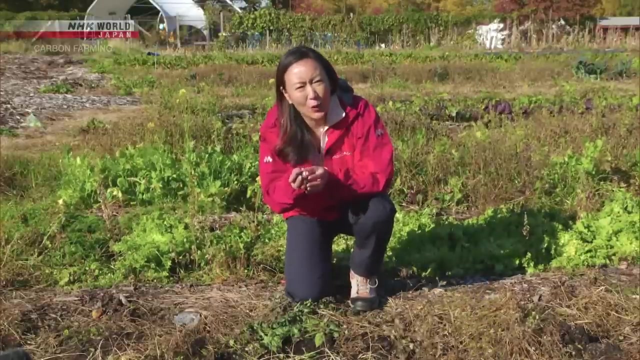 Thank you for watching. Thank you for watching. Let's take a look at the soil. It's dark, kind of like rich chocolate, And it smells clean, fresh and earthy. That's because the soil here contains a lot of carbon. 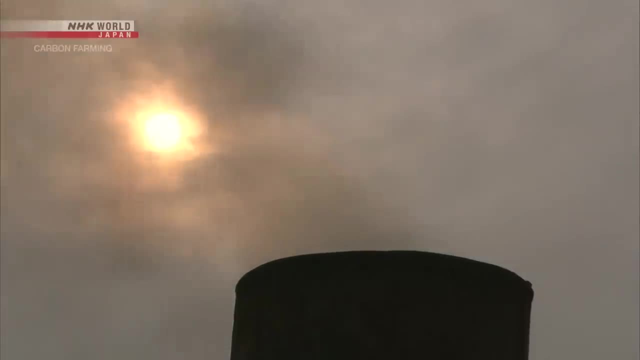 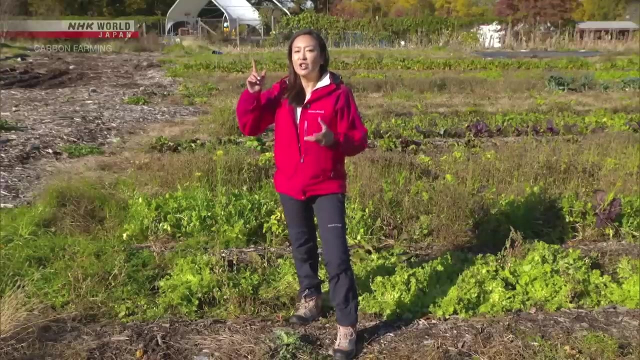 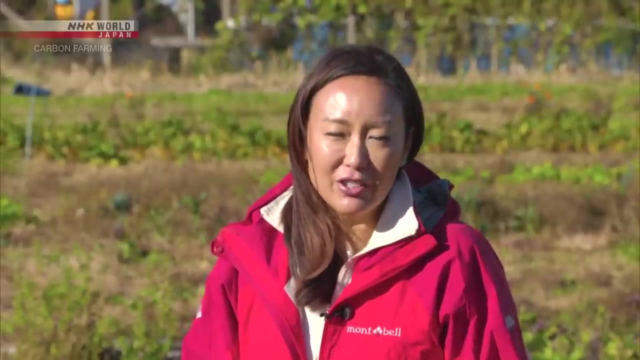 Carbon is often villainized in the climate conversation, but it may hold the key to tackling the climate crisis. Today, more and more farmers are utilizing carbon that's in the air to enrich the soil, which, in turn, produces more nutritious food. Some call this regenerative agriculture. 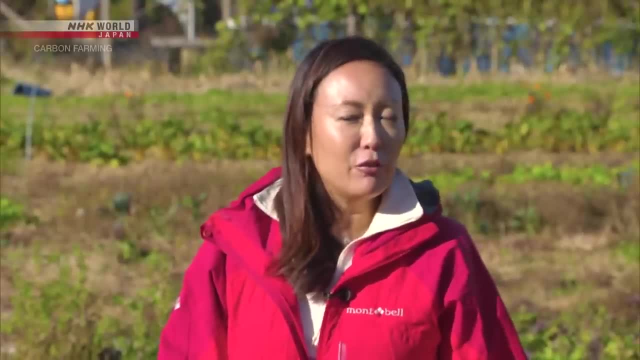 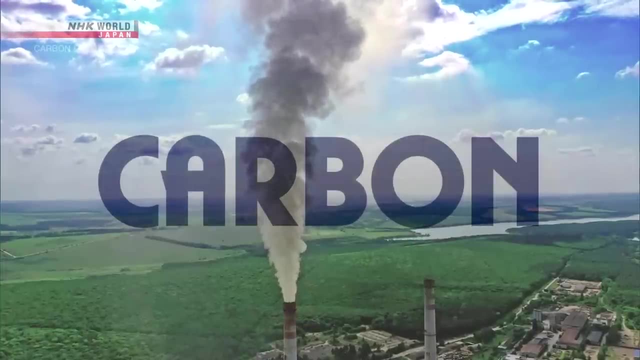 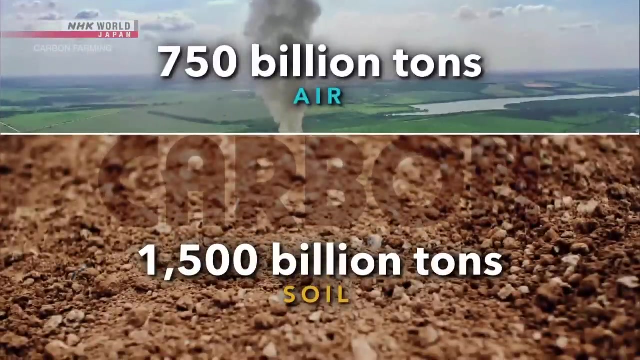 Others call it carbon farming. It's a paradigm shift from conventional agriculture and food production. Earth's atmosphere contains 750 billion tons of carbon And there's twice as much carbon in the soil- 1,500 billion tons of it. For thousands of years. human activities like deforestation and cultivation 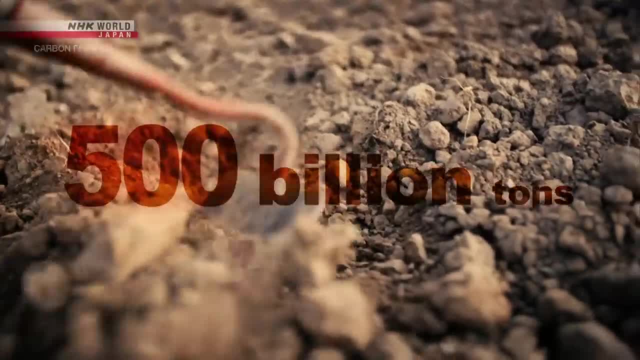 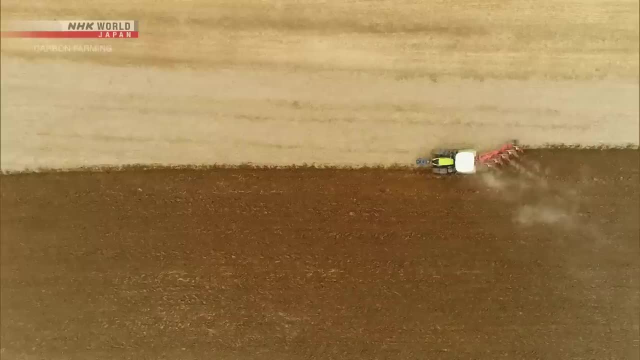 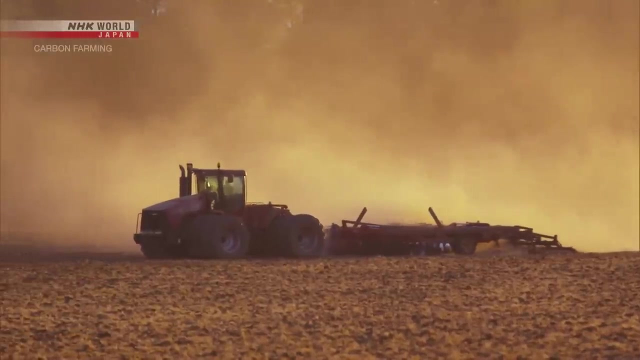 have released 500 billion tons of carbon from the soil into the atmosphere. Modern industrial agriculture has accelerated the pace of carbon emissions that contribute to the warming of our planet. And it's not just about carbon, it's about the environment. And it's not just about carbon, it's about the environment. 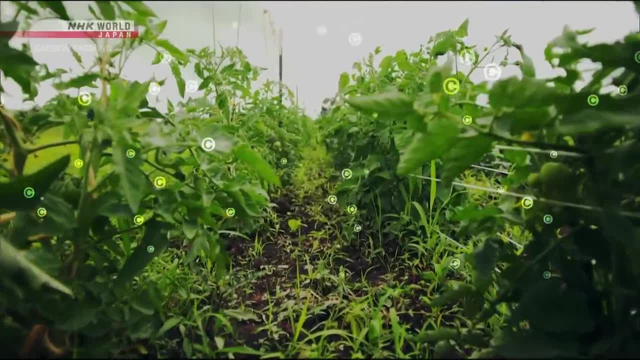 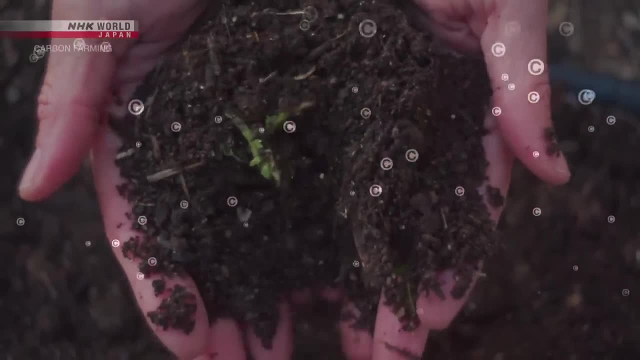 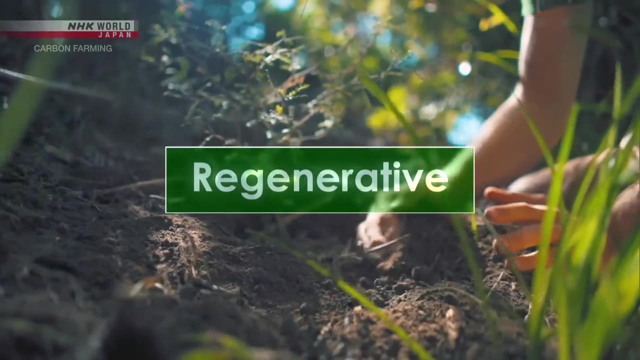 But carbon farming, or regenerative agriculture, can shift the trend, offering a way to put the carbon in the air back into the soil. The operative word is regenerative, as the methods help restore the soil and revive the natural ecosystem. Efforts to adopt these methods are now spreading around the world. 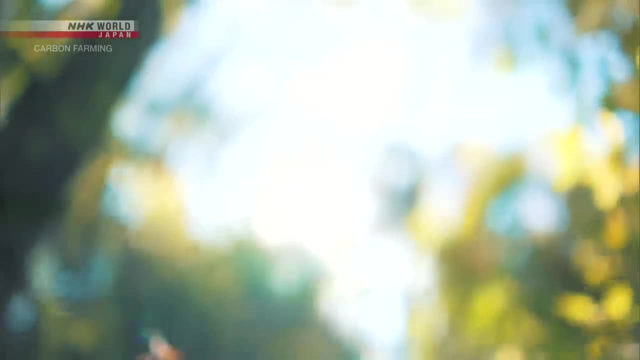 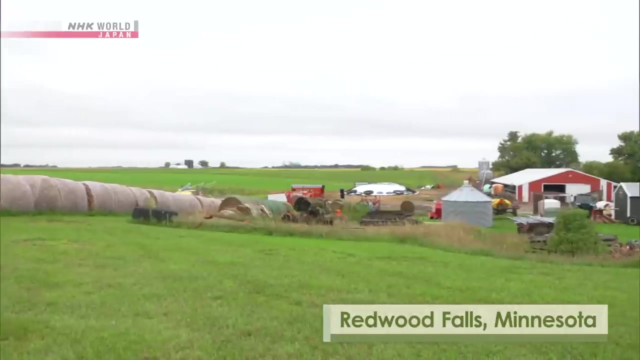 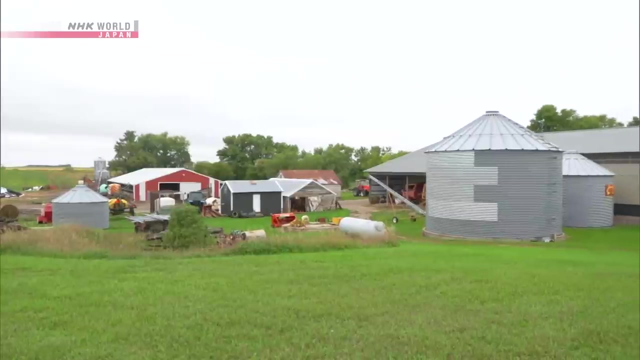 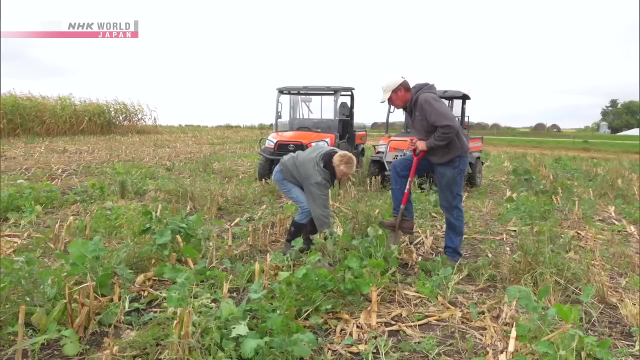 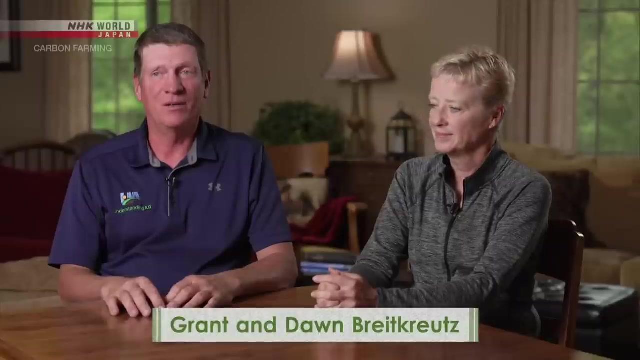 and are spreading worldwide. The so-called Corn Belt region of the US is a hub for the world's agricultural production. Grant and Dawn Breitkreutz are third-generation farmers of this land. They practice regenerative agriculture. We own and operate Stony Creek Farm here in southwest Minnesota. 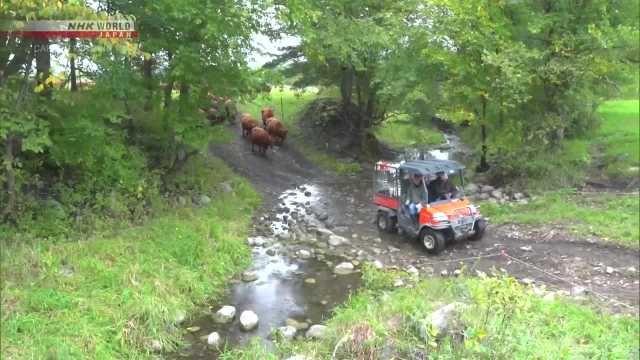 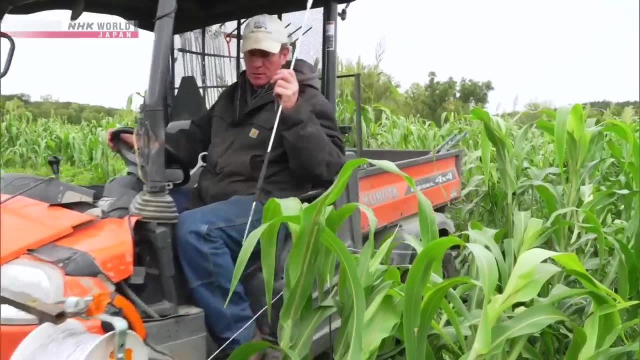 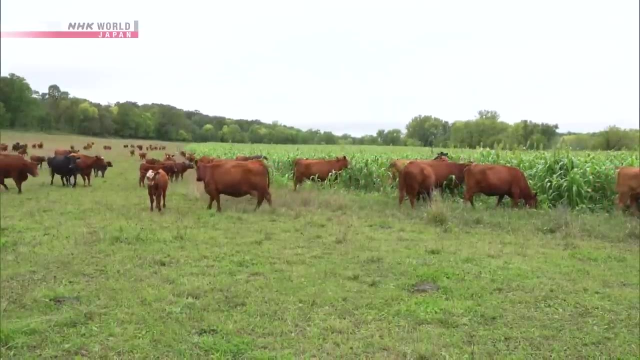 along the Minnesota River. We operate about 1,400 acres total. here We put in the corn, soybeans and other grains. We have our protein meat sources. we have a cow-calf operation. You know how long have we been on the regenerative path? 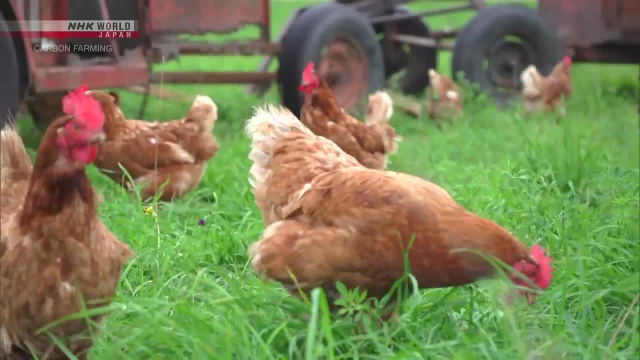 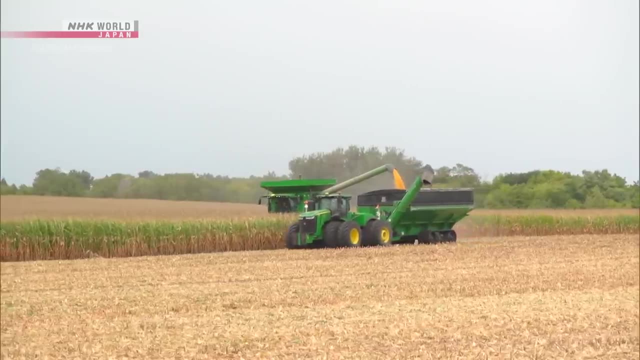 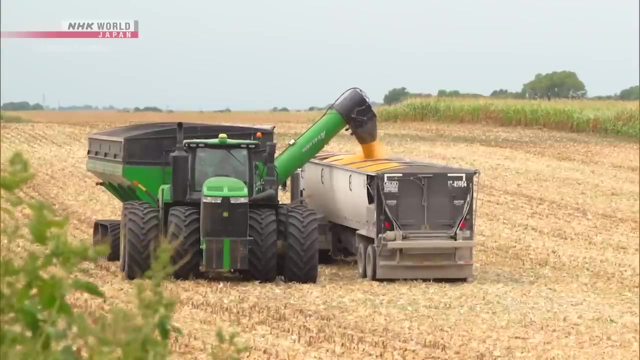 Intentionally, probably the last 10 to 12 years. Let's call the cameraman. In this region, many farmers rely on industrial agriculture. Overheads like fuel for machinery, as well as fertilizers and pesticides, weigh heavy on their income. 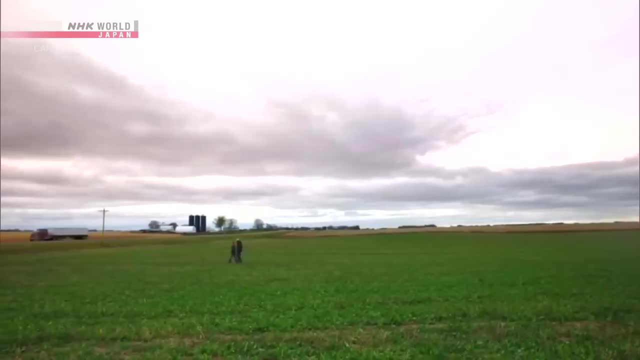 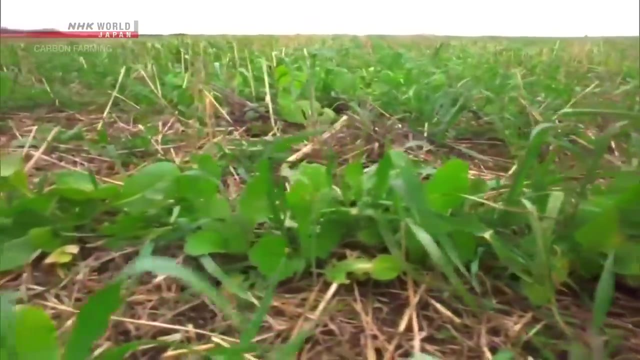 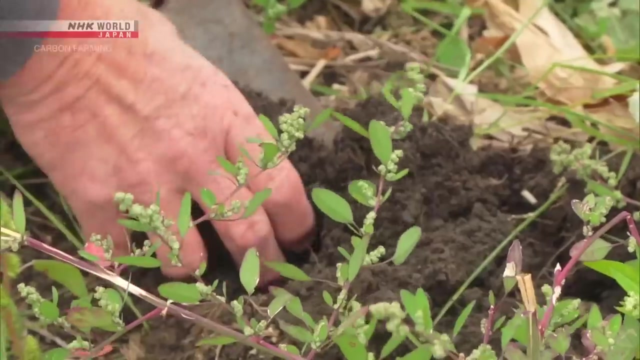 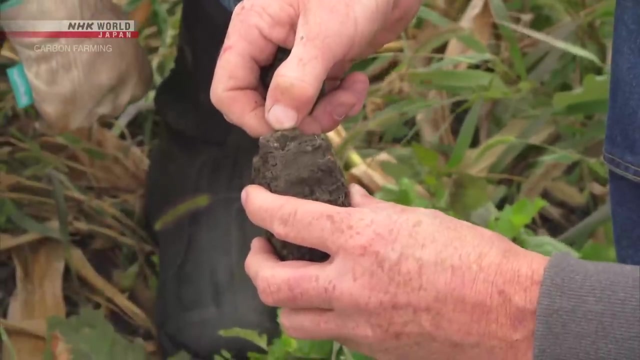 Seeing their profit margin diminishing every year, the Breitkreutzers turn to a method that doesn't require tilling or chemicals. Instead of relying on chemicals and human labor, their method focuses on regenerating the soil by working with nature. This is the color our soil used to be, and now we're turning it black. 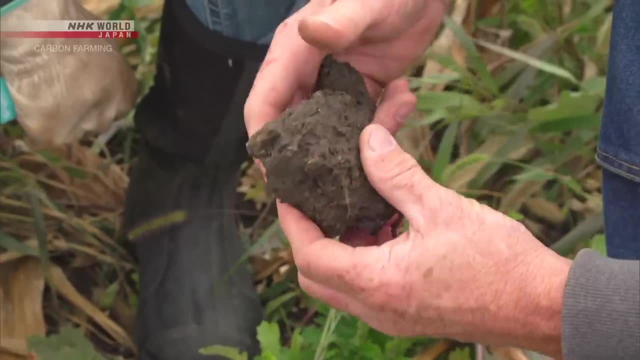 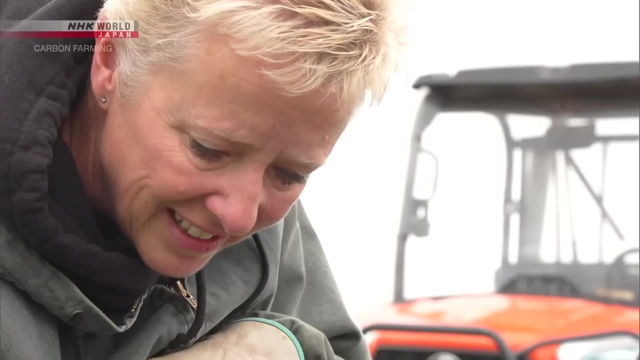 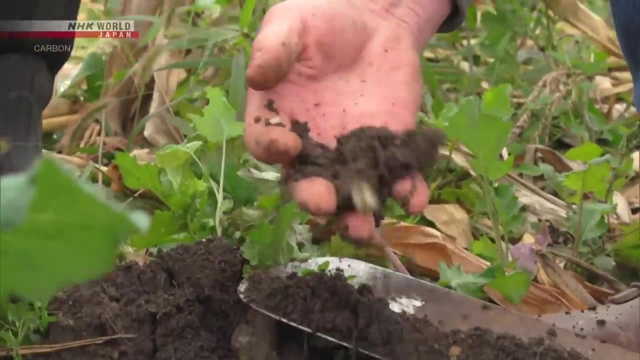 This hill would have been all that color, that yellow clay, and now we've turned it to black topsoil. Wow, Even this field- It's awesome- Looks like chocolate cake. So you guys come out and check these fields often. 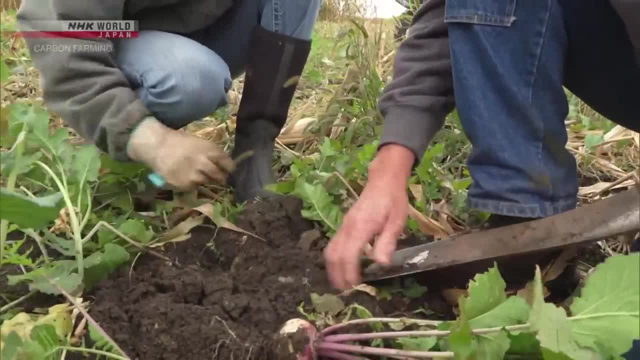 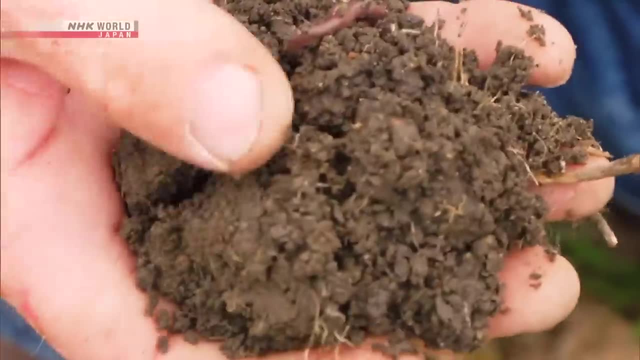 Yeah, especially now that it's started raining All the time. Now that it's started raining, we're out here all the time Just looking for our aggregation, looking to see if the biology came back. and by biology, the simplest way for us to look for biology is just earthworm activity. 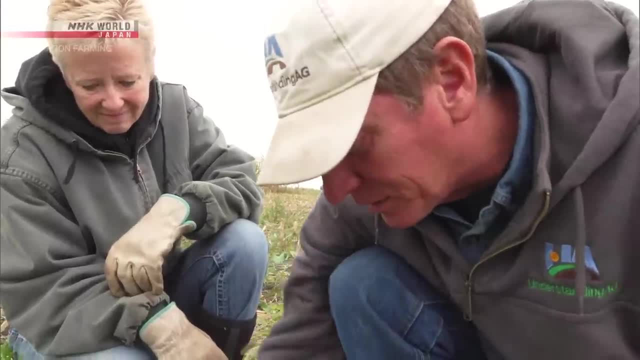 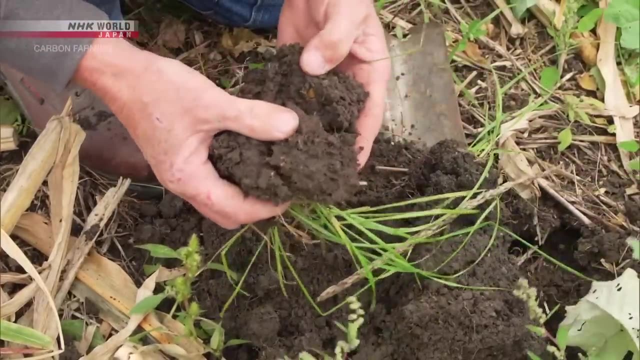 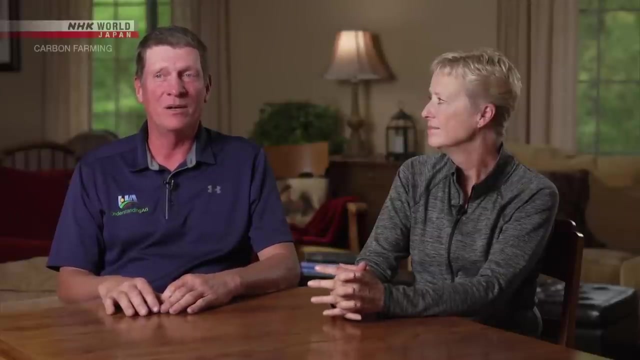 That's what we look for. Obviously, they're back here working away. The couple has been reaping the benefits of carbon farming. Obviously, 2018-19,. we came through some very wet years and we used to lose a lot of crop on this farm to wet spots. 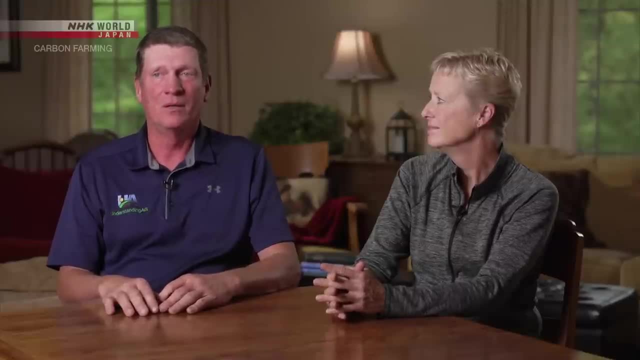 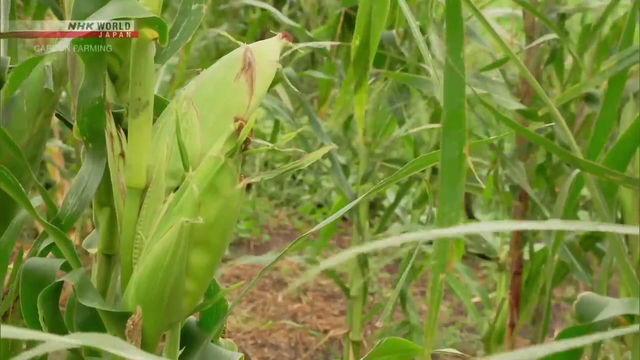 you know that would drown out. We lost nothing. Our crops will just about always be harvestable, whereas some of our neighbors are dealing with flat corn, twisted corn, that type of stuff. There's a lot of benefits to healthy soil. 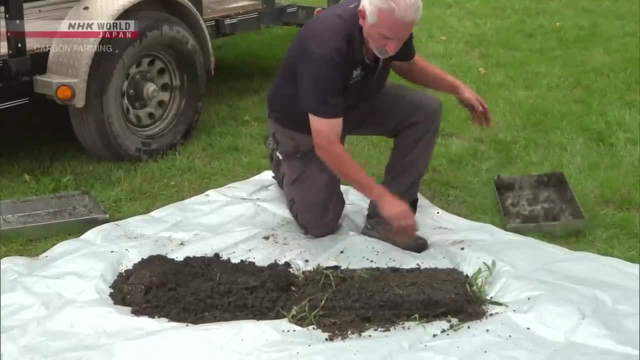 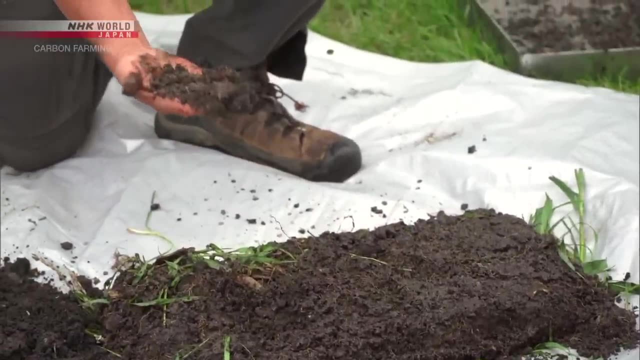 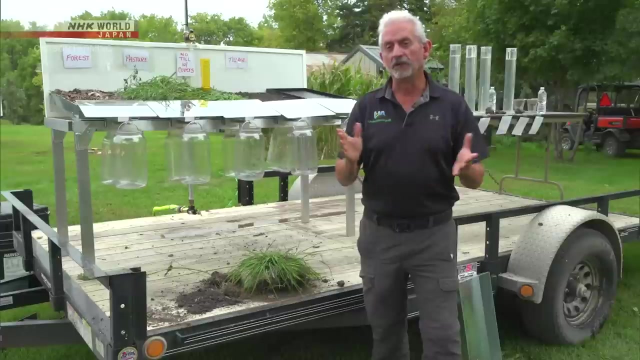 What's different about the soil at the Breitkreutz's farm? Soil expert Ray Archuleta tells us about its secret. Hello, my name is Ray Archuleta. I'm a retired soil health specialist. I retired with the USDA NRCS. 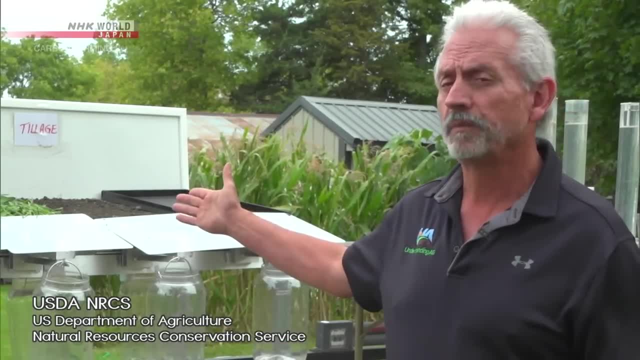 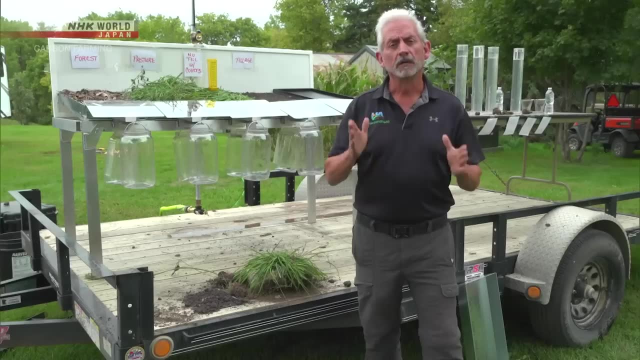 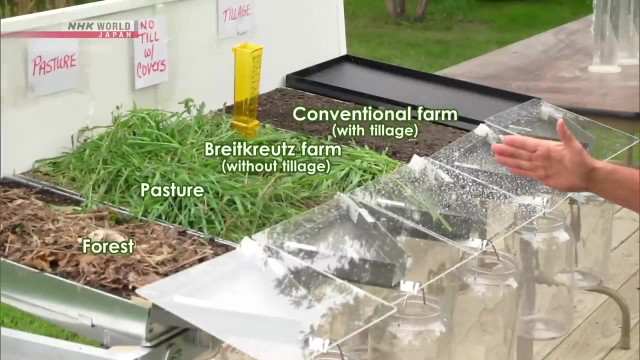 What I'm going to show you here is a rain simulator. This basic, crude model will show us how powerful functioning soils are. Archuleta will compare different soils taken from a natural forest, a pasture, the Breitkreutz's farm and a conventional farm. 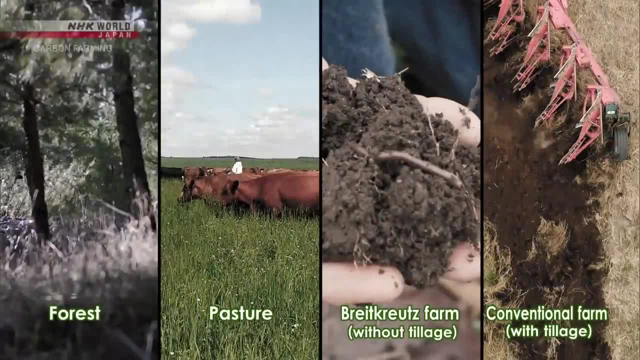 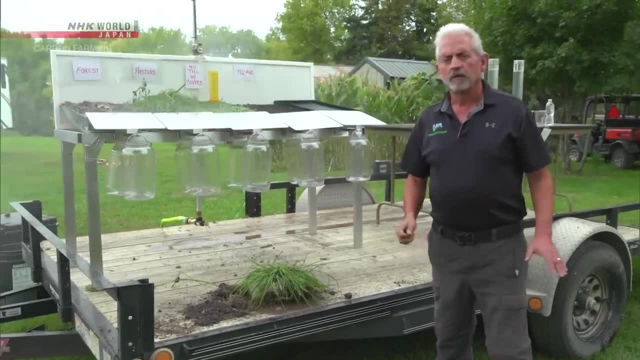 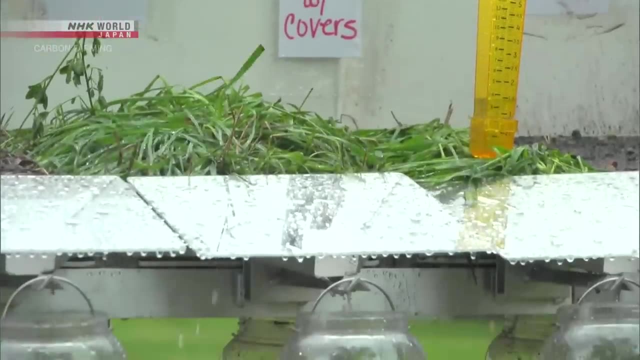 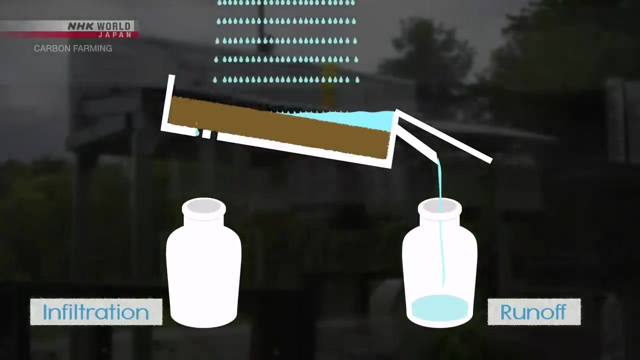 We'll see how much water each type of soil can hold and how much it allows to pass through. The bottles in front capture the water that doesn't soak into the soil and runs off, and the bottles in the back catch the water that passes through or infiltrates into the soil. 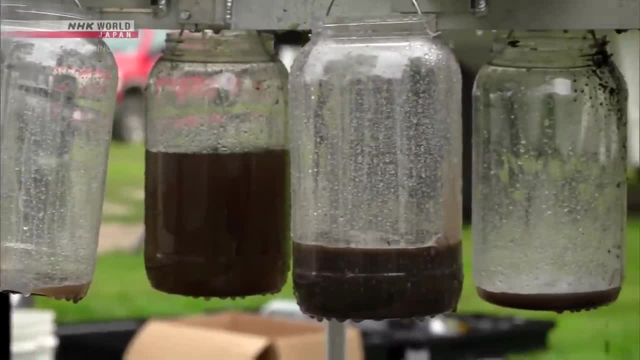 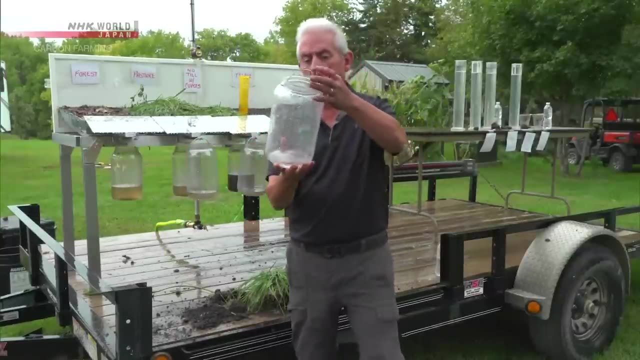 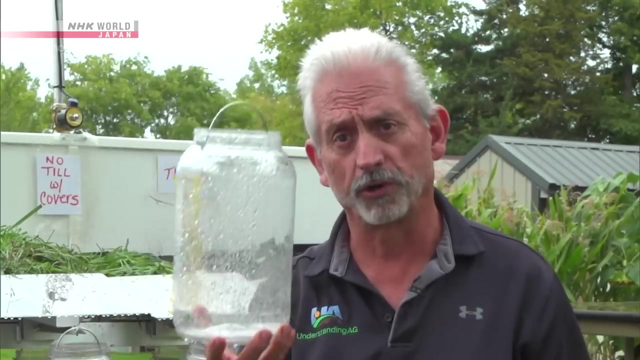 The bottles in the back catch the water that passes through or infiltrates into the soil. So let's start from the forest soil. We applied an inch of rain and look how much ran off. Very little. That is excellent. That shows that the forest soils are infiltrating and the soil is functioning. 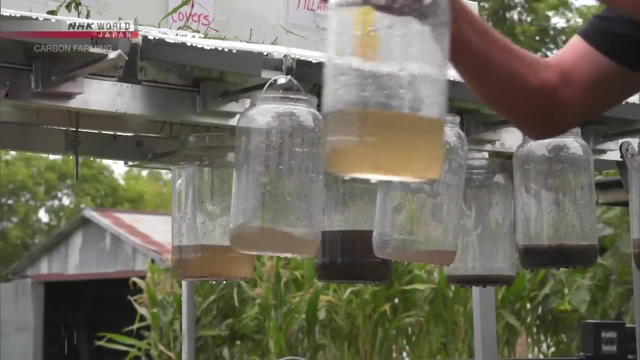 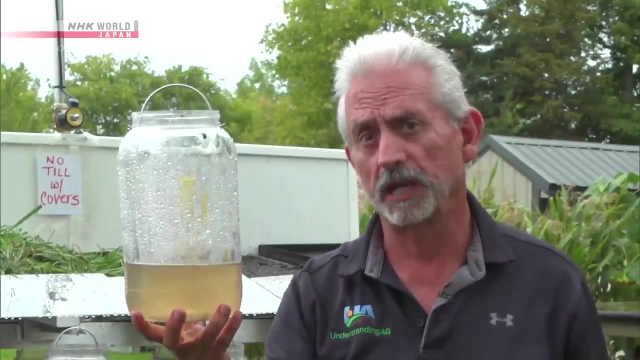 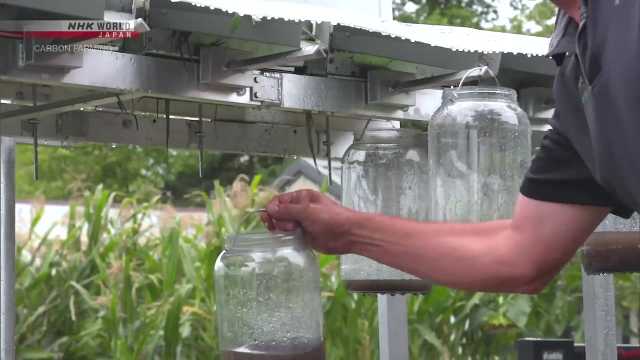 Now look at this forest soil. Look how much water infiltrated into the forest soil. This is exciting. That shows that a majority of our forest soils are working. Now look at the no-till with the cover crops, the regenerative. 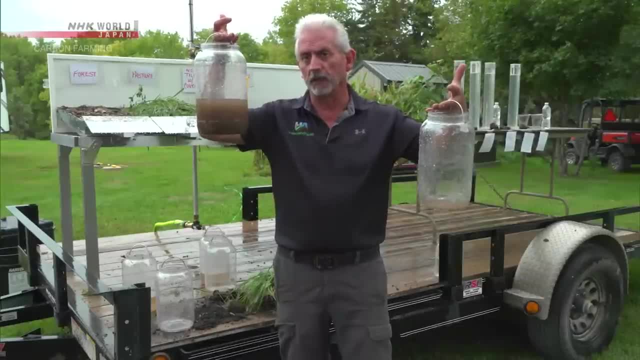 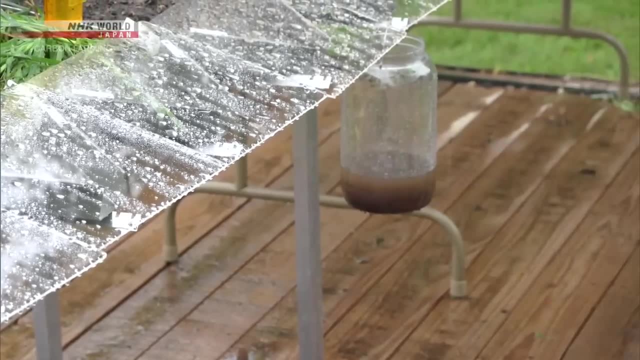 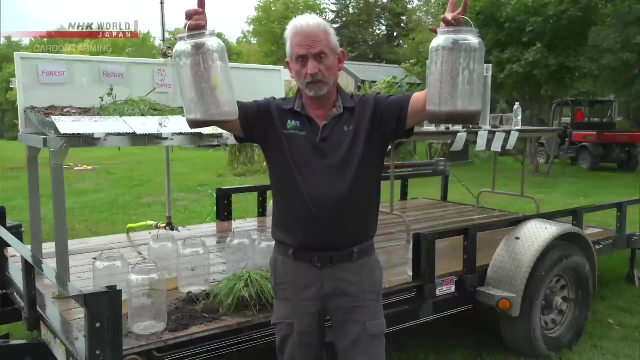 Notice how much water infiltrated in the regenerative farm and look how little ran off. Let's look at the conventional. Look how much water ran off. Look how much infiltrated Between these two. the soil from the Breitkreutzes farm absorbs more water. 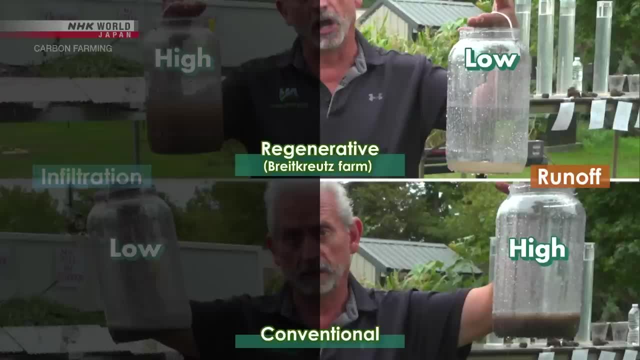 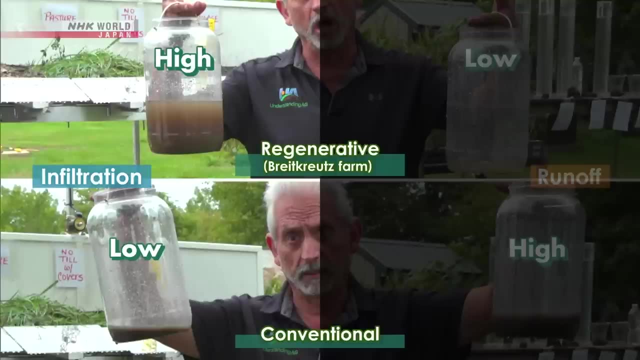 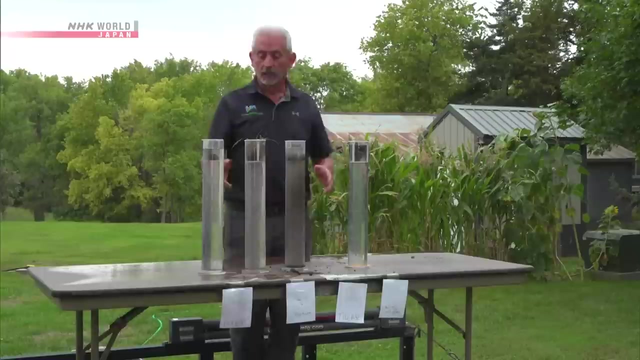 and allows less of it to run off. Its higher rate of infiltration means it can carry water deep into the ground. Soil that absorbs and holds more water is more resilient against flooding and droughts. Let's see what happens here. You will see that the forest system 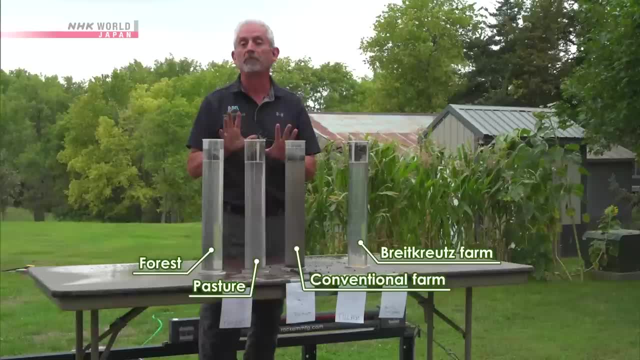 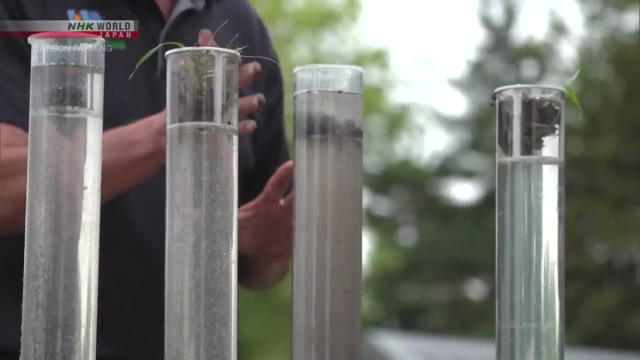 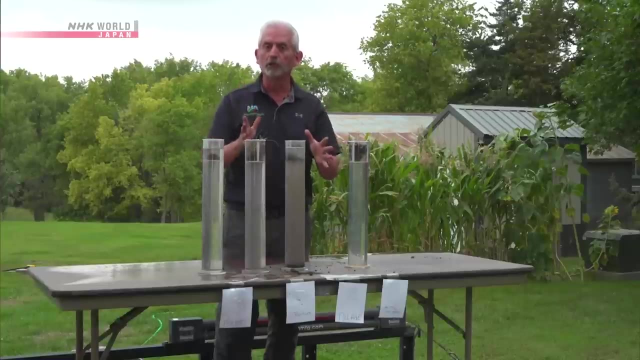 it's holding its integrity. It's clear. Water's rushing in to fill the pore space. Notice the column. It is clear. but notice the conventional soil: It's beginning to fall apart. Please understand: soil is the life, It's the glues. 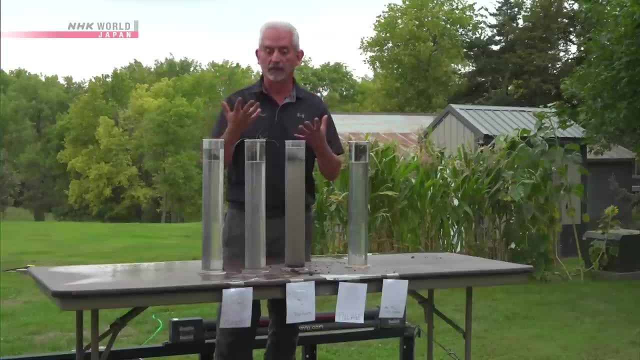 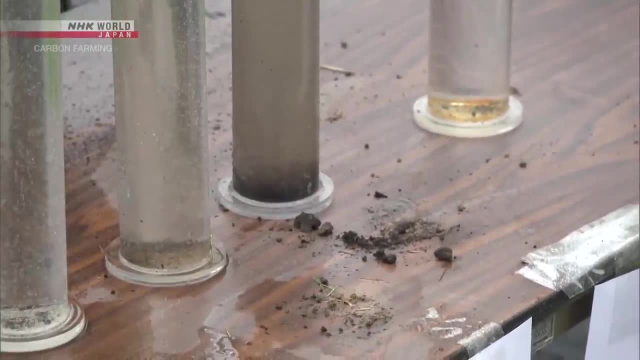 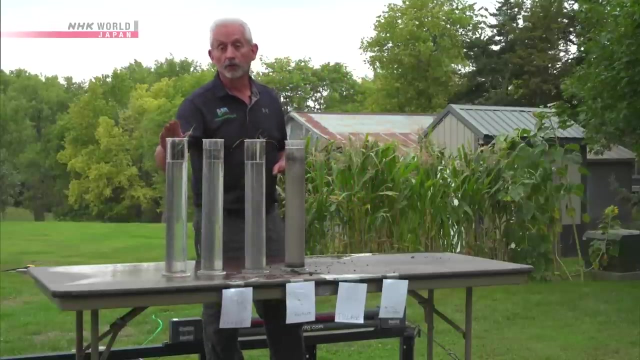 It's the byproducts of organisms and the living plants They create the glues. Notice this ones. The glues have been diminished. Now let me move this over here, So you know what the Breitkreutze is doing. 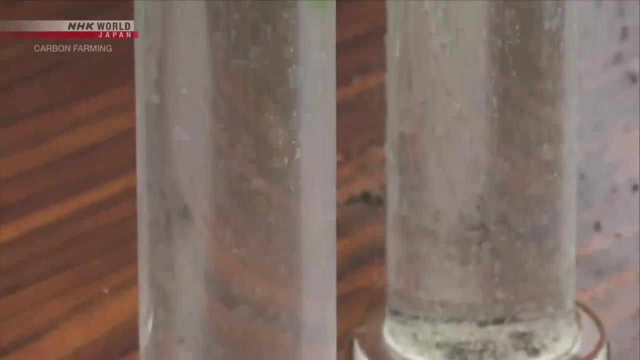 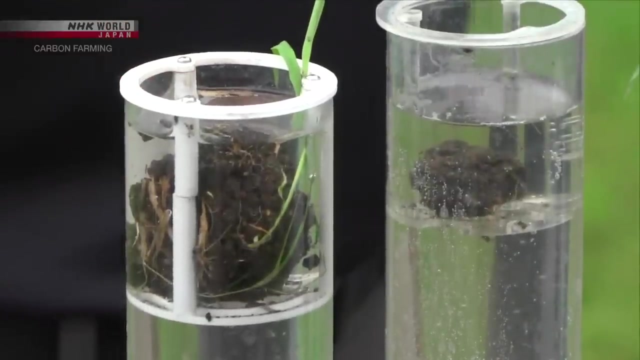 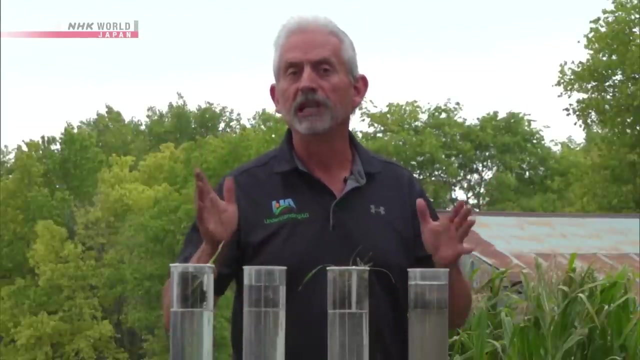 They're farming like the forest Clear. Nothing's falling, apart All those biotic glues, the organic matter, it's still present. Nature does not till Her tillage. equipment is earthworms, living roots, life biology. 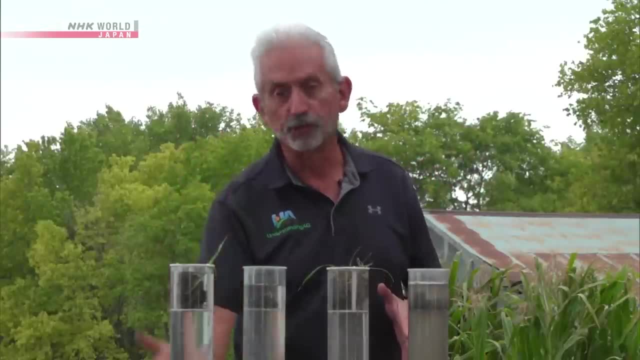 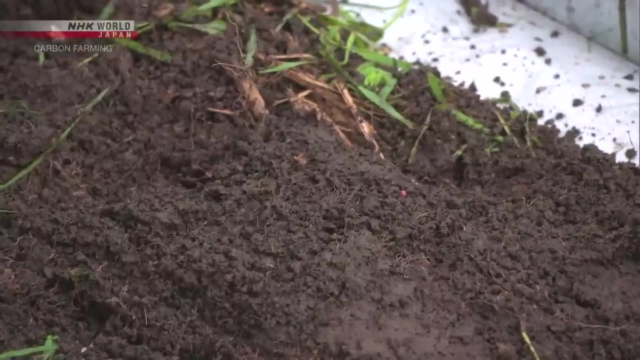 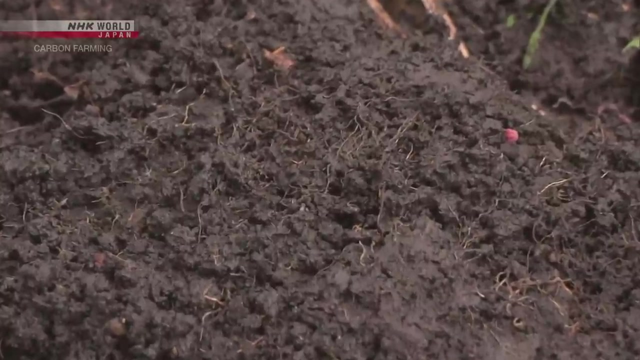 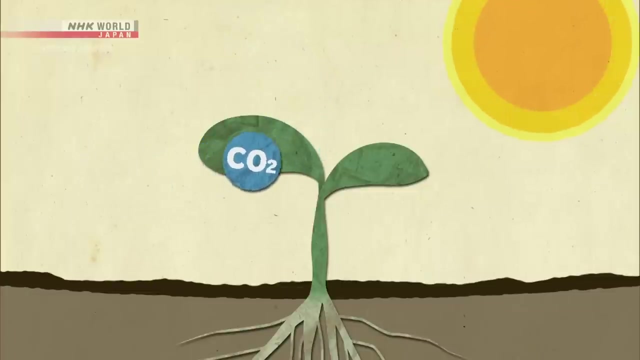 Notice the columns here. This is regenerative agriculture: Farming like nature, Natural soil that's not tilled. What on earth is happening inside this natural environment? Plants absorb CO2 from the air in a process called photosynthesis, And by doing that you can produce CO2.. 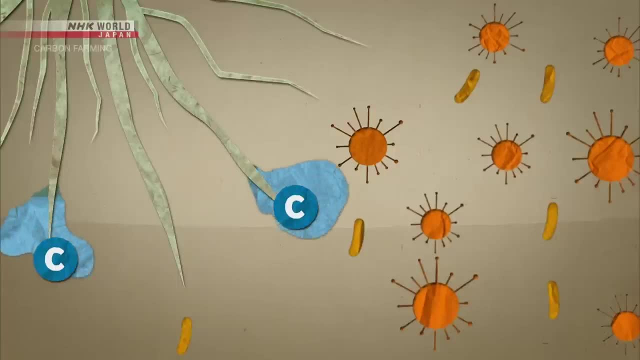 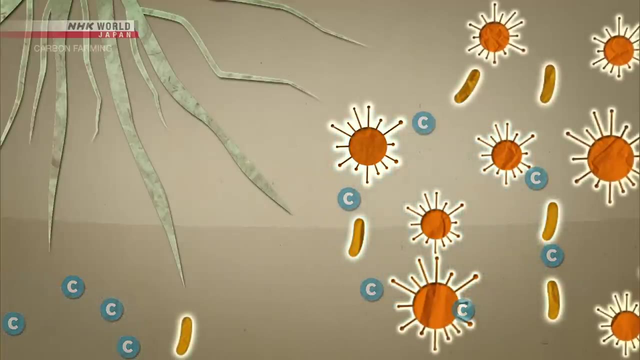 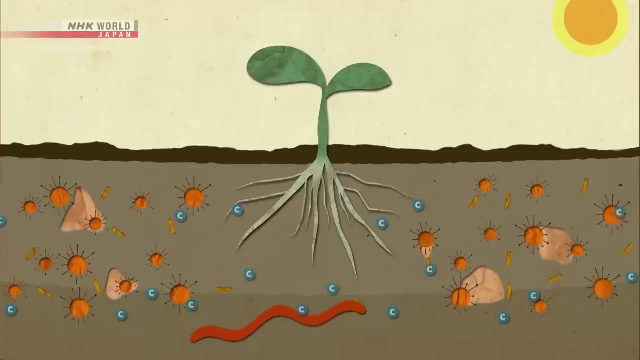 The carbon turns into sugars and other carbon compounds and are secreted through the roots. Some of those compounds serve as food for microorganisms. These microorganisms break down organic substances in the soil, making it easier for the plants to absorb nutrients, Secretions from these microbes, as well as waste matter. 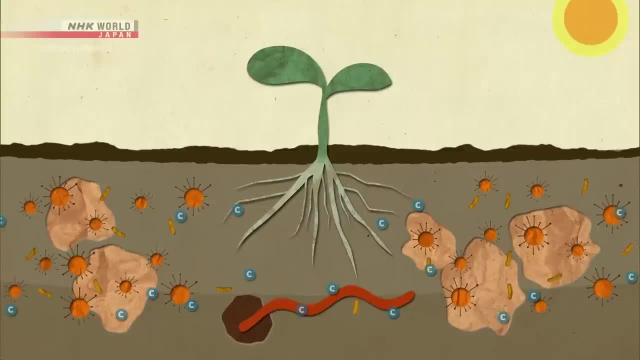 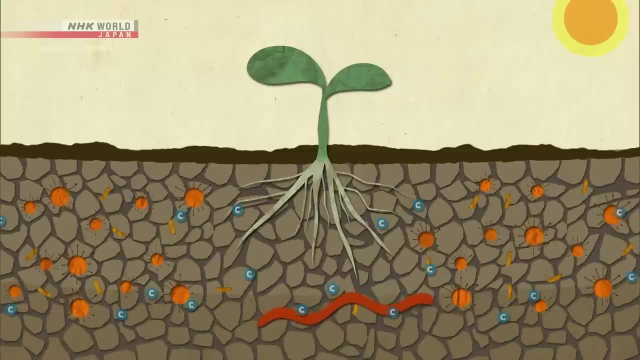 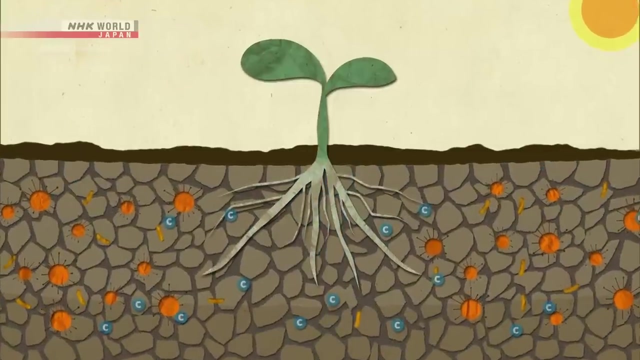 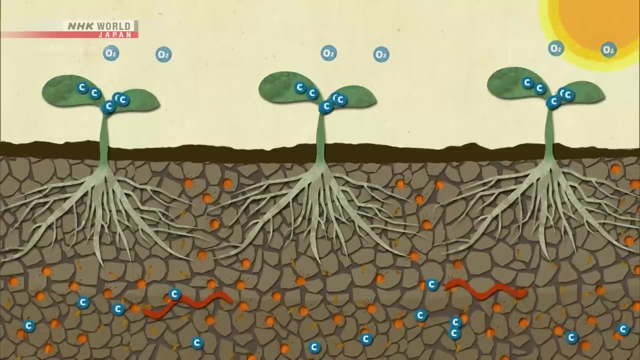 from. little creatures like earthworms work as a glue to keep the soil together or aggregate it. Aggregated soil has spaces that allow for air and water to flow. These spaces also create room for roots to grow. This way, the more the ecosystem in the soil flourishes. 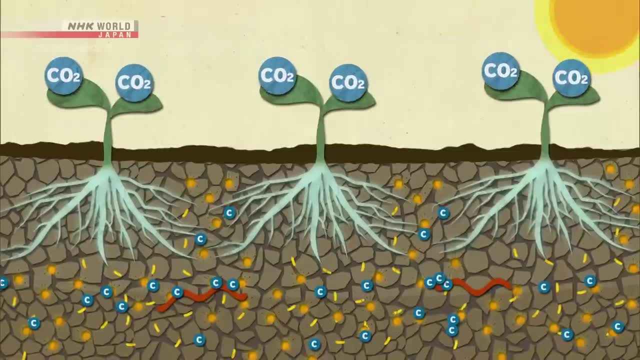 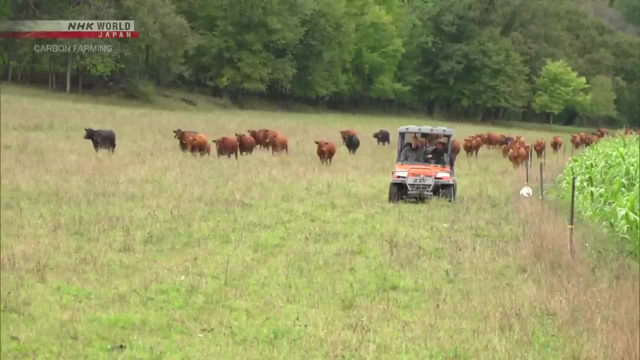 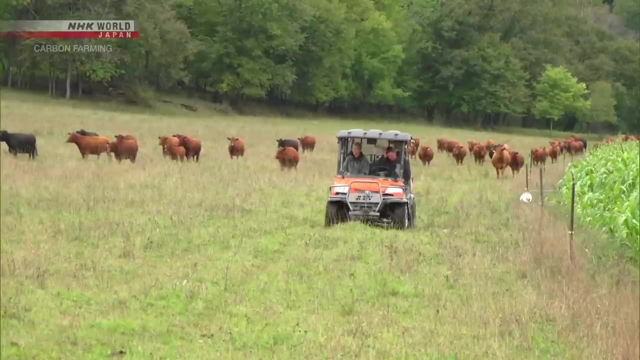 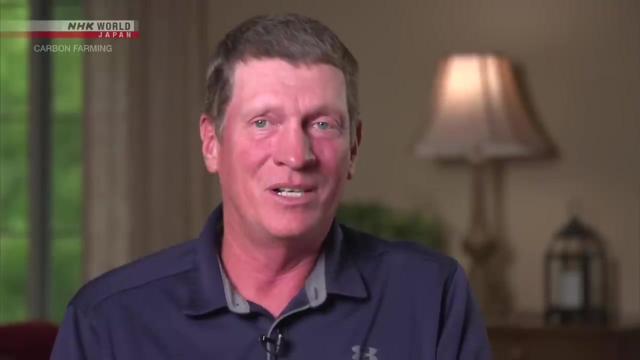 the better the soil's condition and the higher the amount of carbon in the soil. The Breitkreutzes say they've seen a significant change in their field since they started regenerative agriculture. We've regenerated some of our soils and we've seen the benefits of it. 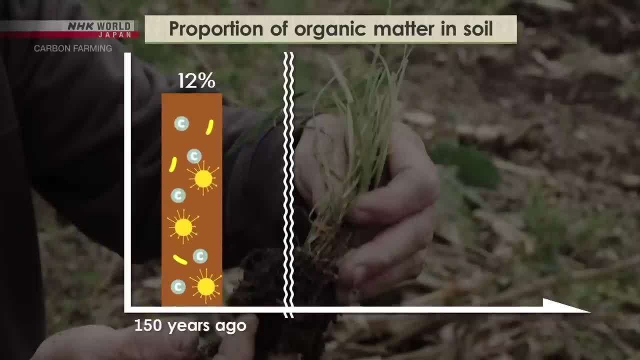 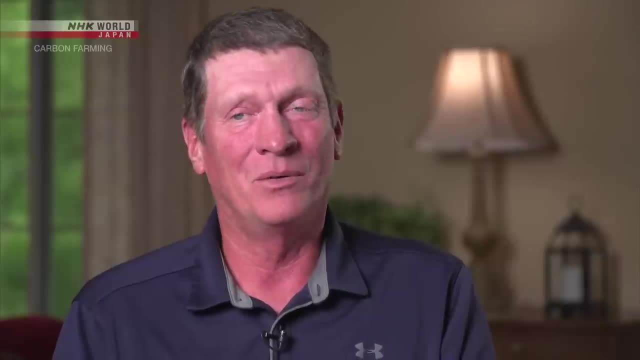 point in time these native prairies are about 12 organic matter. we're down to two and 150 years of farming now. in say 10 to 15 years of focused regeneration on this land. we've got it back up to five and six if we could keep going. the 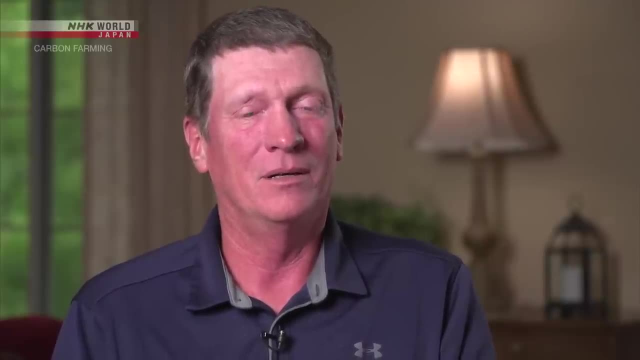 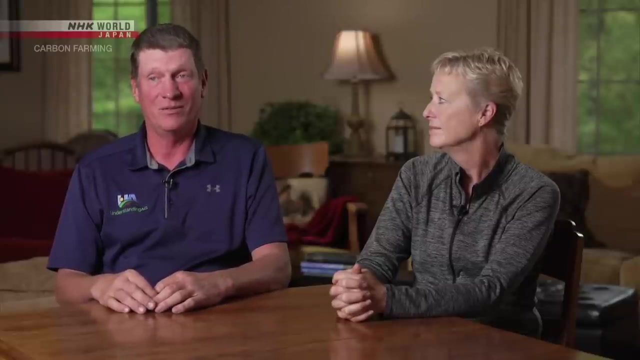 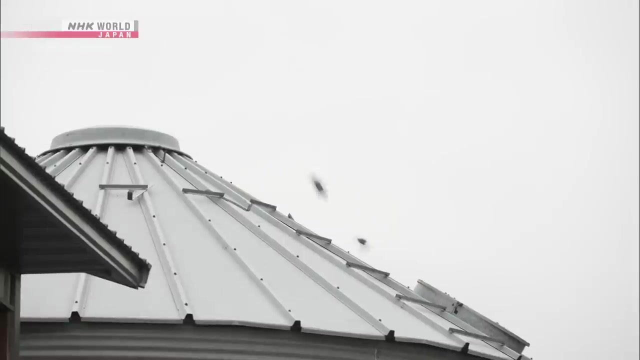 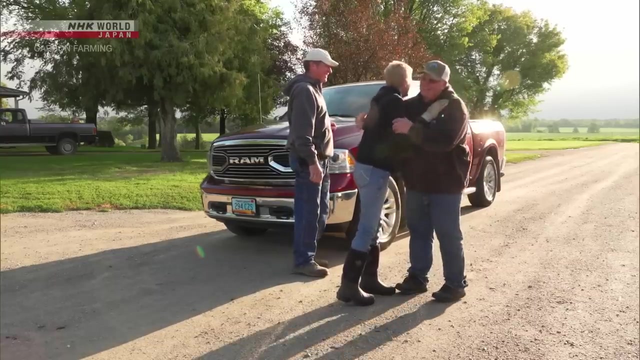 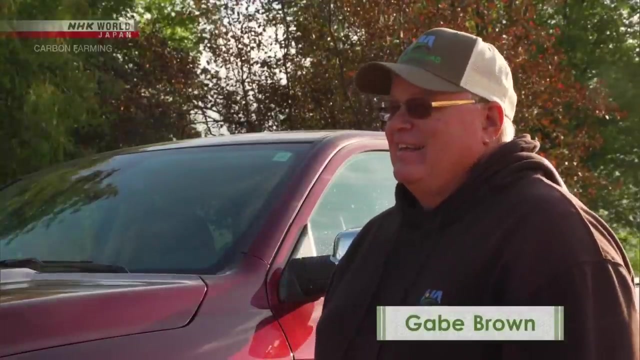 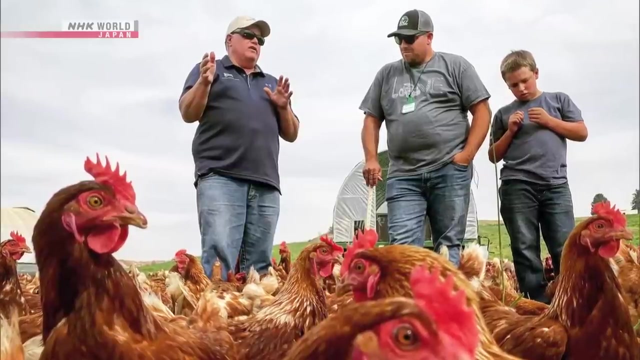 right way and definitely not turn back the other way. it gives me hope that generations on this farm and worldwide can survive and thrive in the future. the couple was inspired to get into carbon farming by Gabe Brown, a pioneer in regenerative agriculture. he himself runs a farm spanning 2,000 hectares in North Dakota to tell people. 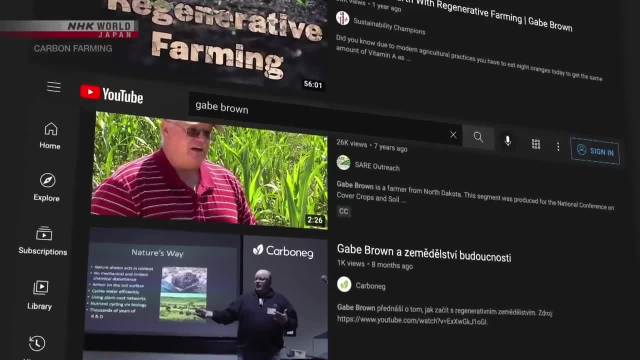 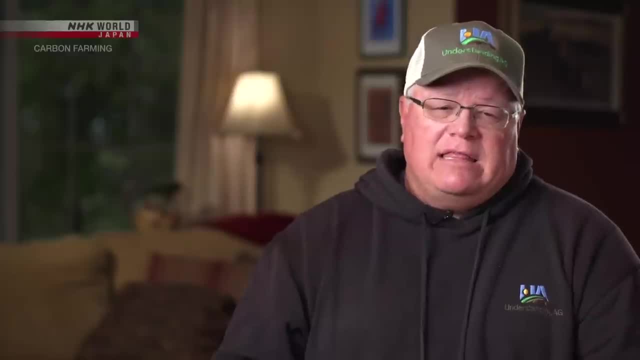 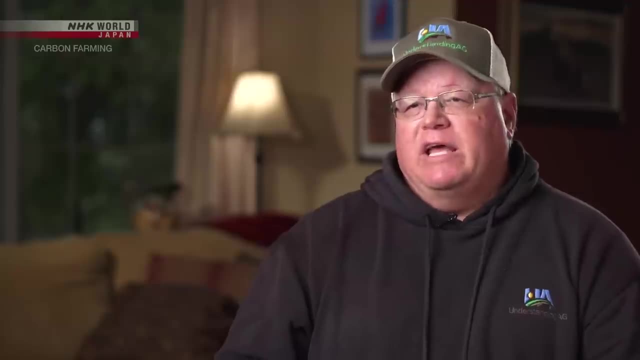 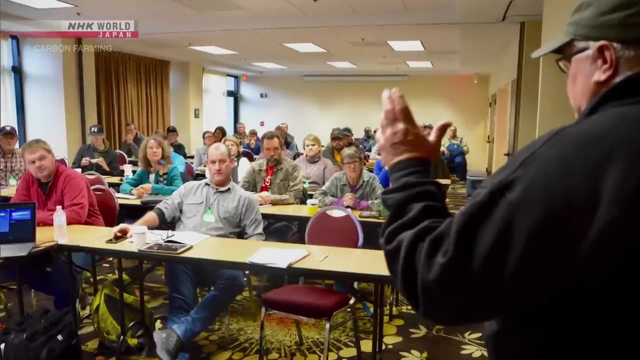 about his unique farming method. he spends much of the year giving talks about his principles. I think that a lot of what we're seeing globally today is a direct result of the mismanagement of our ecosystems, because farmers, ranchers and others are have not used and applied these principles we're now seeing 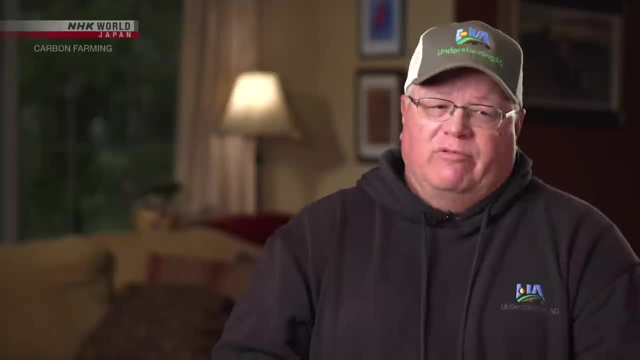 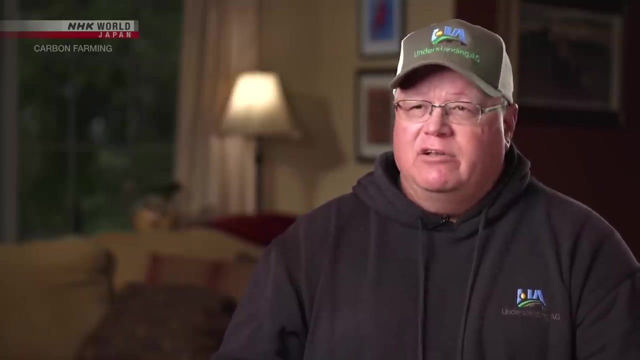 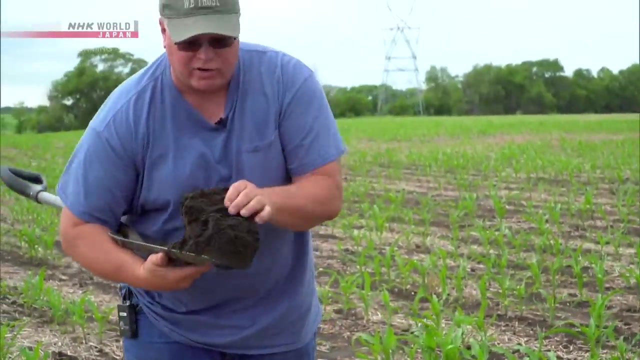 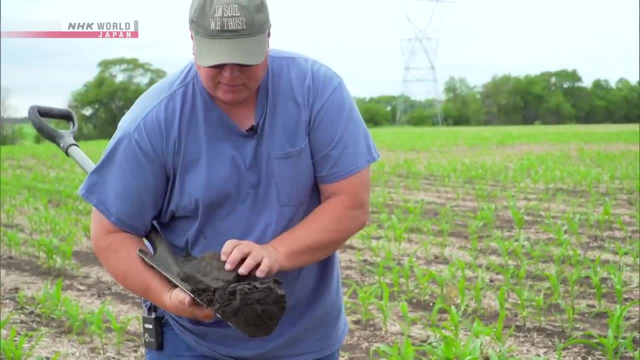 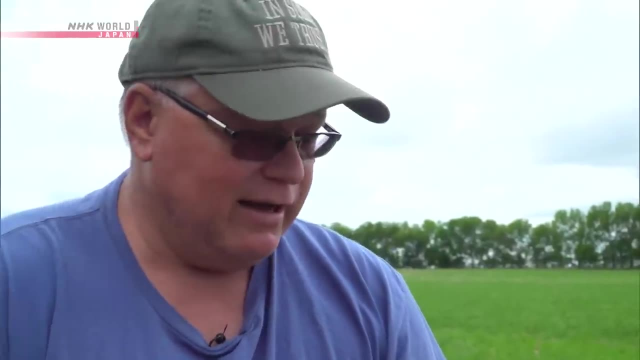 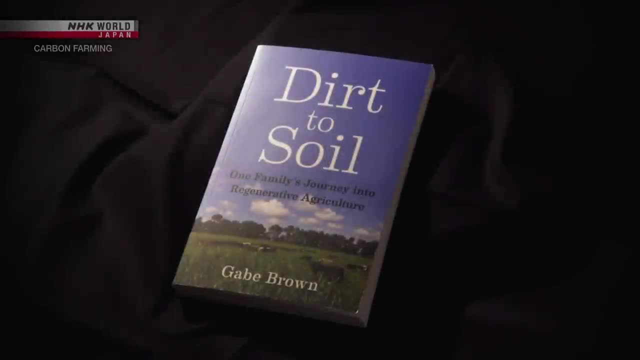 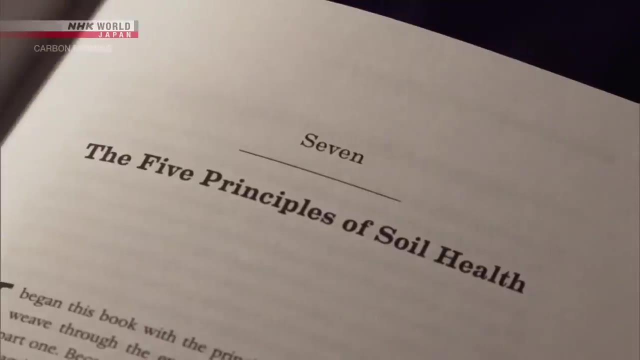 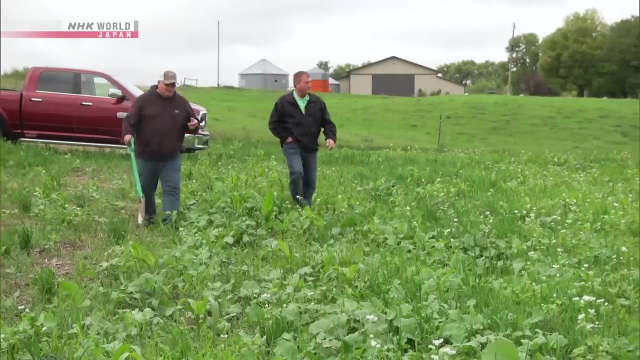 farming. he relates his struggles and success in his book dirt to soil. in it he summarizes the theory and practice of his ground breaking farming method into five principles. let's walk out here. let help the real gardener To learn the know-how. more than 2,000 people a year have visited Brown's farm. 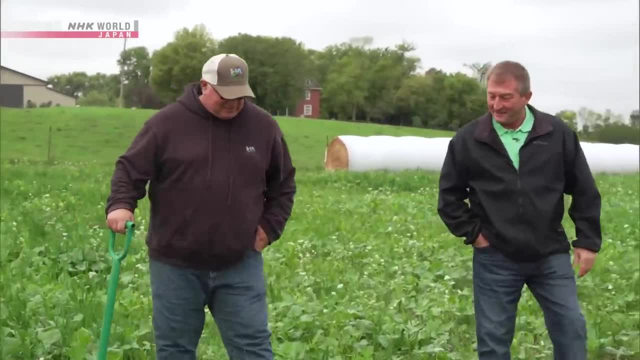 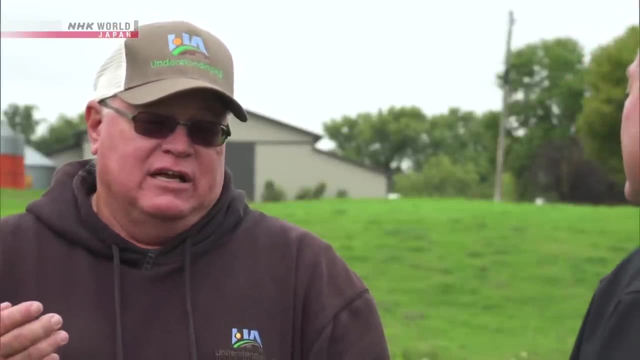 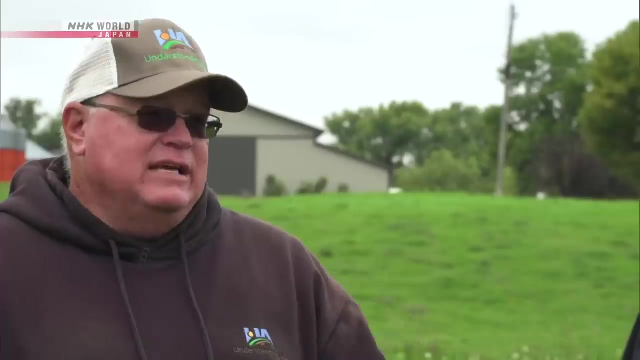 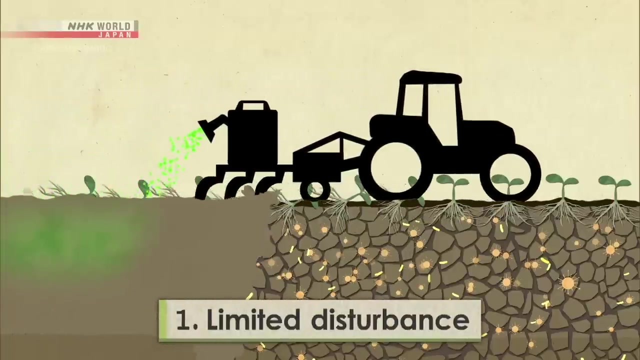 A lot of different plants. that's right. I always tell people when they're interested in regenerative agriculture is you have to understand the processes and the principles. So the first principle is the least amount of mechanical chemical disturbance possible. Principle one is to limit the disturbance of soil. 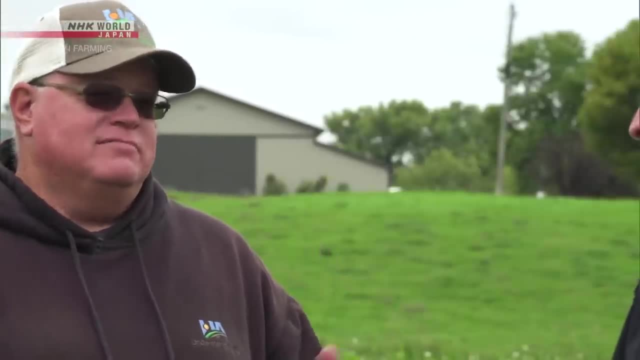 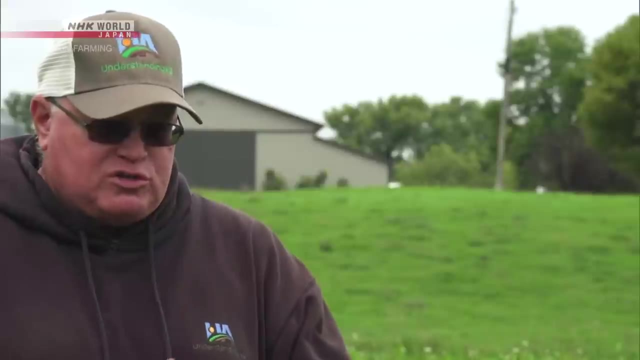 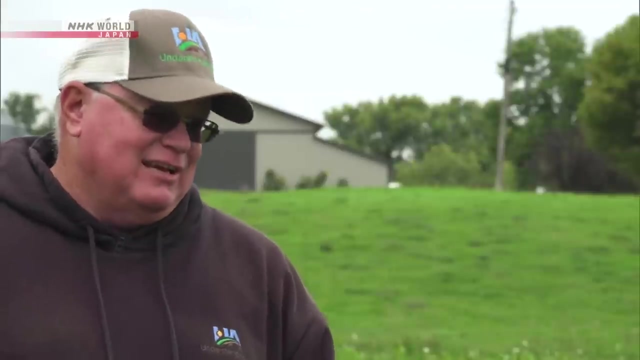 OK, where in nature do you find tillage? You don't People rototill their garden. What happens when you do that? You destroy the natural home for all that biology, the same biology that's going to cycle the nutrients to help those plants grow. 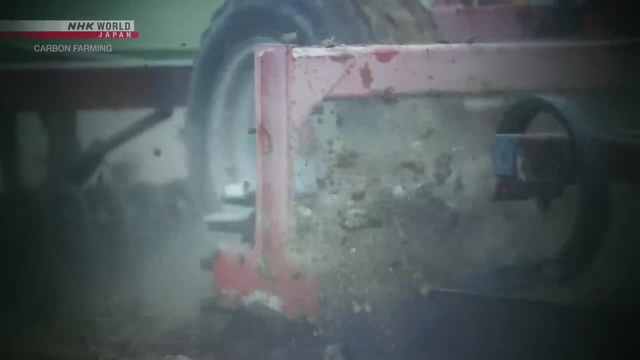 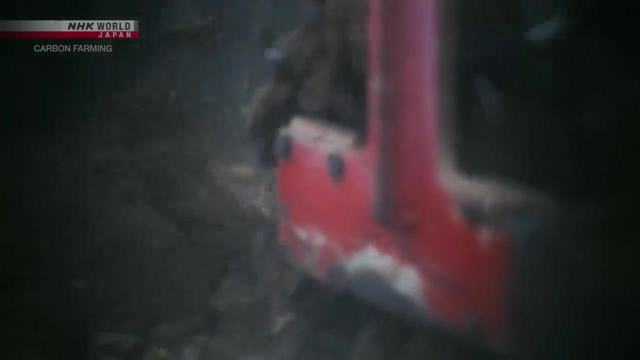 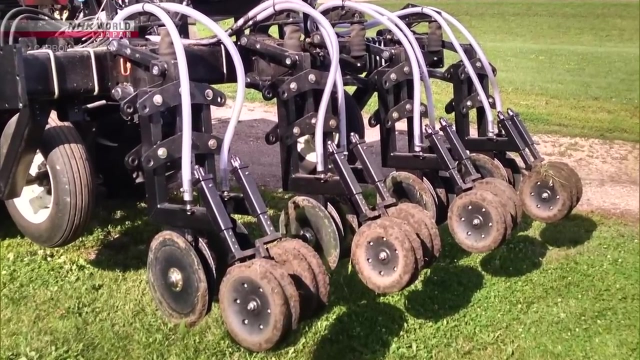 Tilling breaks down the soil structure that has been created by the soil, Created by living things. It destroys the home of the diverse organisms and creatures that are necessary for the growth of plants. No-till farming uses special equipment that cut narrow grooves in the surface. 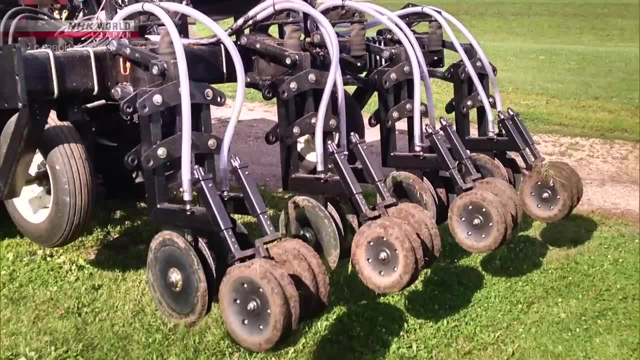 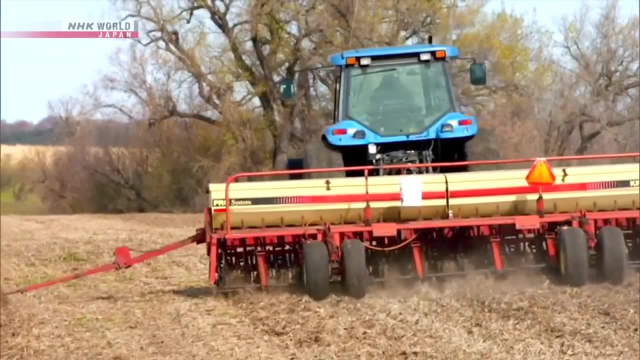 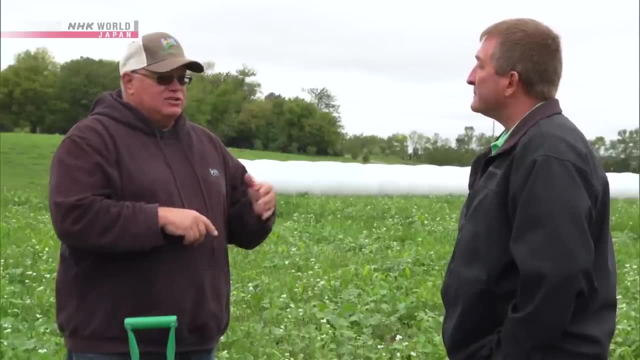 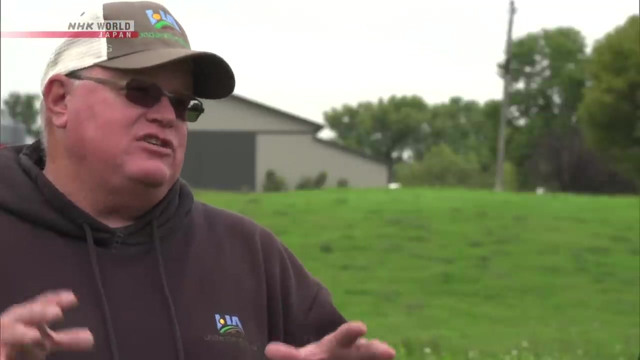 just deep enough to plant seeds. By not plowing the soil, the underground ecosystem remains intact. It's not only tillage, It's also chemical disturbance. So synthetic fertilizer is a chemical: Herbicides, pesticides, fungicides. That's fighting nature when we do that. 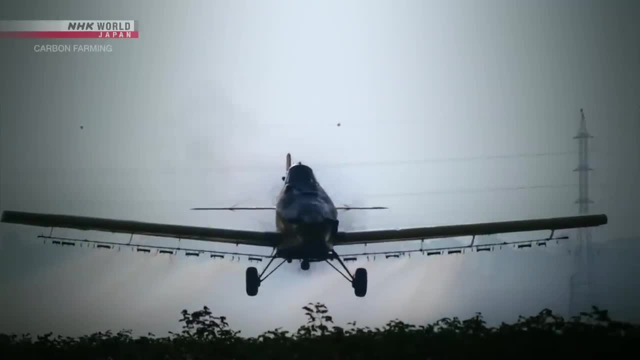 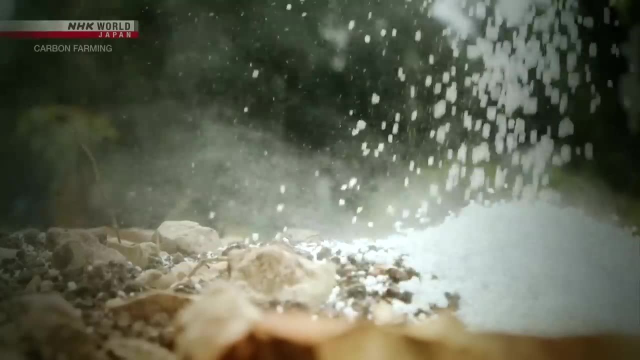 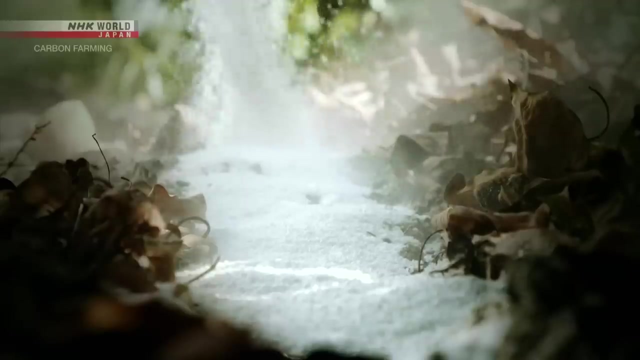 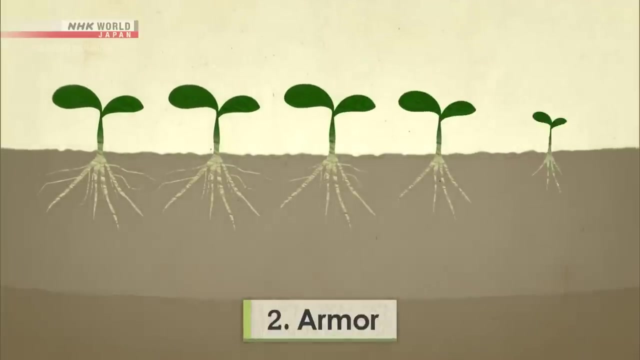 Agricultural chemicals kill not just harmful insects and germs, but also microorganisms that are beneficial to plants, And it's best to minimize the use of chemical fertilizers, as they disturb the symbiotic relationship between plants and microorganisms. Brown's second principle is to keep the soil covered with natural armor. 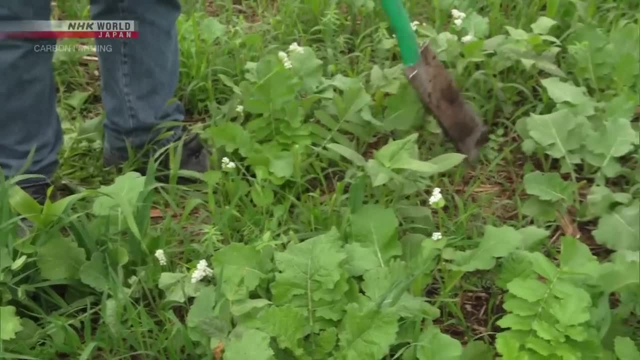 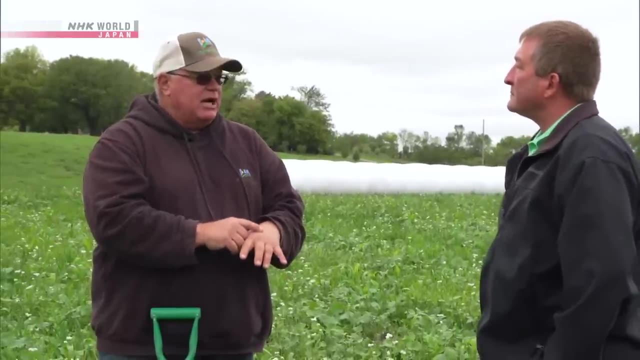 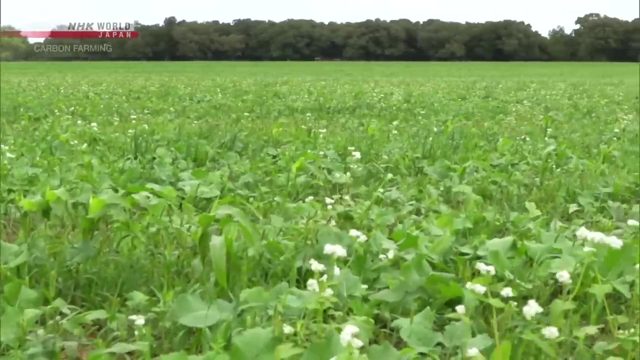 And look here where we're standing. Look at the armor, that residue that's covering the soil. That protects the soil just like our skin protects our body. Soil should not be exposed, but covered with plants at all times. This protects it from erosion by wind and water. 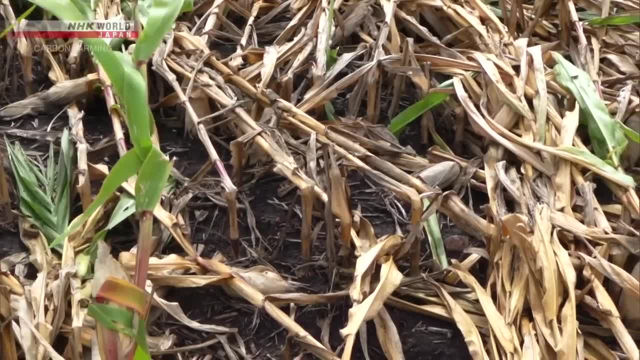 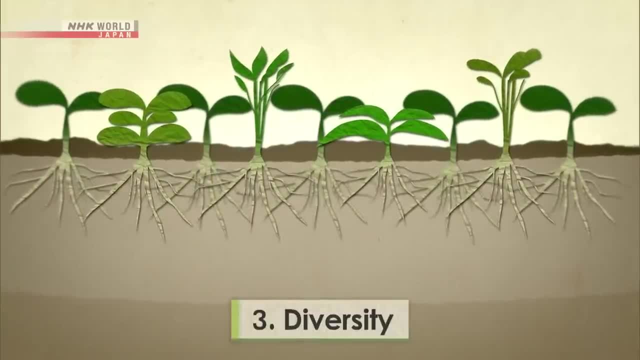 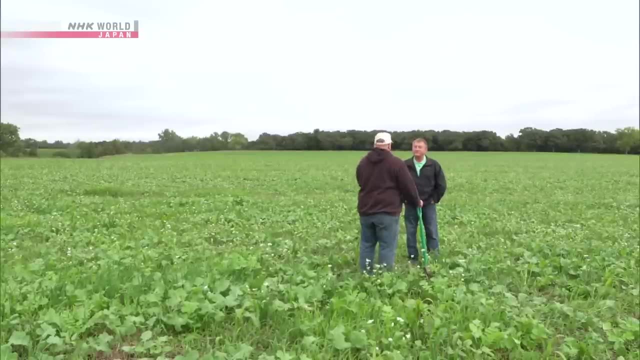 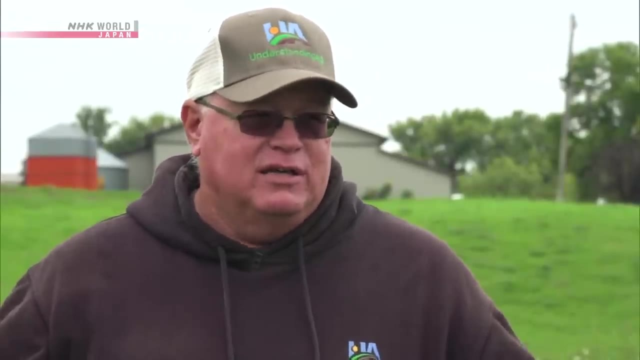 and also prevents moisture evaporation. Principle three is diversity. So look here in this cover crop I actually have about 12 different species of plants growing here together. Nature abhors a monoculture, does not want a monoculture. Brown says diversity enhances ecosystem function. 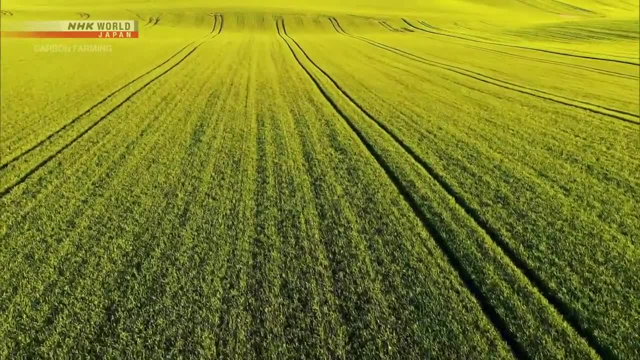 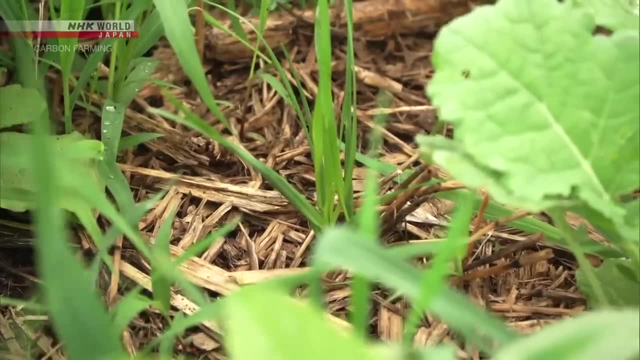 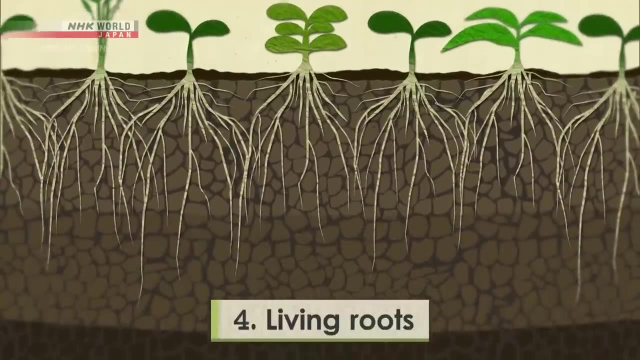 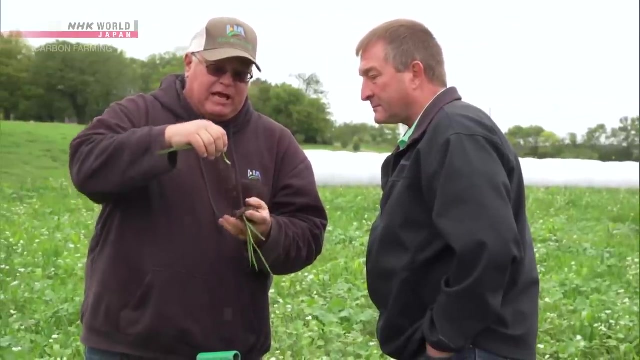 A single species is not enough to ensure a well-balanced soil. Each plant or living organism plays a role in maintaining soil structure and in creating a resilient, healthy soil. Principle four is to maintain living roots. If we look at this like here's a young growing plant. 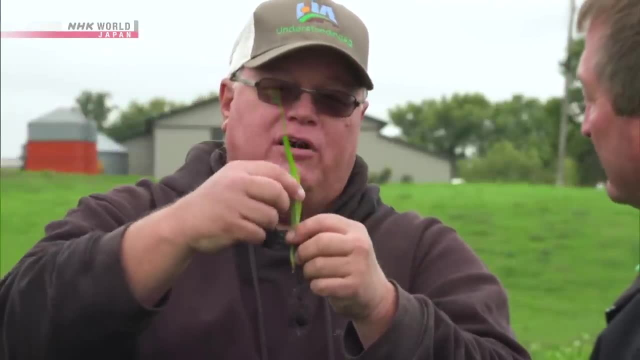 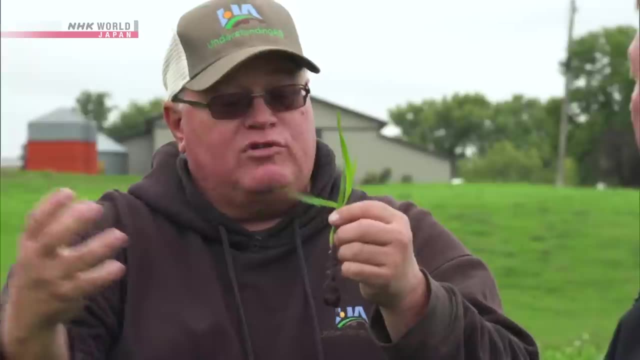 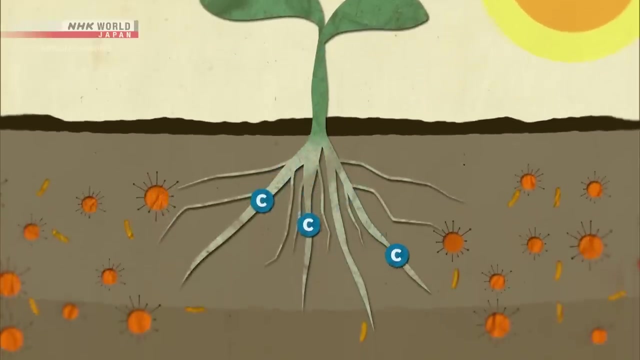 this plant is taking in sunlight. it's using part of that carbon compounds for growth. the rest of it's moving down to the roots and exuding out to attract biology, so that biology running its life cycle can feed it nutrients, If living roots are maintained in the soil all year round. 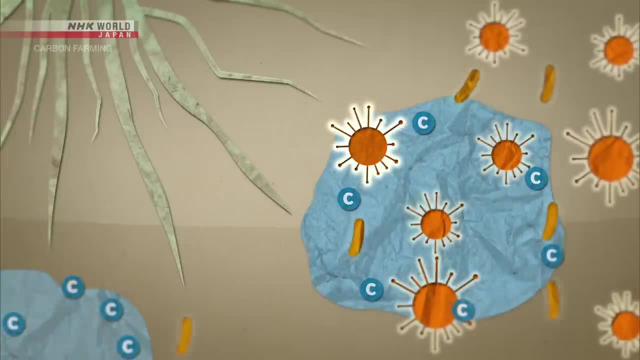 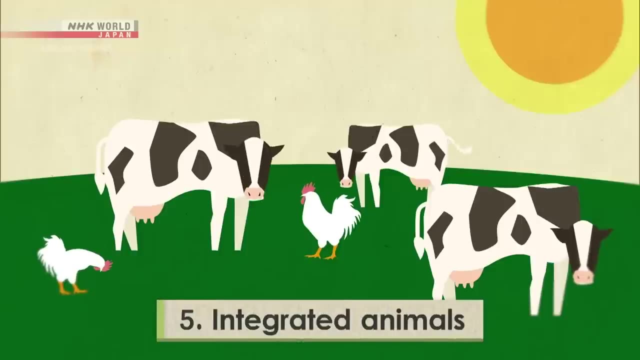 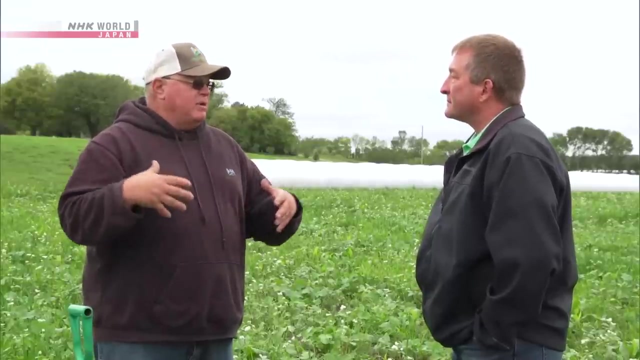 they continue to supply carbon compounds that serve as food for microorganisms. This preserves the health of the soil. Principle five is to integrate animals into farming. Livestock have a lot of biology in their guts, just like we do as humans. That biology then as they're grazing. 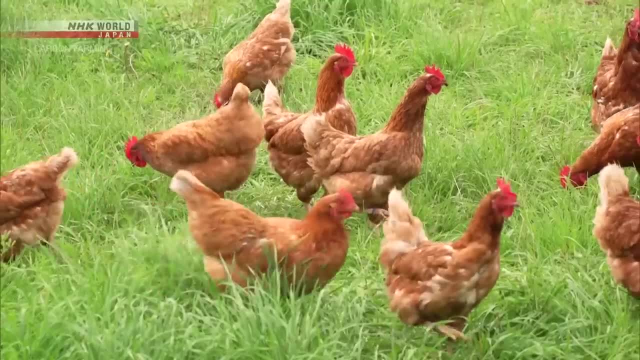 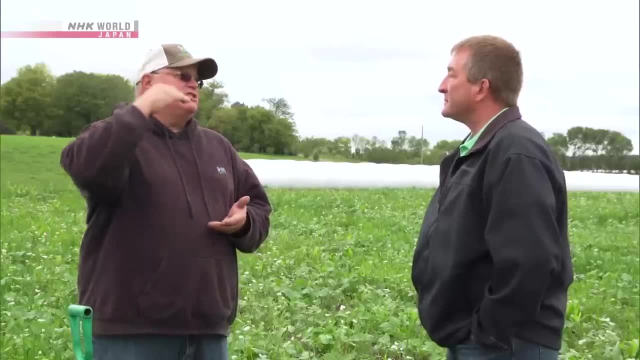 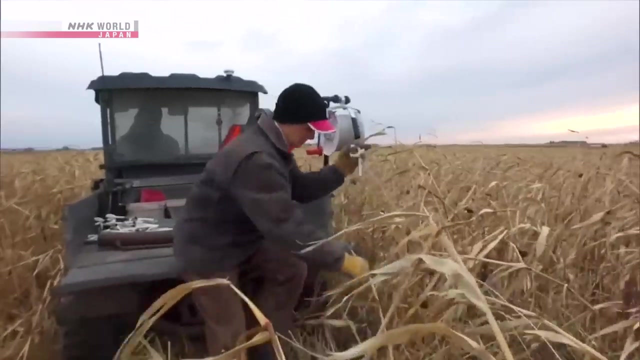 some of that biology will be expelled through grazing, through their manure, through their urine. that fertilizes the soil, And it'll just take your soil health to another level. As a way to achieve that, Brown uses a form of intensive grazing. 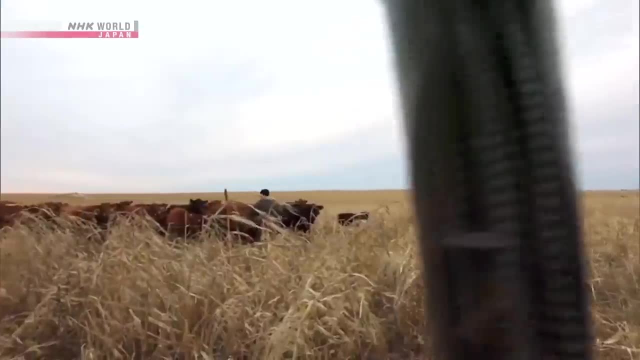 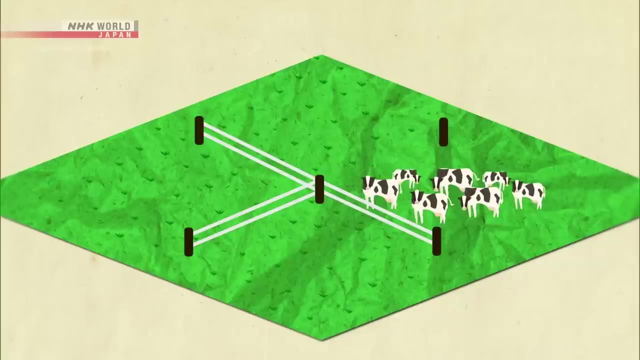 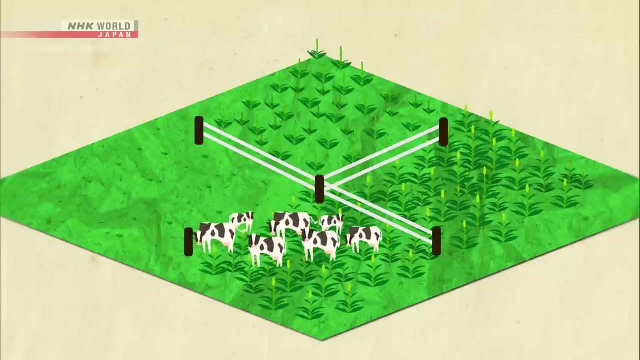 He divides his pasture into sections and packs one of them with cattle To prevent overgrazing and damage to the soil. he moves the cattle frequently, creating a more adequate grazing cycle that stimulates the plants to grow and sends more carbon into the soil. 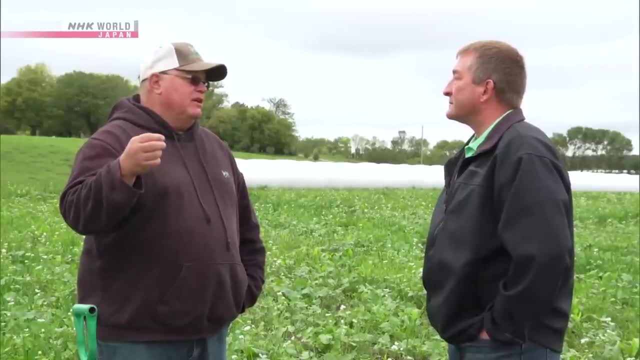 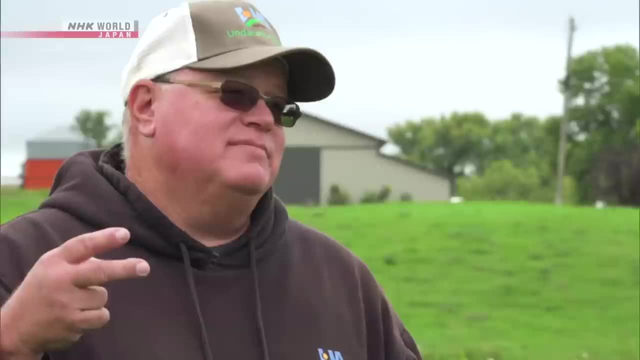 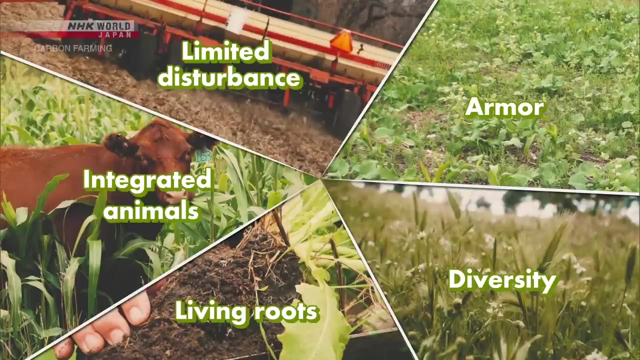 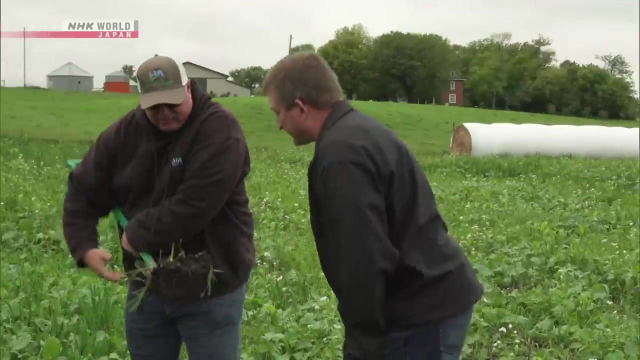 We can increase profitability and improve advanced soil health in as quickly as two years. Two years is all. All five principles center on the goal of restoring the natural ecosystem of farmland. The key is in the relationship between soil roots and microorganisms. 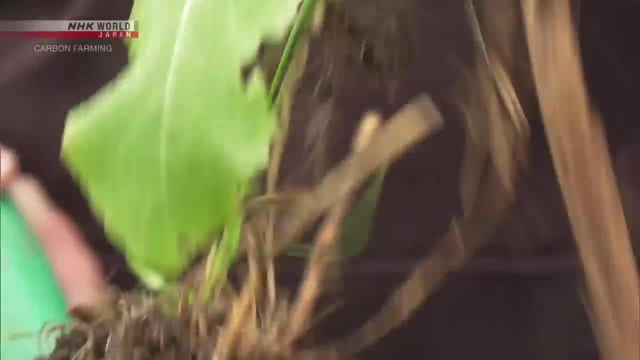 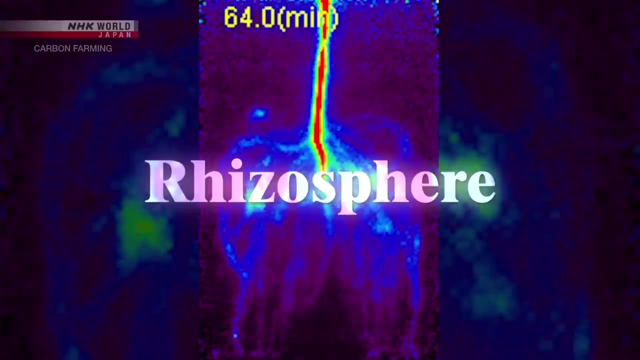 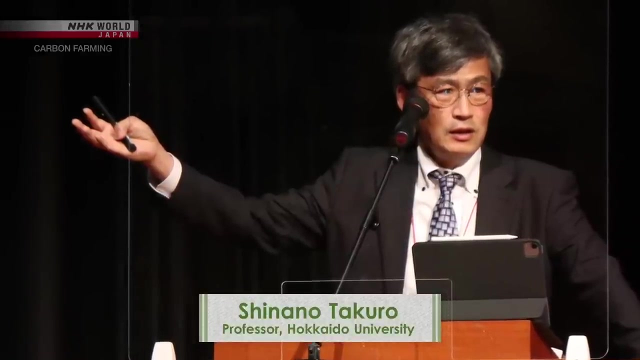 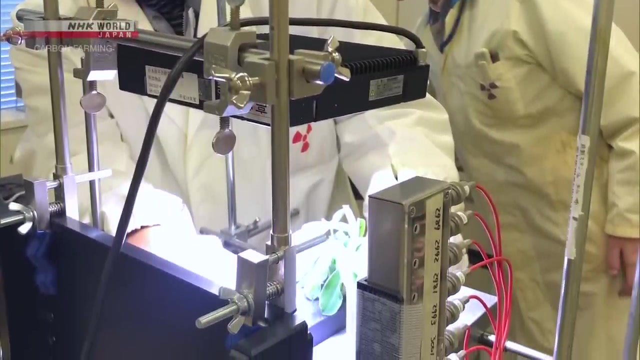 They interact with each other in a micro-world called rhizosphere, or rooting zone. Researchers are uncovering its secrets. Shinano Takuro is an agronomist specialized in soil. His team has succeeded in capturing the world's first visual images of what's happening in the rhizosphere. 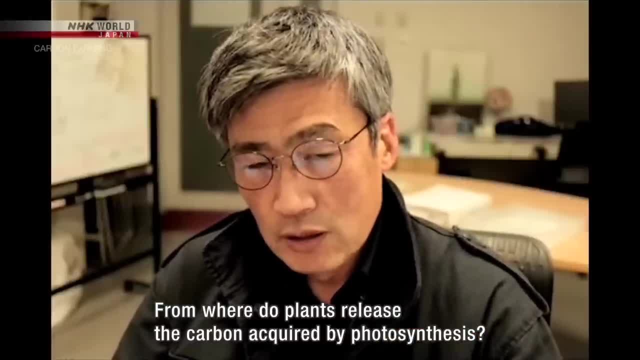 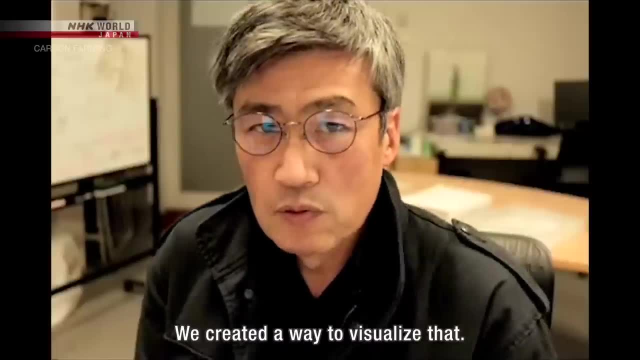 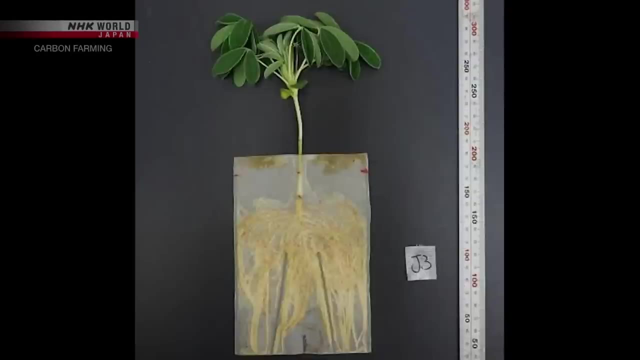 We've discovered where carbon is obtained from and how it interacts with microorganisms. That's what we've developed. The team conducted an experiment with a plant of the leguminosae family. They sandwiched its roots with soil and took images using a special camera. 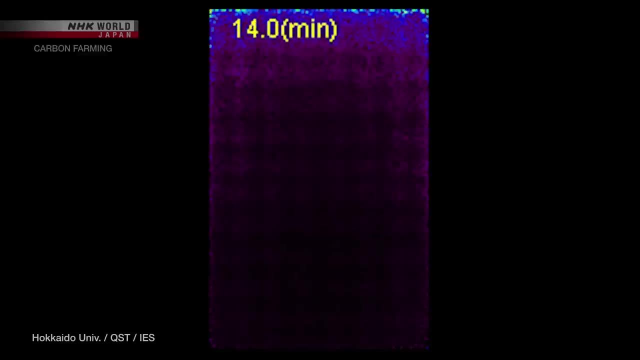 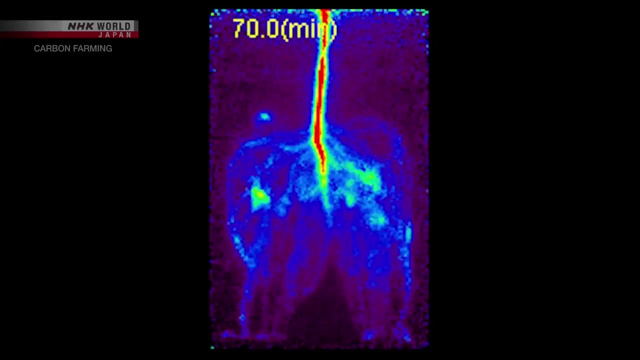 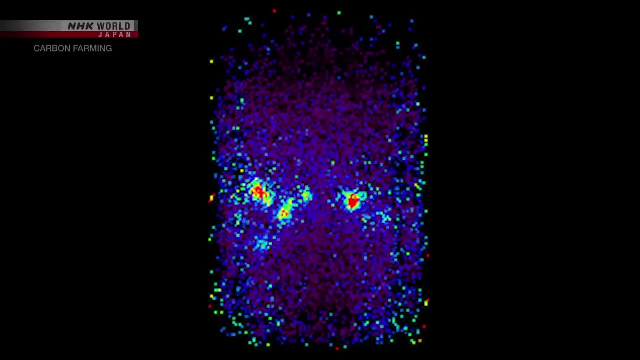 They show that carbon compounds generated by photosynthesis are gradually carried down to the roots. The red portions indicate larger amounts of carbon. When the roots are removed, the carbon secretions in the soil are clearly visible. This shows how the plant actively releases carbon into the soil. 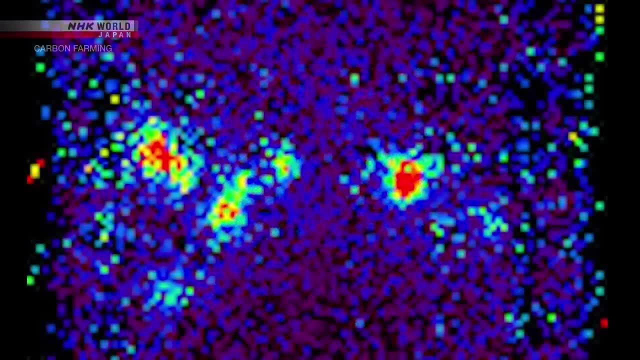 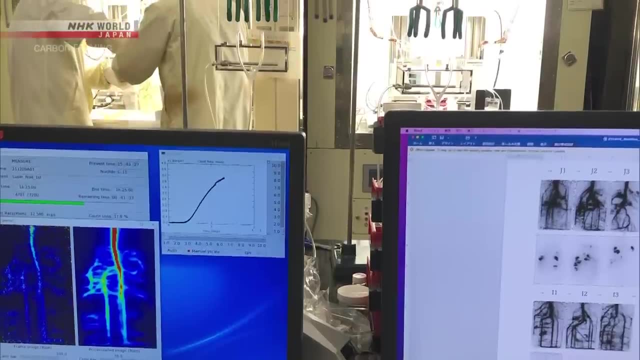 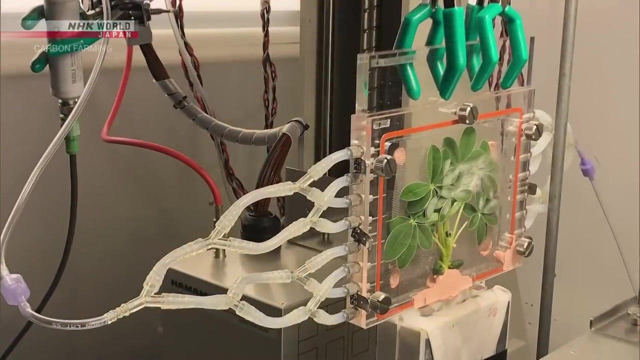 to directly interact with the soil and also sustain its symbiotic interaction with microorganisms. Shinano wants to expand his research so he can help enable sustainable agriculture that doesn't rely too much on chemical fertilizers In the first place in terms of the world. 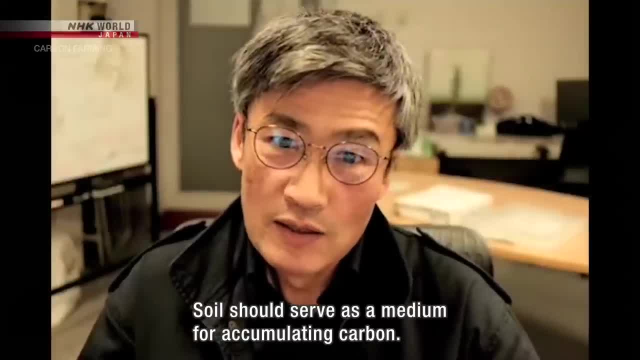 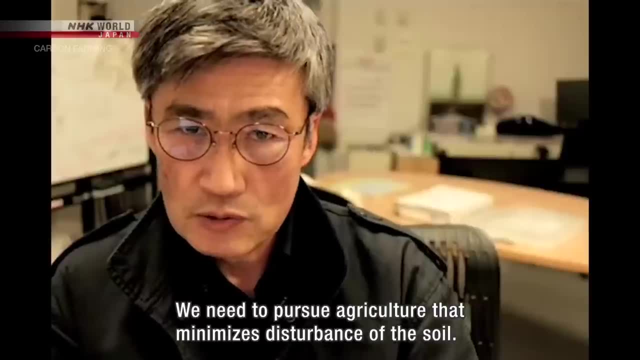 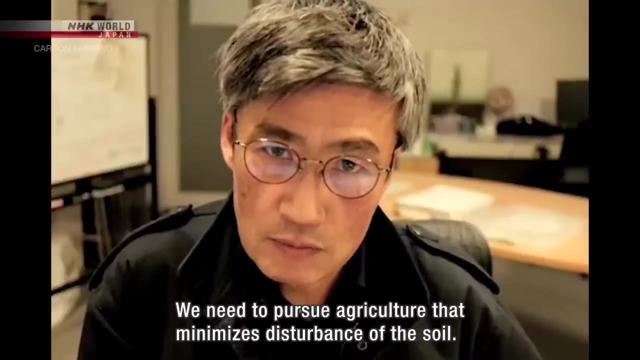 soil is supposed to be a medium that accumulates carbon, But by doing agriculture, its capacity is gradually decreasing. This is something that should be taken into account. I think that agriculture should try not to put too much pressure on soil. The rhizosphere is the stage for the interactions. 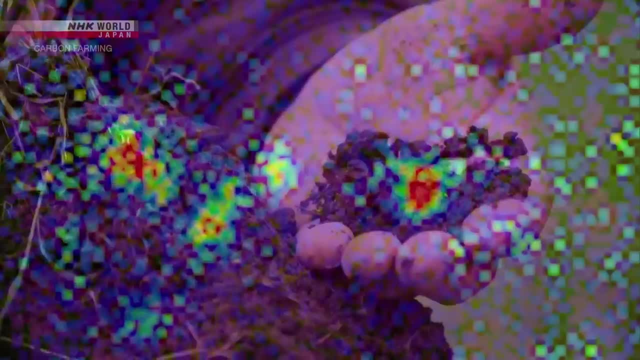 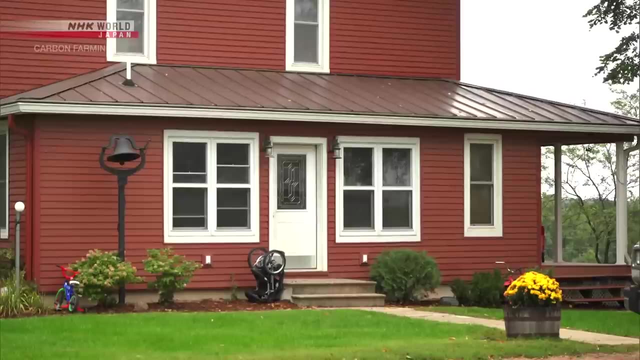 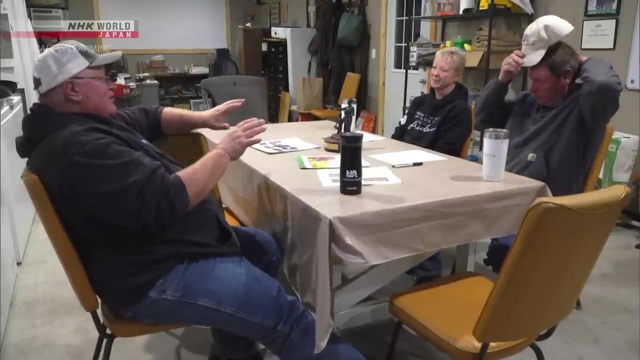 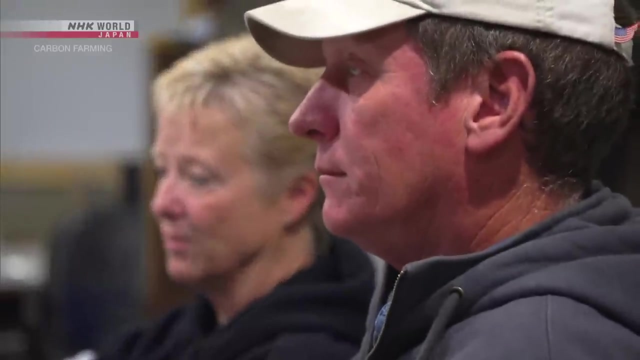 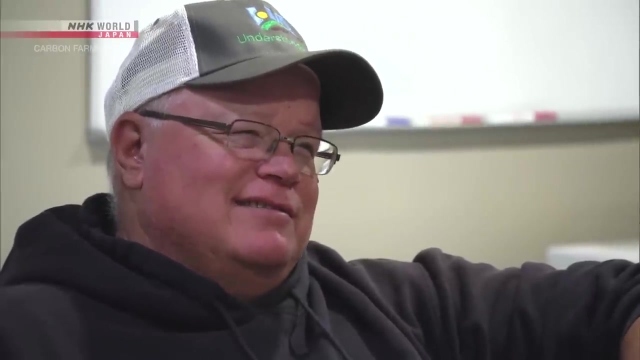 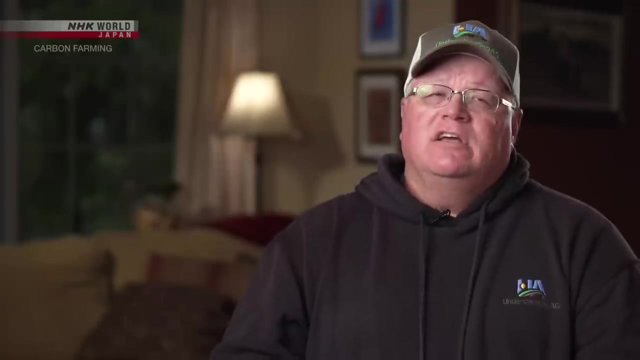 between soil roots and microorganisms. Carbon farming fully utilizes the workings of the ecosystem. Brown and the Breitkreuzes have set up organizations to promote and teach carbon farming. Meanwhile, Brown's five principles are also evolving. The sixth principle we added recently was context. 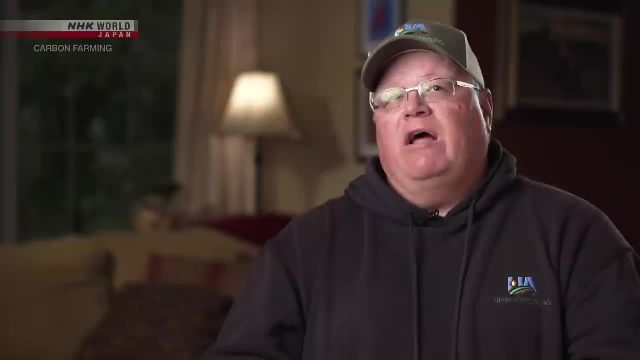 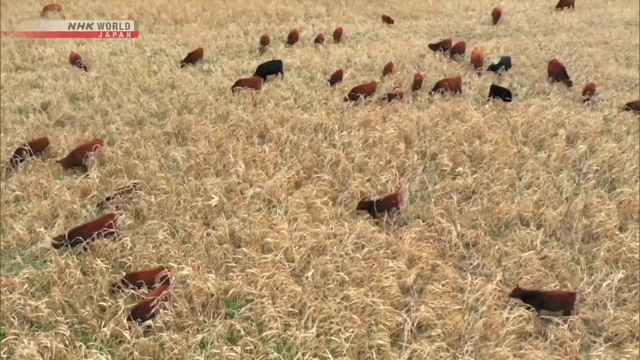 because, as we travel extensively around the world, we see farmers and ranchers not working within the context of their environment. We need to work with nature, not against it. There are six time-tested ecological principles that occur anywhere in the world where there's production on land. 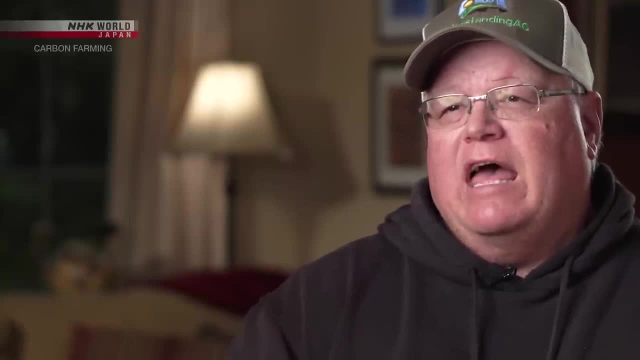 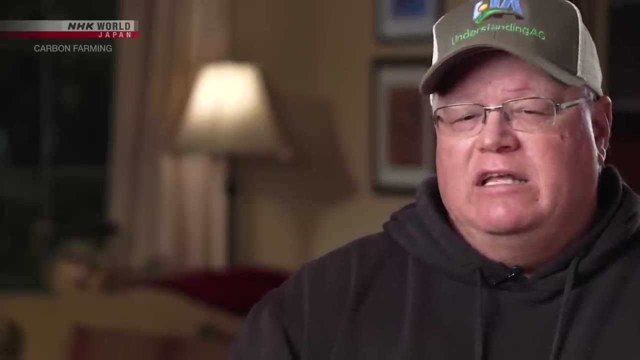 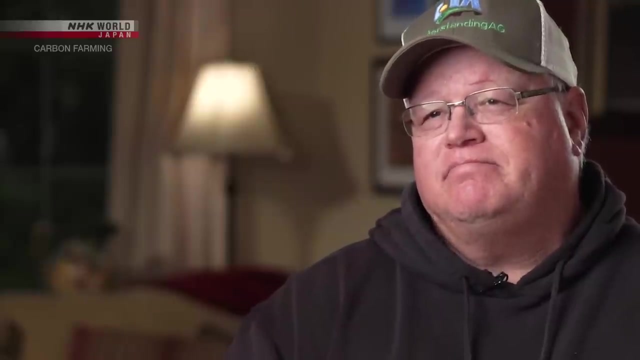 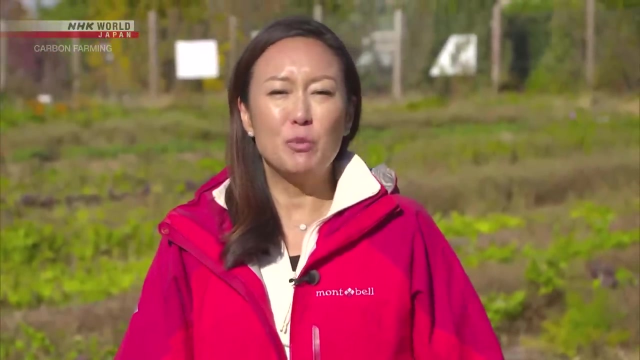 I think this is the only way that agriculture will survive in a way that is truly sustainable And leaves the opportunity for future generations to continue to farm and ranch. Carbon farming is gaining momentum worldwide. The international community is looking to the power of carbon farming. 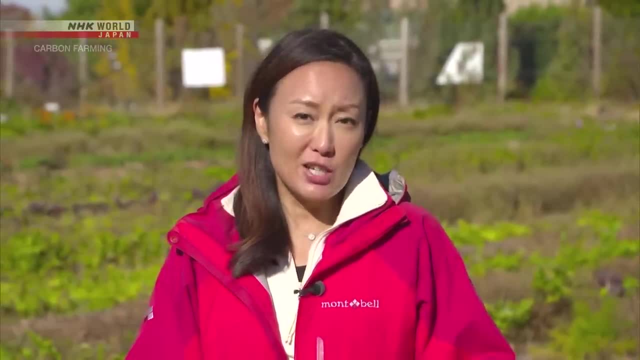 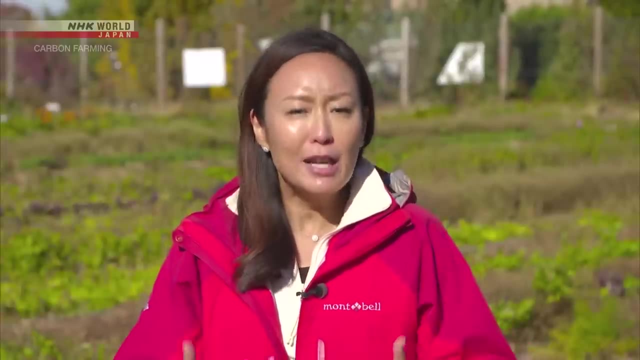 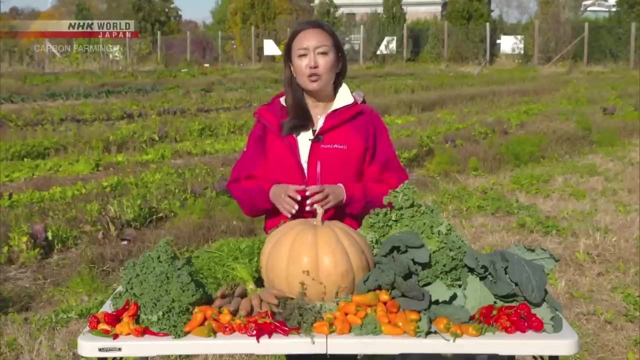 to offset our CO2 emissions. The latest report by the UN Intergovernmental Panel on Climate Change notes that regenerative agriculture is a viable option to address the crisis. Farms, big and small, have started to take action. In southern Japan, one entrepreneurial farmer 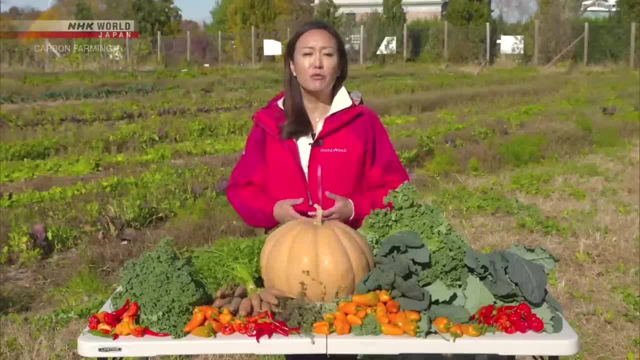 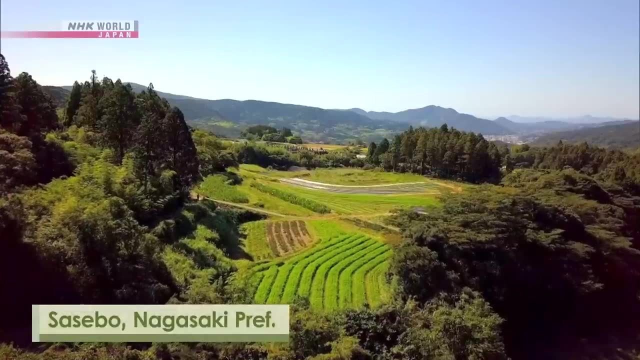 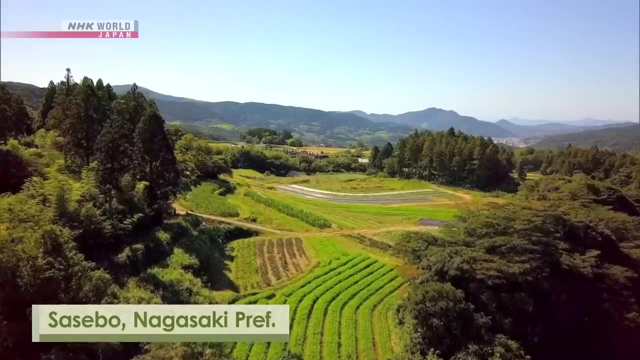 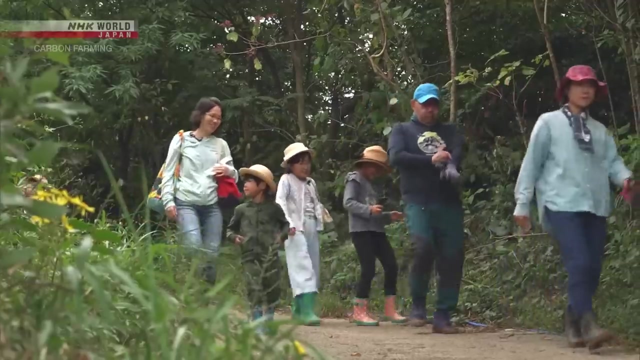 is practicing an effective and low-cost carbon farming method that is also gaining popularity among home gardeners. It all started on this modest two-hectare field. On this day, people gathered to learn about a simple regenerative farming method. anyone can practice. 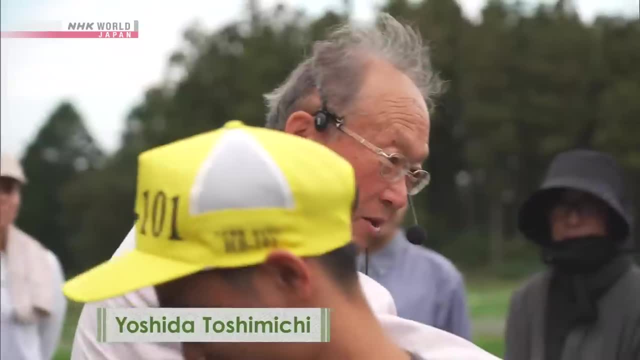 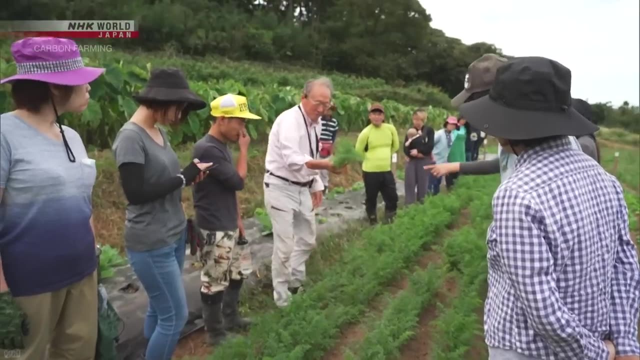 Their teacher, Yoshida Toshimichi, promotes organic agriculture that uses the power of microorganisms in the soil. This is the first time I've seen this. Look at the soil, It's so cute. Why isn't there any soil on it? 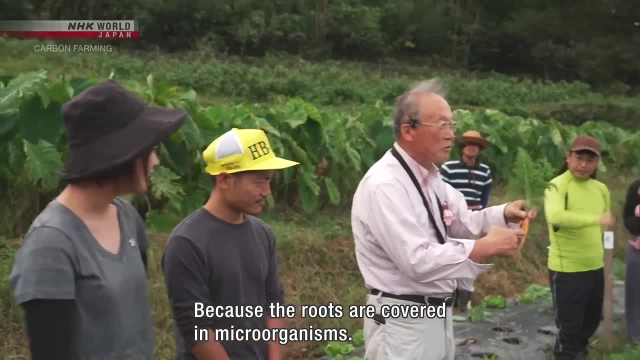 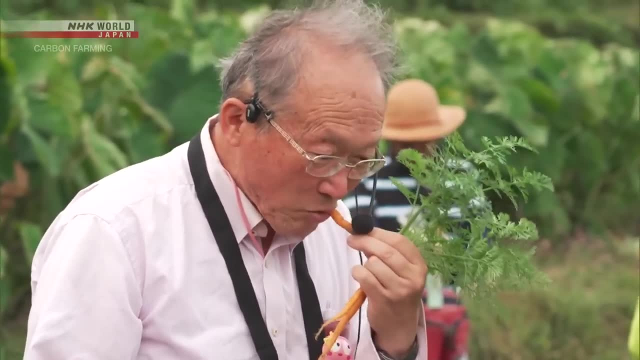 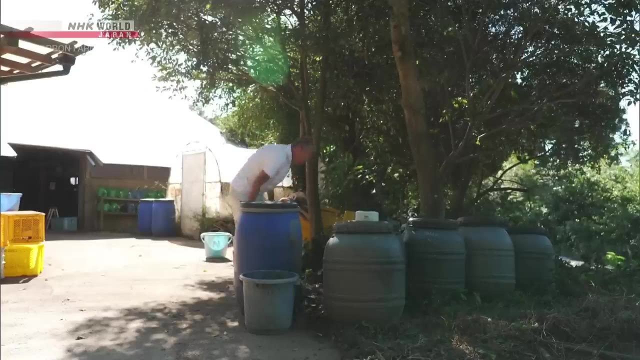 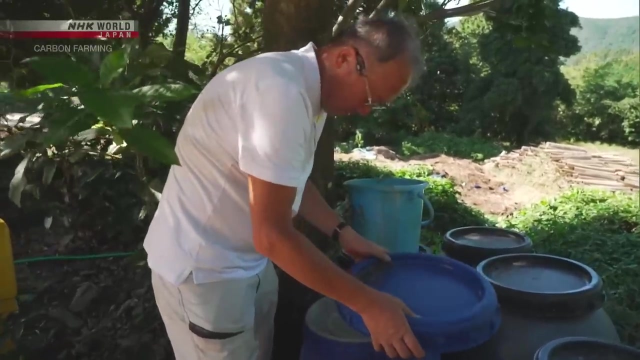 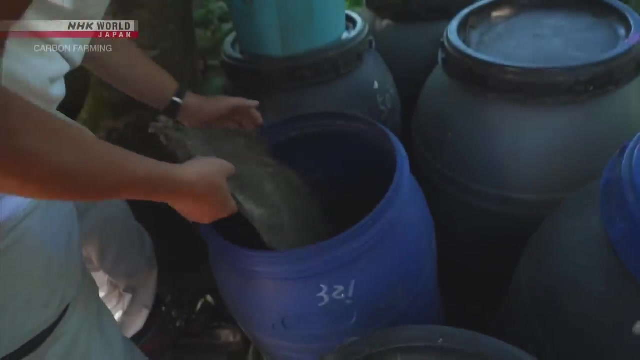 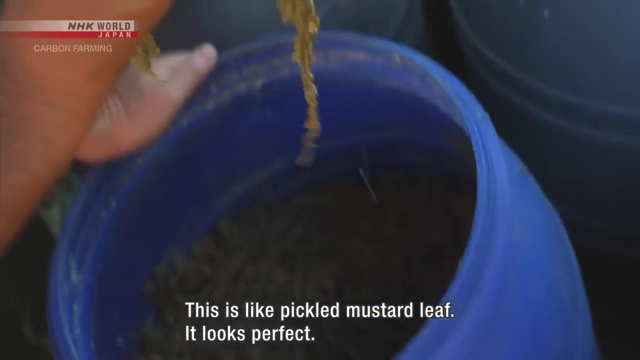 Because the root is Kin-chan right. Kin-chan is attached to it. He refers to microorganisms as his friends and affectionately calls them Kin-chan or deer bacteria. Yoshida makes his soil using things that are easily available To make natural fertilizer. 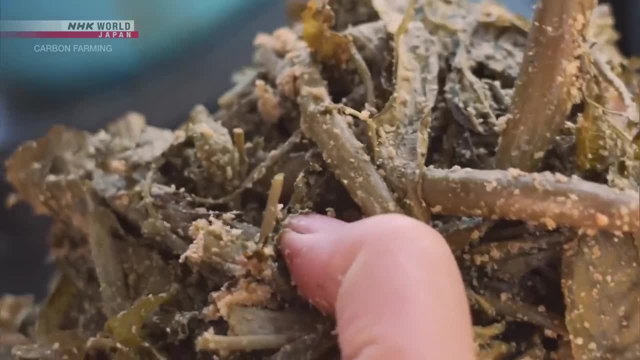 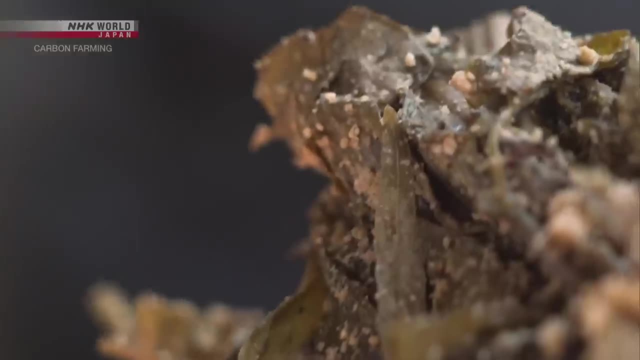 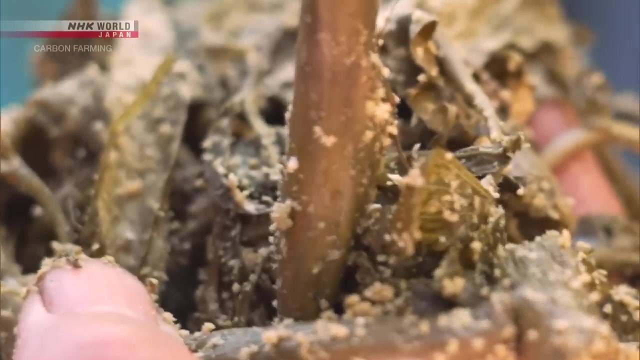 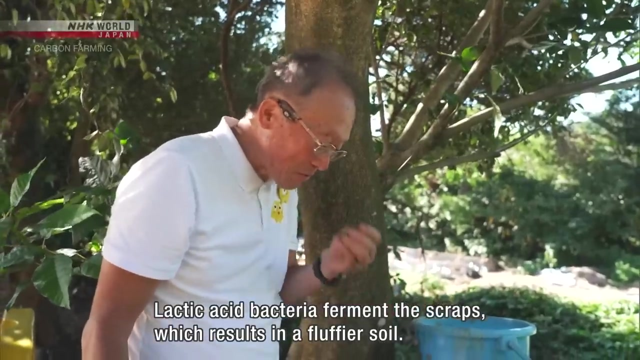 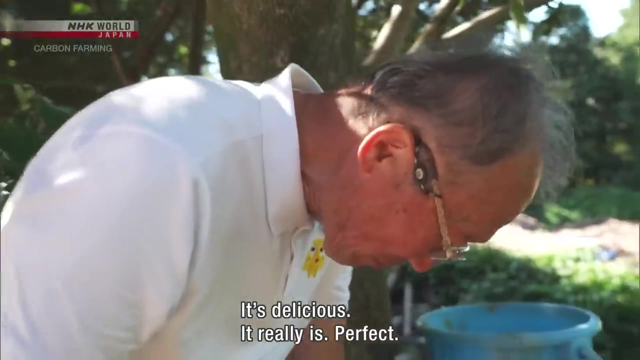 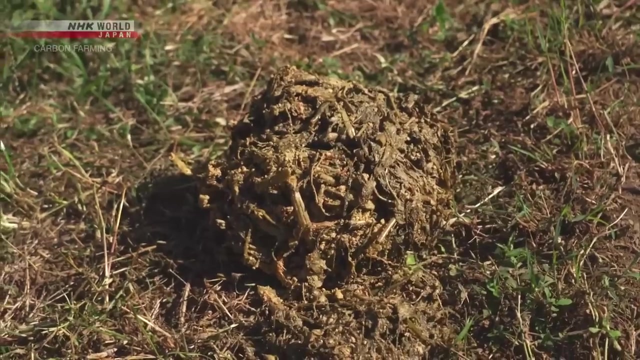 he ferments food scraps that people would normally throw away. He puts them in airtight containers and adds rice bran and salt. It's a method similar to that for making Japanese pickles. After about a month of fermentation, he mixes the food scraps into the soil. 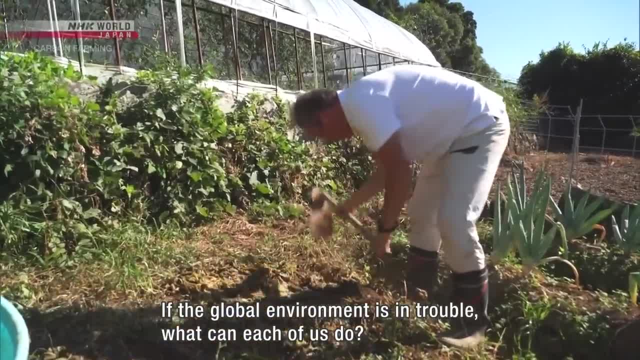 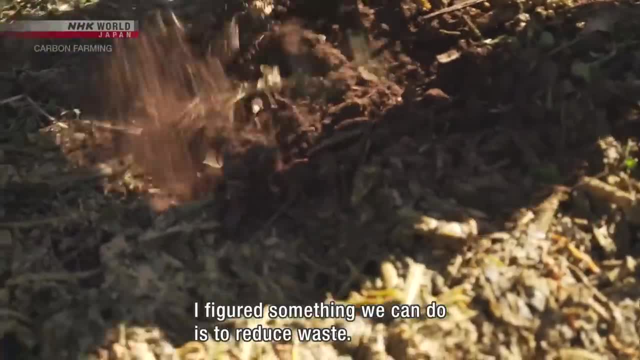 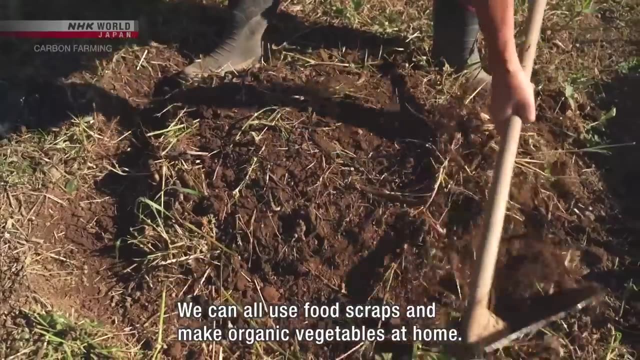 When I heard that the global environment was in danger, I wondered if we could do something about it. What we can do is reduce the amount of garbage. We can use the garbage to make organic vegetables in our own homes. We can use the garbage to make vegetables. 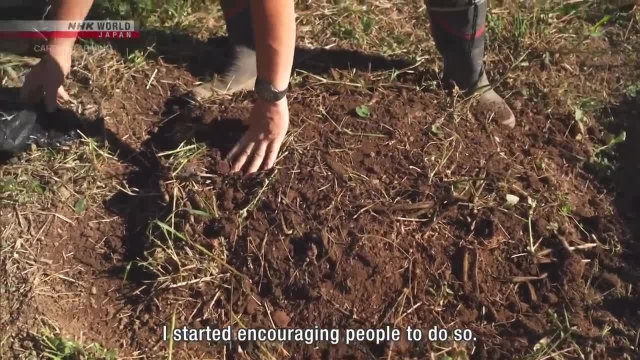 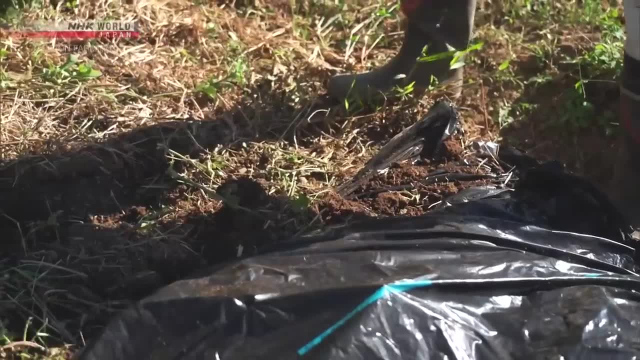 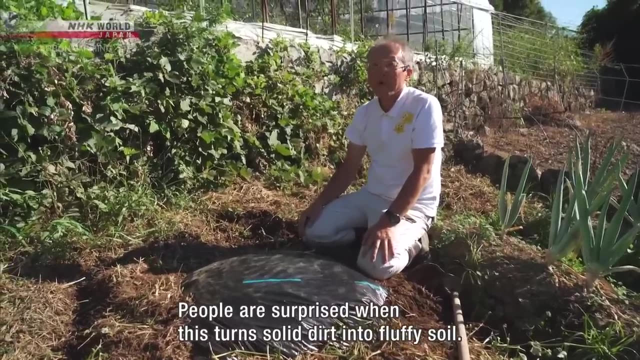 We can use the garbage to make vegetables. Yoshida tightly covers it with a black plastic sheet. After waiting for about a month, the soil will be rich and ready. If the soil wasn't good in the first place, everyone would be surprised. 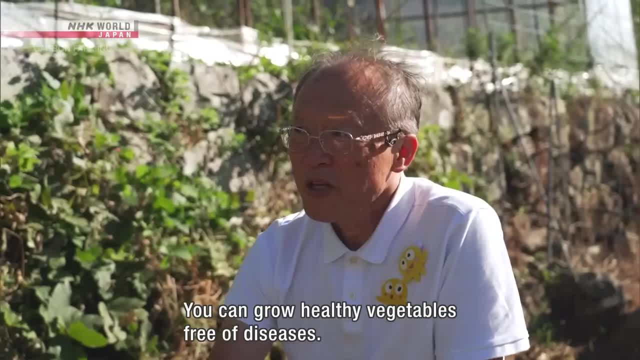 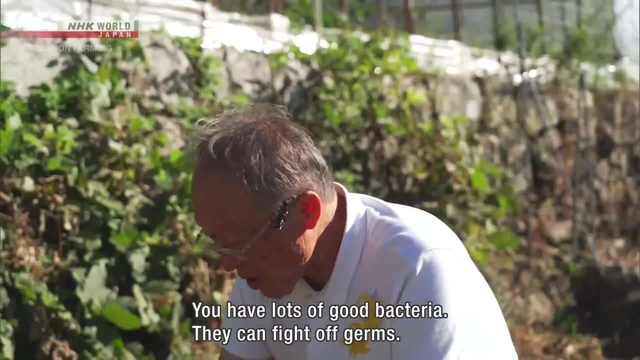 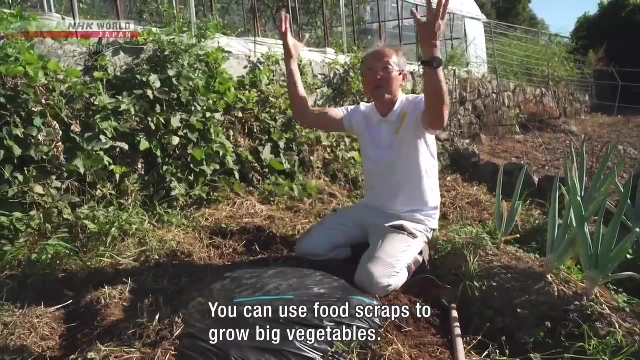 The soil would be rough and fluffy, But we can make good vegetables. The disease will go away. It's just good bacteria. Even if we get sick, we'll fight over it. The garbage we throw away will make the vegetables bigger. Yoshida used to work for the local government. 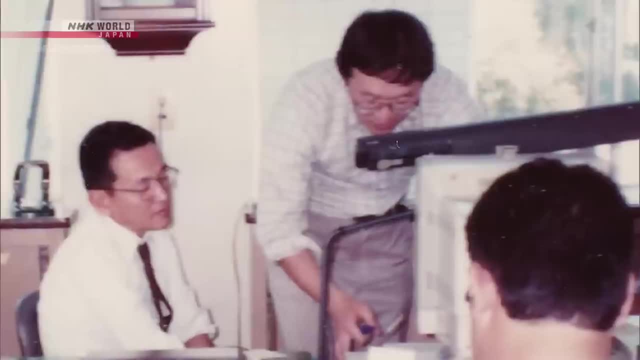 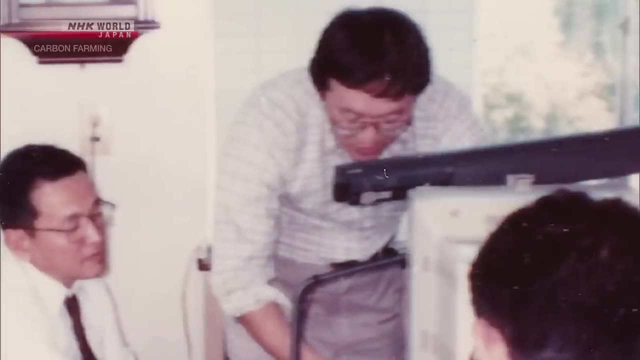 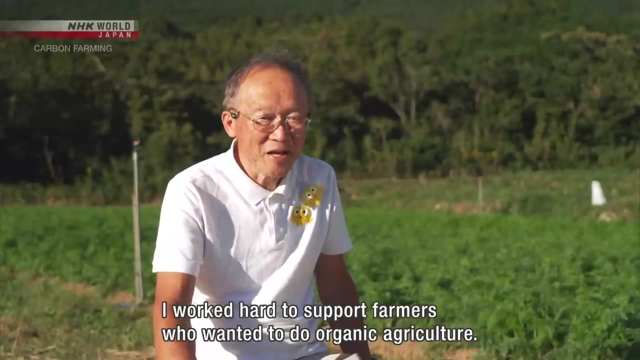 as an adviser for farmers. He started to question conventional farming because it relies on chemicals, So he encouraged farmers to go organic. If there are people who want to do organic farming, we'll support them. We've been doing our best, But things don't go well. 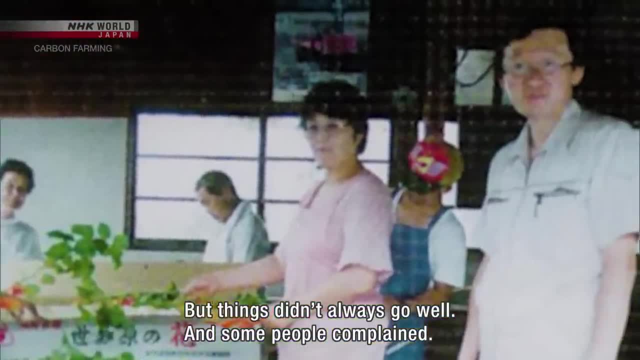 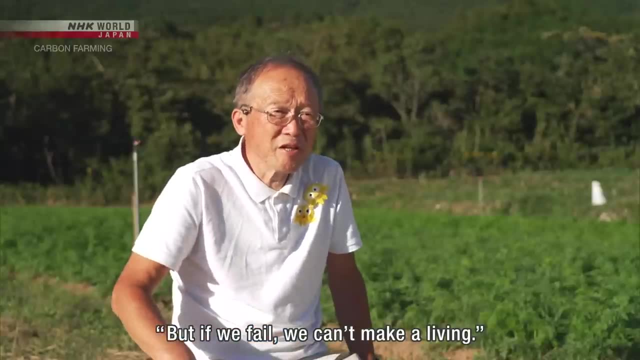 When things didn't go well, he got angry. He said: you're going to change the agriculture. You're a farmer. If we fail, we won't be able to live. He said: if we fail, we won't be able to live. 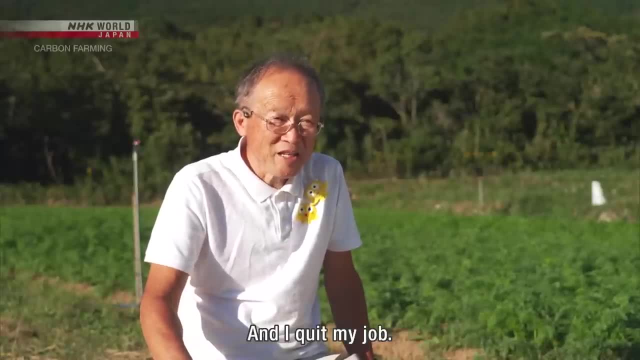 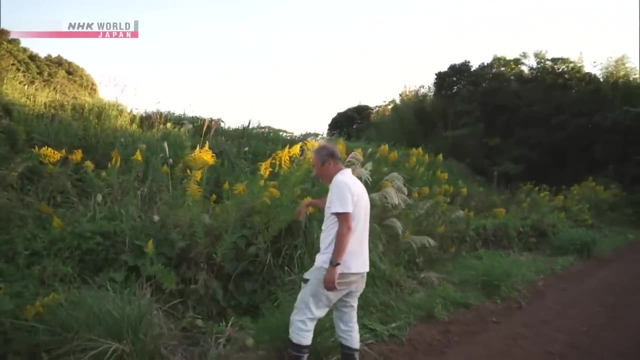 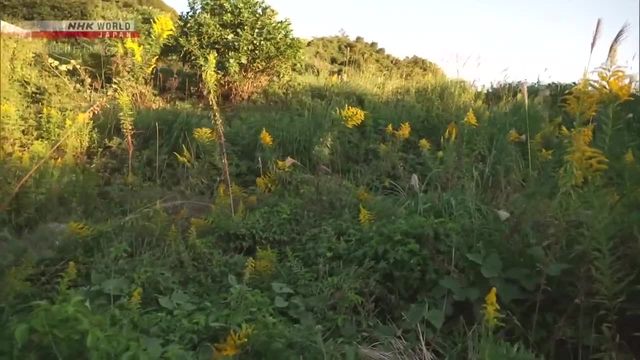 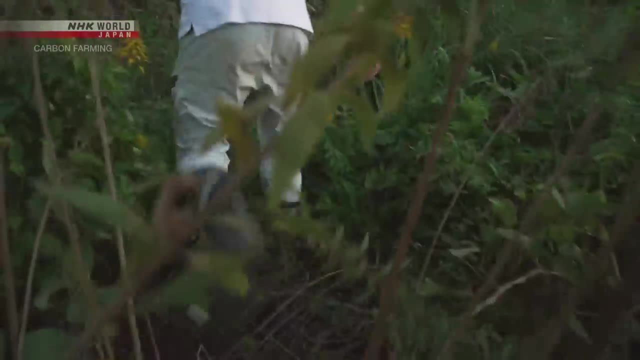 we won't be able to live. When he became the prefectural government, Yoshida became a farmer. It wasn't easy, though. He could only rent barren fields that had been abandoned for some time, But that was a blessing in disguise. 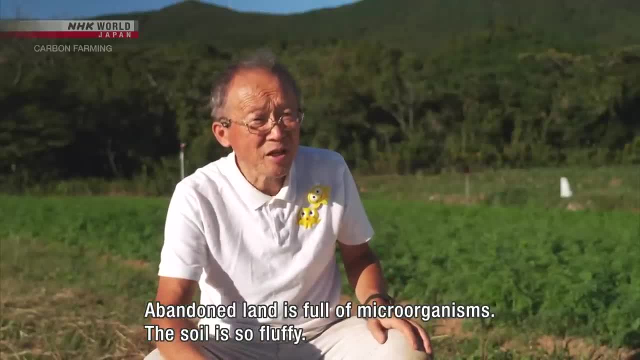 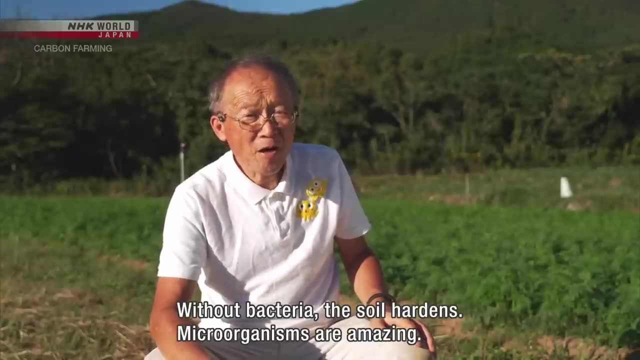 There are so many microorganisms in Kozakoukushi and the soil is so soft. If you use it for a few years, it becomes hard again. When there are no more microorganisms, it becomes hard again. I realized that there are so many microorganisms. 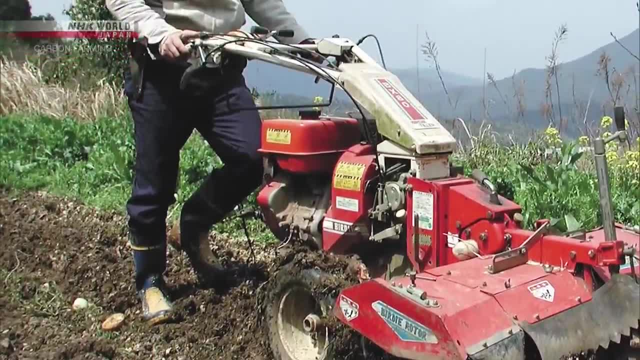 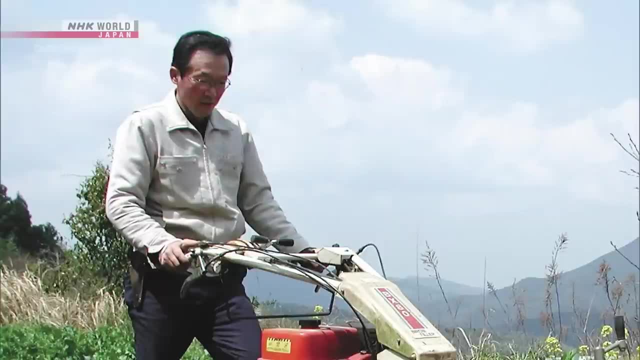 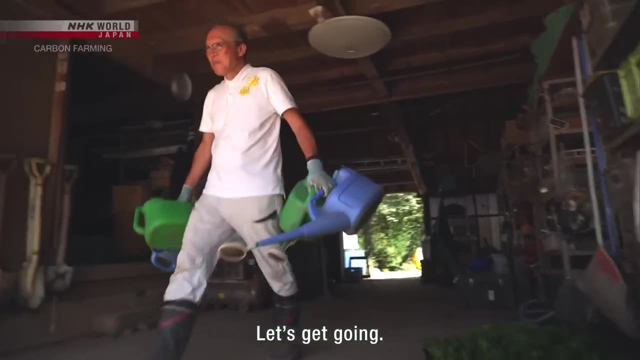 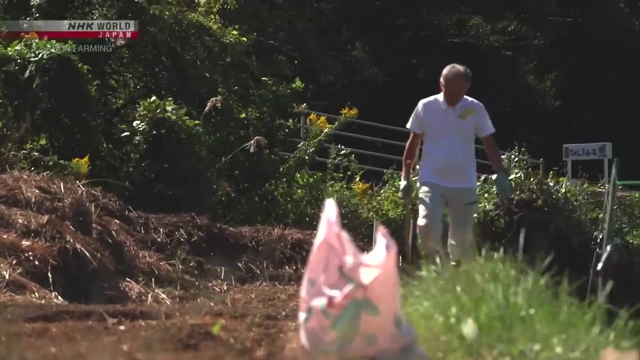 By growing vegetables on deserted farmland, Yoshida experienced the power of nature first-hand. That marked the beginning of his partnership with microorganisms. I'm going to go now, but the weather is so nice today. Yoshida has tried many things to figure out. 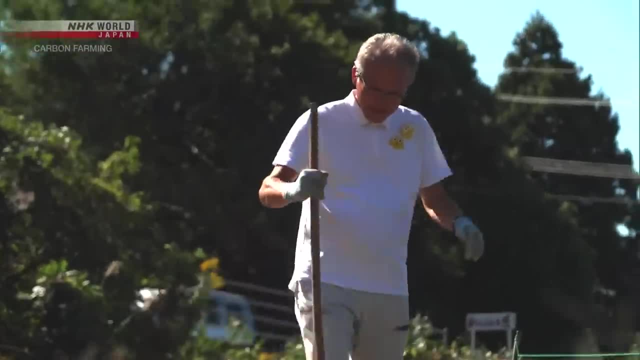 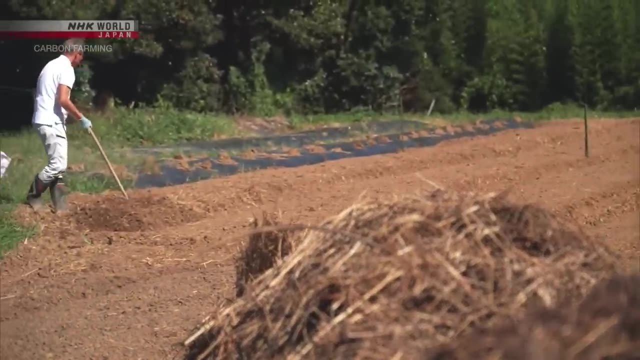 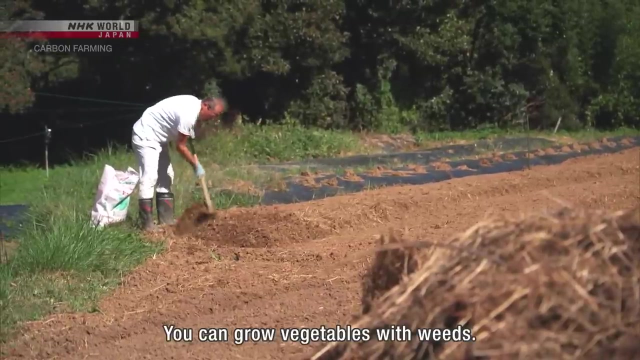 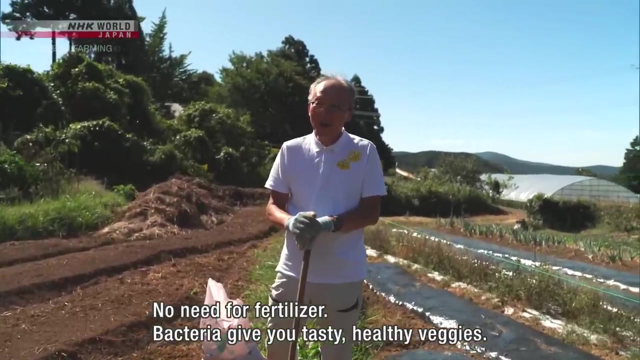 how best to grow microorganisms in the soil of his fields. Right now, he's focusing on making soil using weeds, things that farmers usually don't want. We can grow vegetables using weeds. We don't need fertilizers. If we can connect with microorganisms, we can grow healthy vegetables. 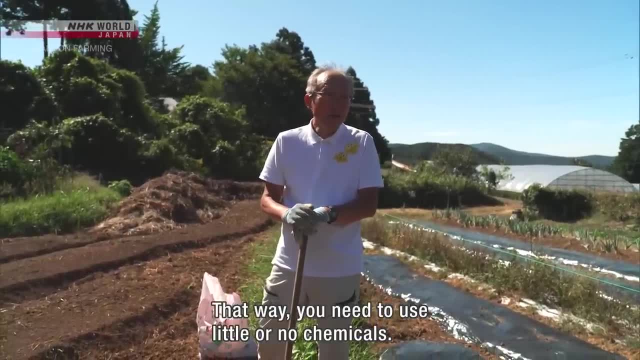 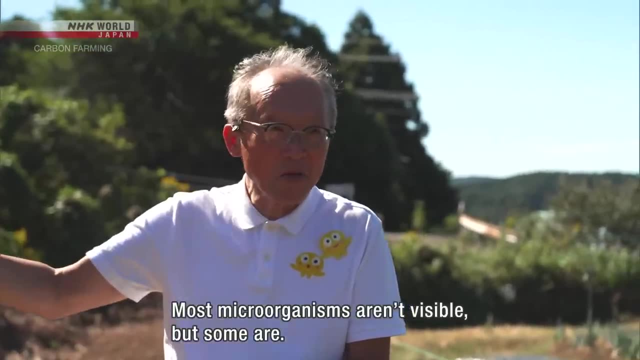 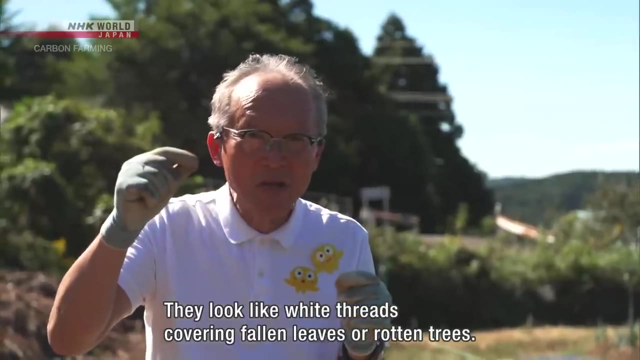 We don't have to use pesticides or other pesticides. That's how it works. We can't see microorganisms, but there are microorganisms that we can see. They usually grow in the forest. There are white threads on fallen leaves. There are many white threads on fallen leaves and trees with thorns. 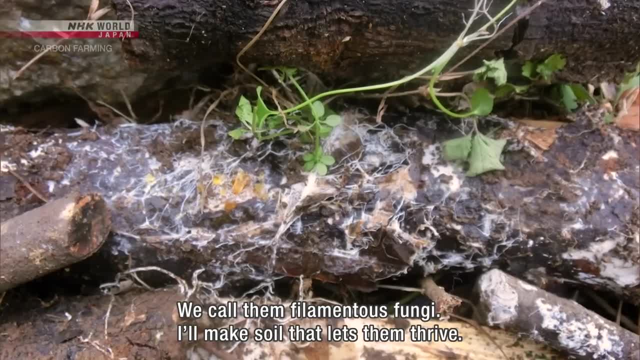 There are many white threads on fallen leaves and trees with thorns. There are many white threads on fallen leaves and trees with thorns. We call that a myelitis. We call that a myelitis. I'm going to make a soil that can increase that myelitis. 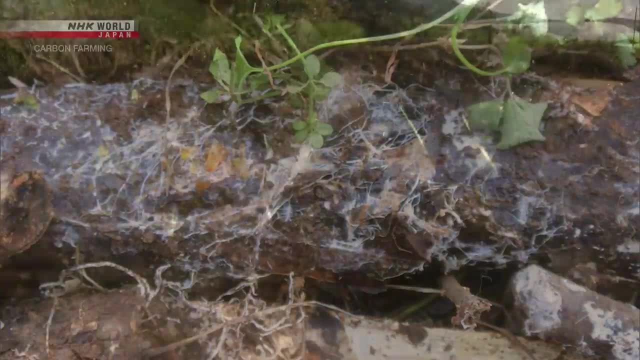 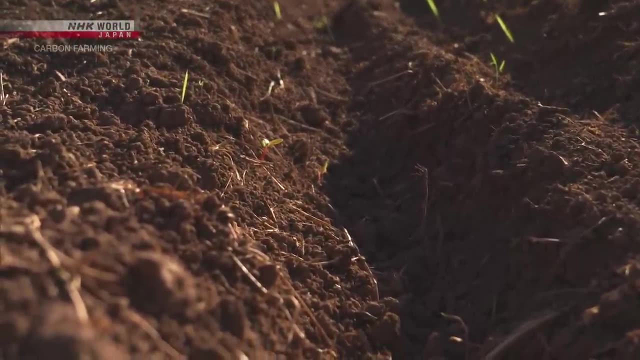 Filamentous fungi are microorganisms commonly known as mould. Yoshida shows us how using weeds can help encourage their growth. I'm going to make a high-heeled urn. The reason why I'm going to make a high-heeled urn is because 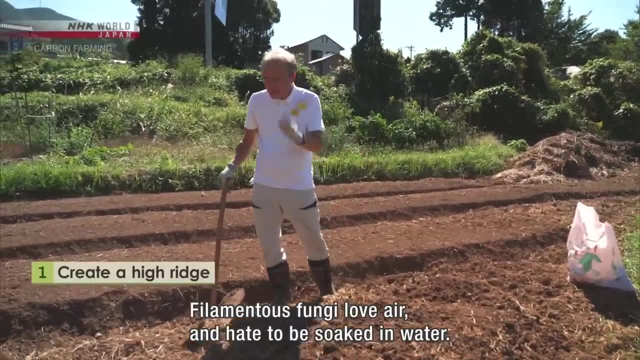 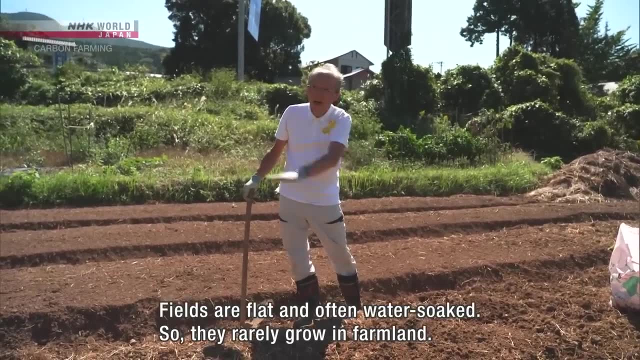 myelitis likes air anyway. myelitis likes air anyway. Myelitis likes air anyway. I don't like water. I've only been in the forest. The fields are horizontal so it's easy to get water. I've only been in the forest. 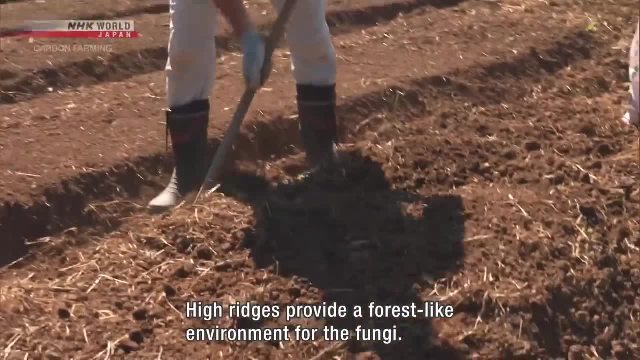 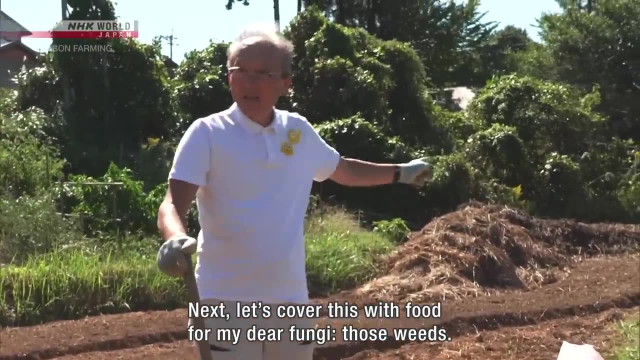 That's why I made a high-heeled urn on the slope to get closer to the forest. Next I'm going to put Kin-chan's food here. That's grass. Yoshida places about five kilograms of weeds per square metre of soil. 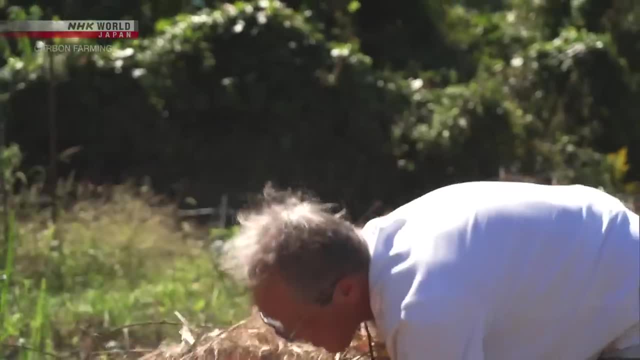 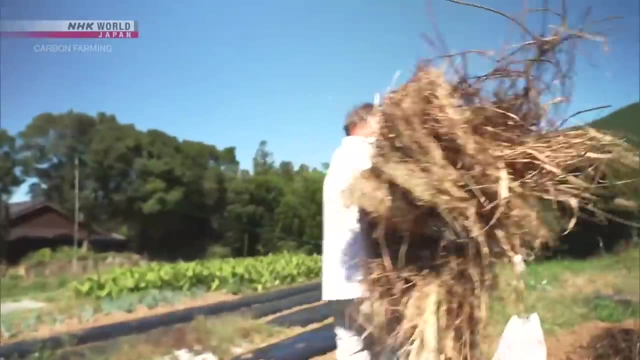 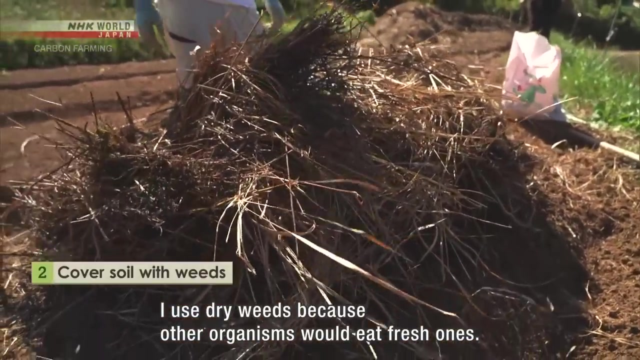 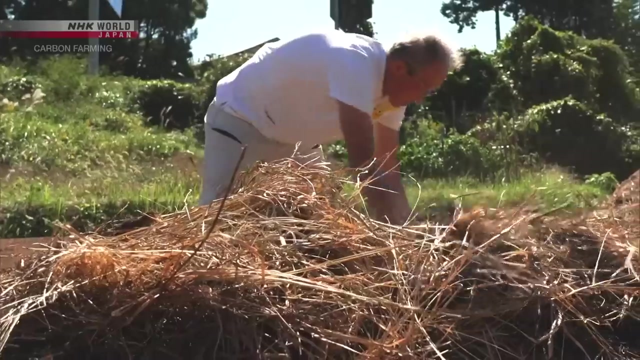 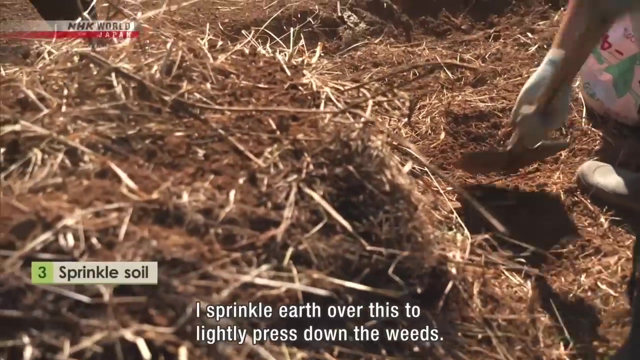 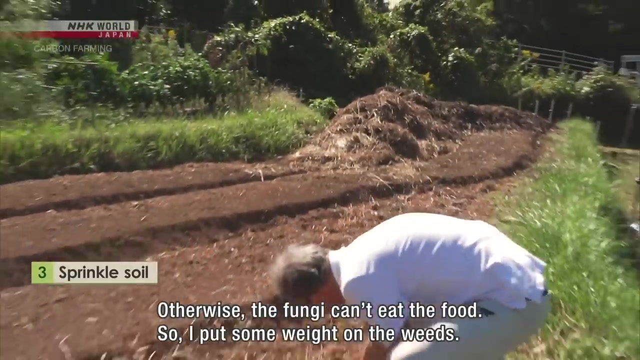 Yoshida places about five kilograms of weeds per square metre of soil. Hard fibrous weeds contain a lot of carbon, so they're a good choice as food for filamentous fungi. Push it down into the air. The grass has to be pressed down so that the microorganism cannot eat it. 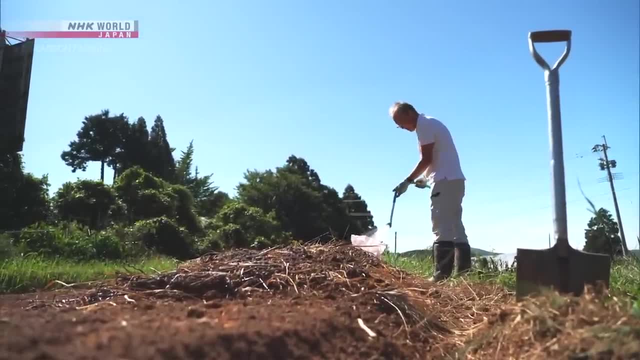 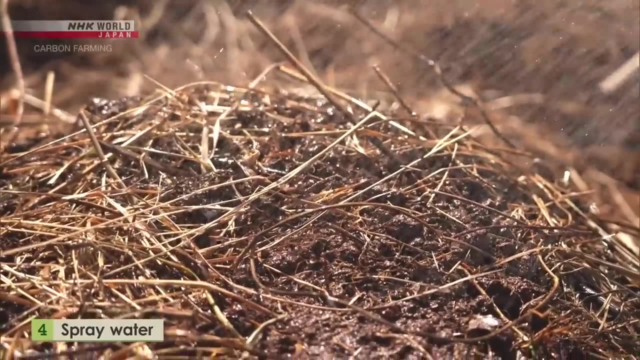 OK. If the weeds are too dry, that slows decomposition by the fungus. If the weeds are too dry, that slows decomposition by the fungus. If the weeds are too dry, that slows decomposition by the fungus. so Yoshida adds a moderate amount of moisture. 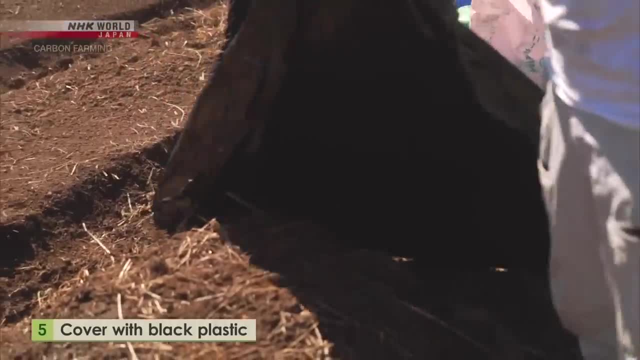 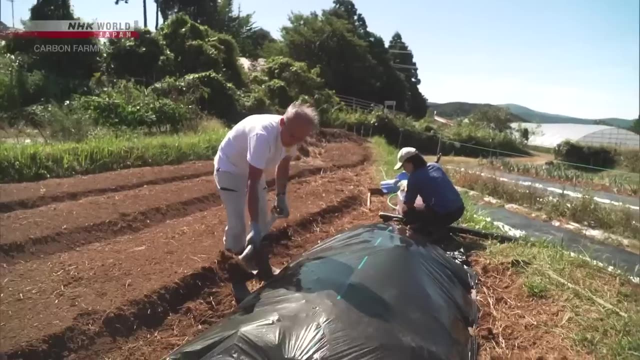 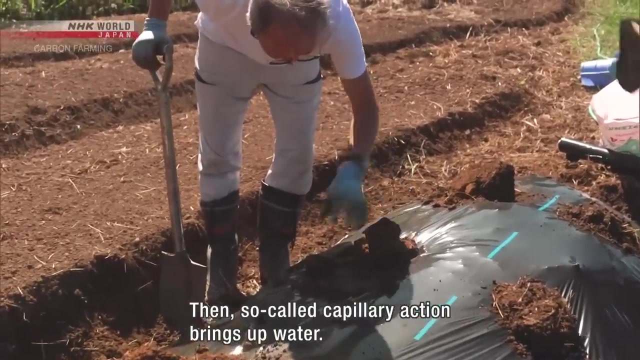 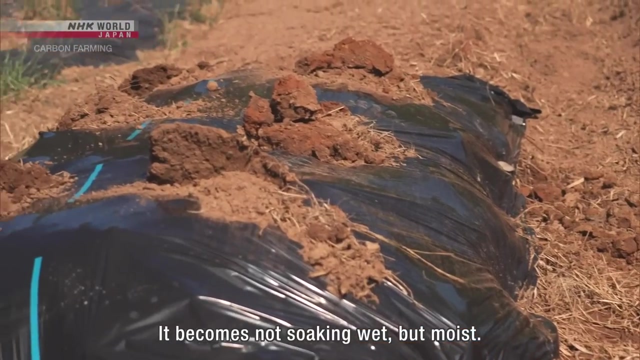 To promote active growth of the filamentous fungi, he covers the ridge with a plastic sheet to keep it moist. If you cover it with a plastic sheet, it will be clogged. This will cause the water to come up. It won't be wet, but it will be damp. 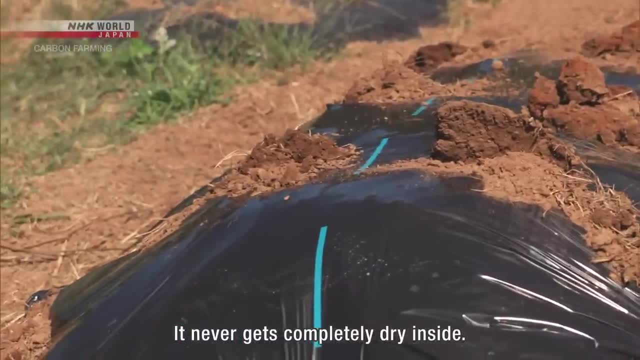 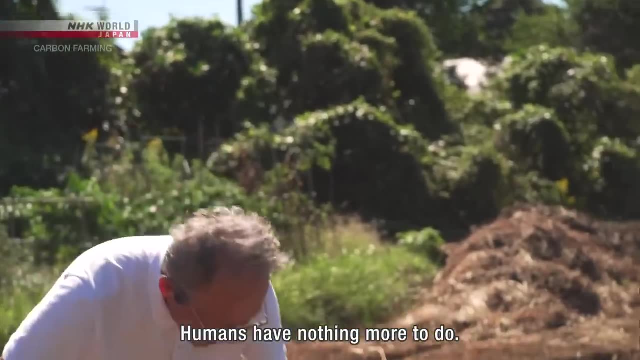 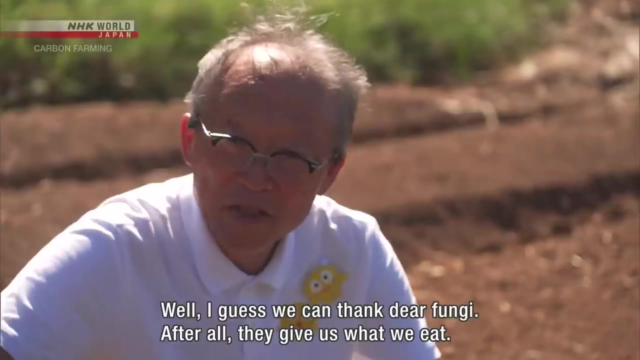 It will never become dry. That's how it works. This is perfect. There's nothing else for humans to do. All we can do is say: Thank you, Kin-chan. Thank you so much, Kin-chan. Kin-nyo and I are eating it. 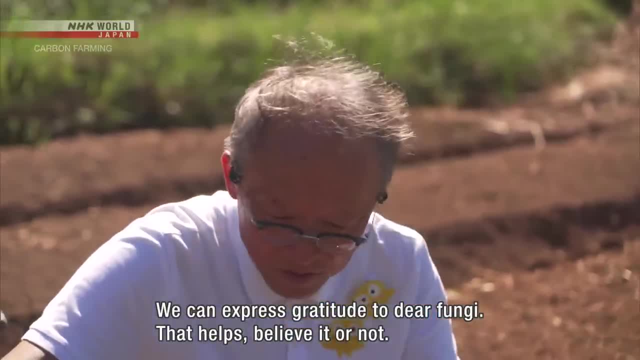 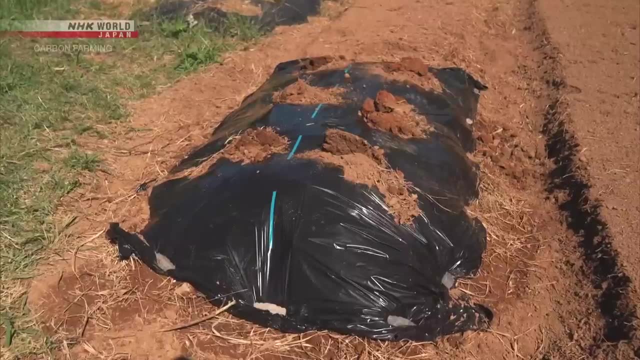 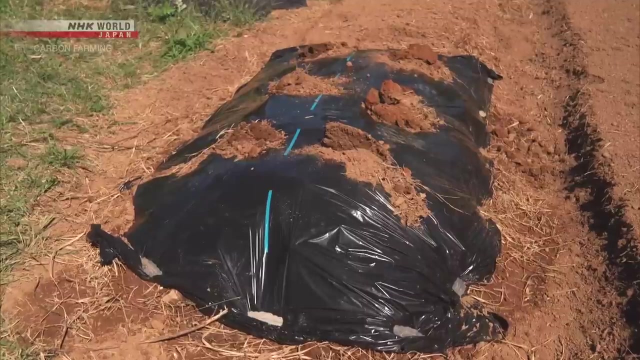 so we just say Thank you, Thank you. That's how it works. It's a bit strange, but it works. The preparations took only 30 minutes. In two to three months, this will turn into fluffy soil With this farming method. 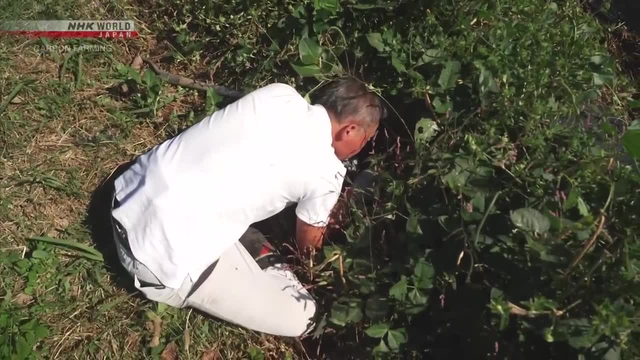 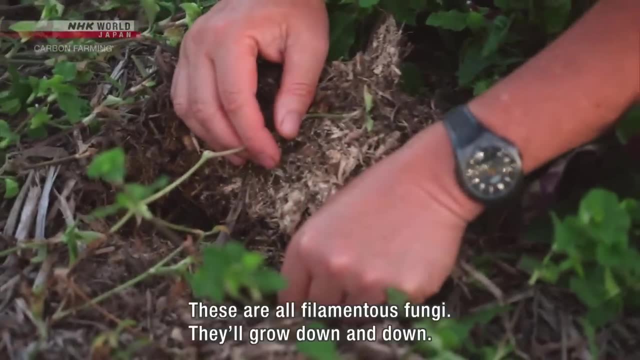 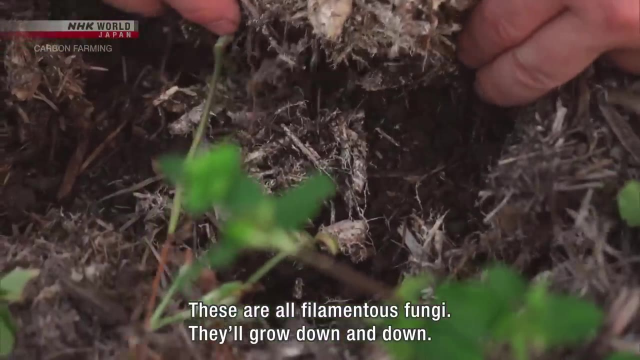 Yoshida created this patch two months earlier. He digs a little and there they are. This is all new. This is all new, All of it. This goes all the way inside. Filamentous fungi cover the surface of the roots. 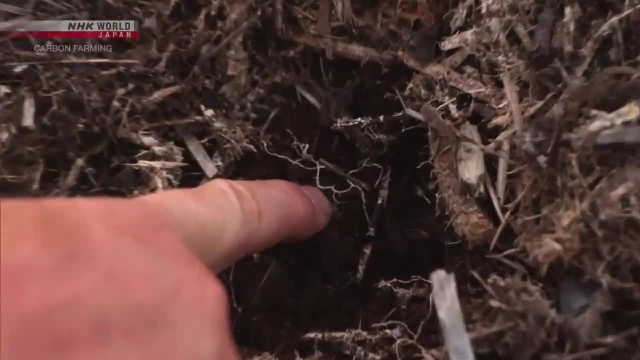 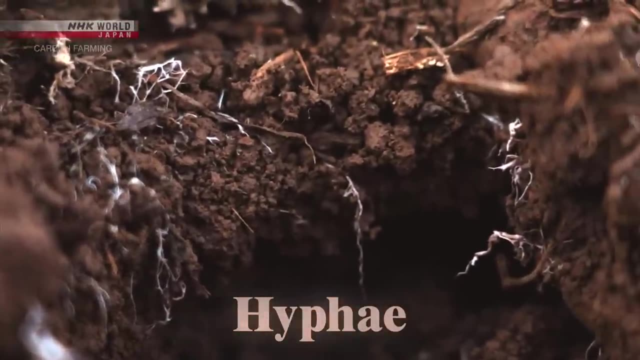 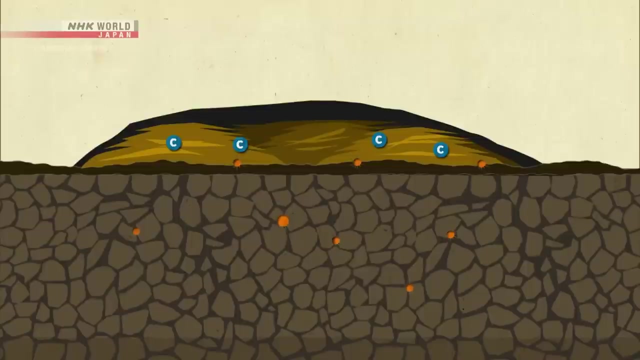 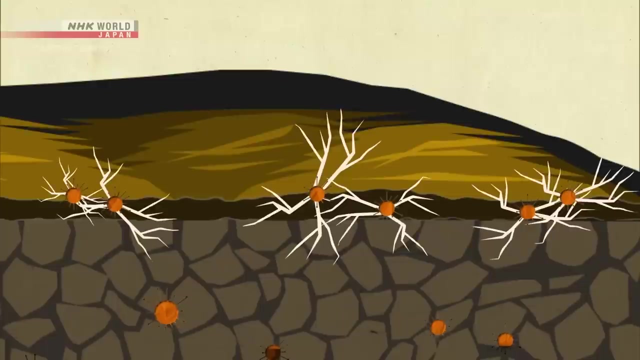 The fungi have grown quite a bit and have extended thick white filaments called hyphae. The hyphae play an important role in the exchange of nutrients between plants and soil. Filamentous fungi feed on carbon to grow and eventually extend hyphae into the soil. 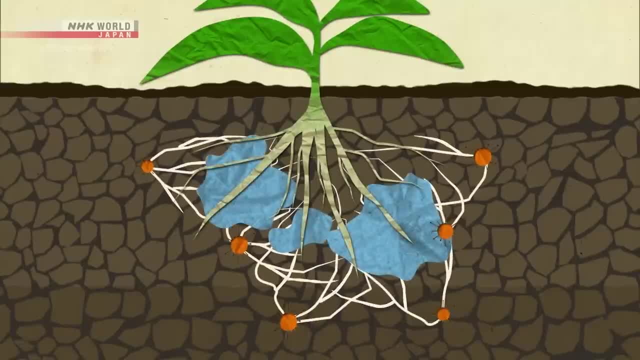 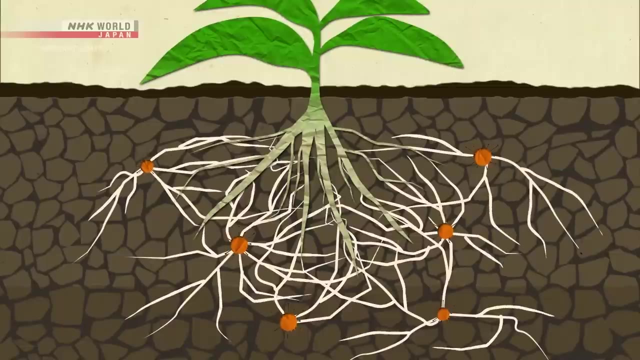 The hyphae are drawn to the carbon released by the plant's roots. They attach themselves to the roots as they grow, supplying plants with nutrients, minerals and moisture. The hyphae have developed a symbiotic relationship with the plants, now serving as extra roots that help the plants take in nutrients. 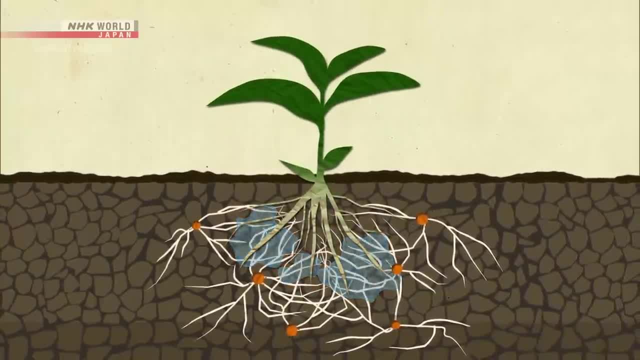 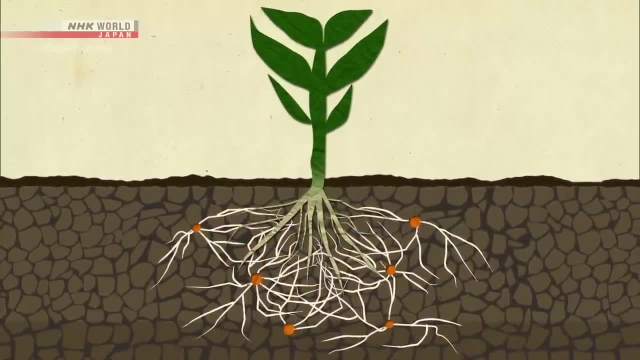 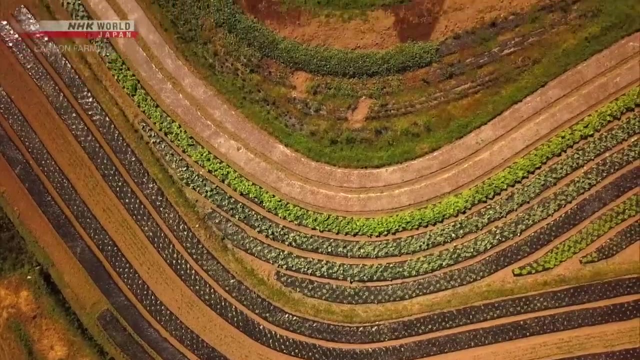 With the help of the fungi, crops absorb more nutrients and grow vigorously. The hyphae can grow even more nutrients. The hyphae can grow even more nutrients. Yoshida finds all the nutrients he needs to grow crops in the ground, courtesy of the microorganisms. 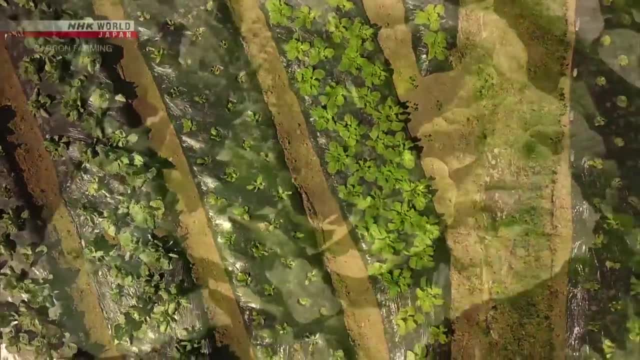 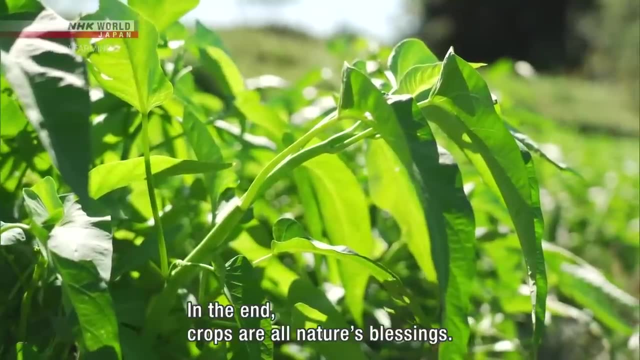 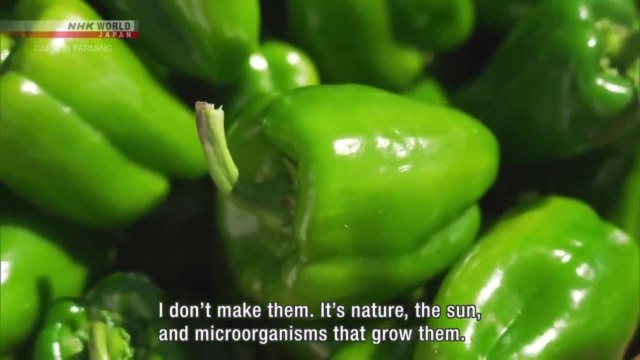 He says crops grown in such a way are more resilient against disease and pest infestation. In the end, everything is a blessing from nature. I didn't make the hyphae. Nature. the sun and the microorganisms gave me life. 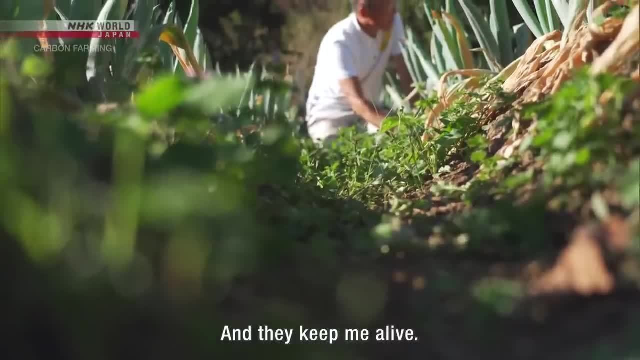 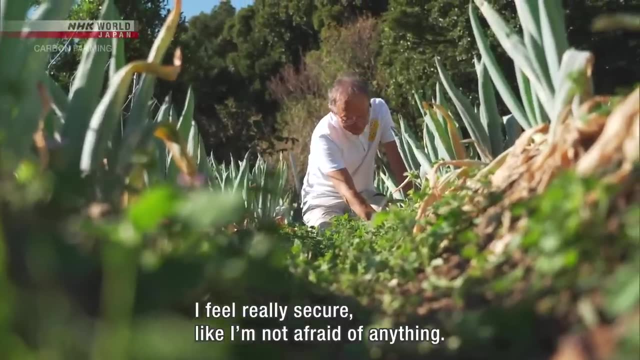 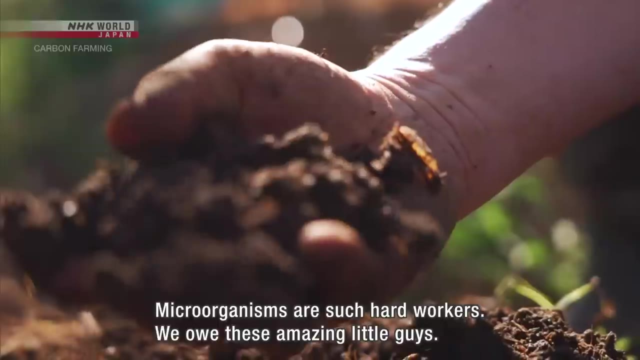 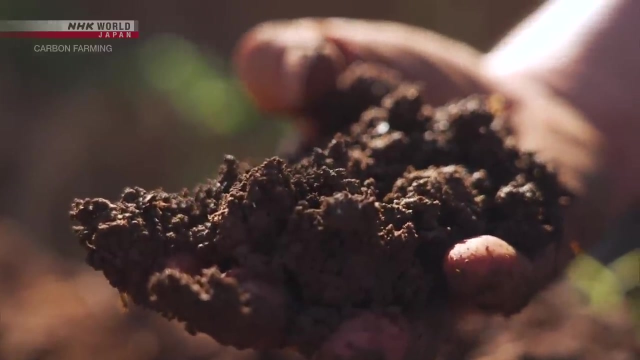 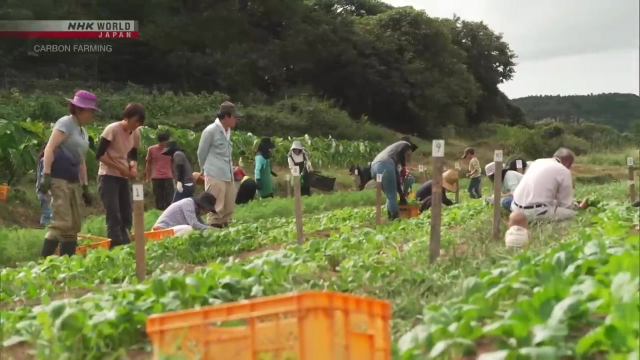 I'm being brought to life in nature. I feel very secure. I'm not afraid of anything. I'm doing my best. It's all thanks to the hyphae. It's strange. It's strange. Yoshida travels around Japan to share his method. 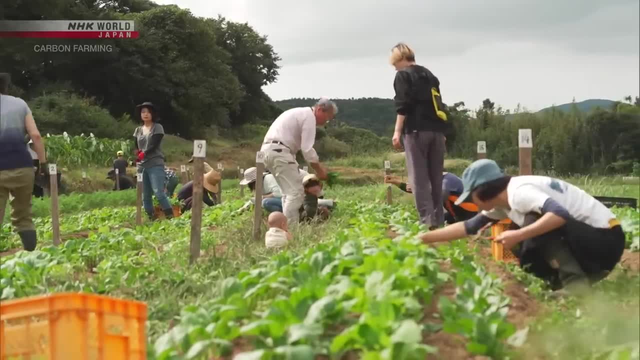 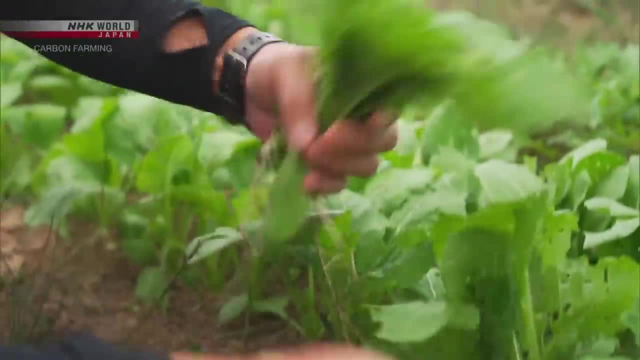 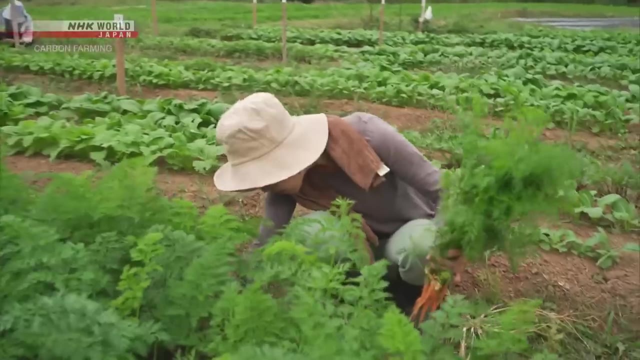 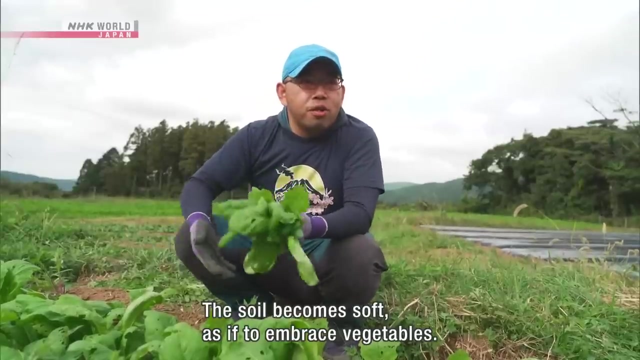 Today he's holding a class on his farm. The participants are learning how to cull vegetables. People from all walks of life attend his class. Some are interested in environmental history, Others are farmers. The soil becomes softer. The soil is ready to accept vegetables. 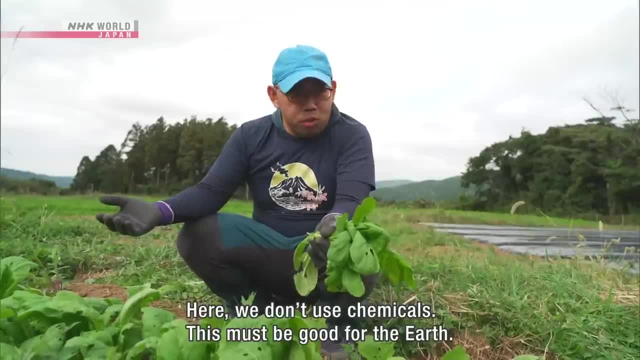 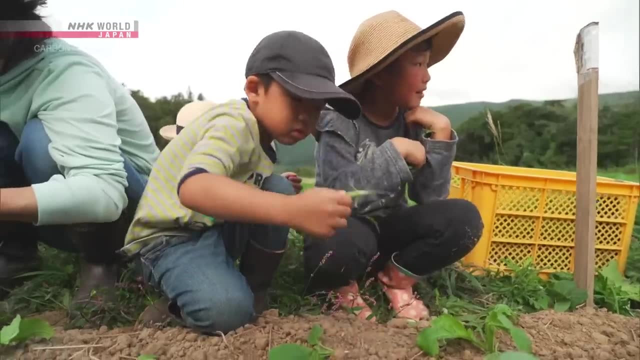 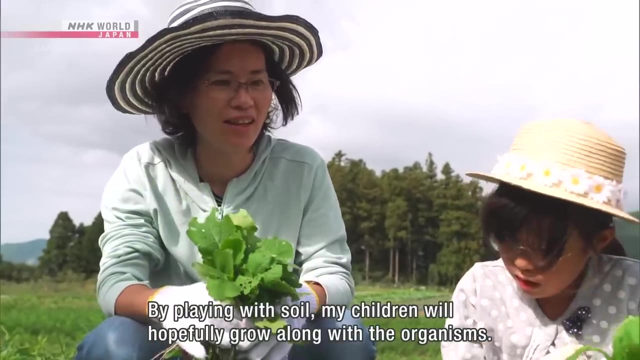 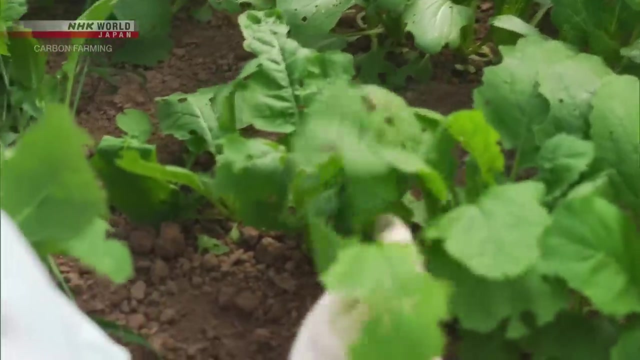 I don't use pesticides, so I think it's good for the earth. I can feel it. I'm touching the soil. I hope the soil grows with the bacteria. I have a corn seed. It's small. It's small. Do you want to hold it? 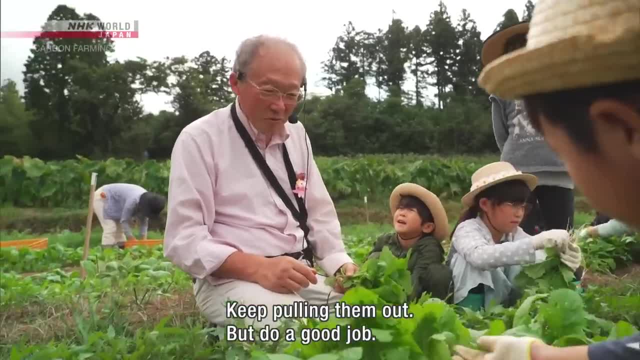 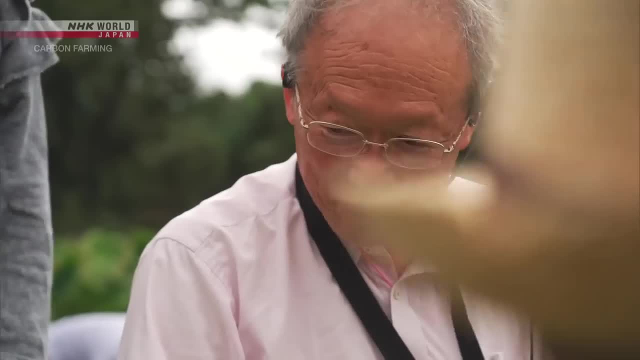 Yes, hold it, It's good. Take it. You can take it, but it's a good idea You can take any. I'll take it, It's good. Yoshida believes in the potential of agriculture and in each of us for solving the global crisis. 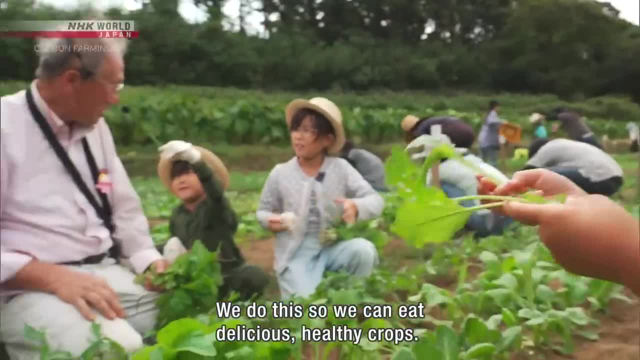 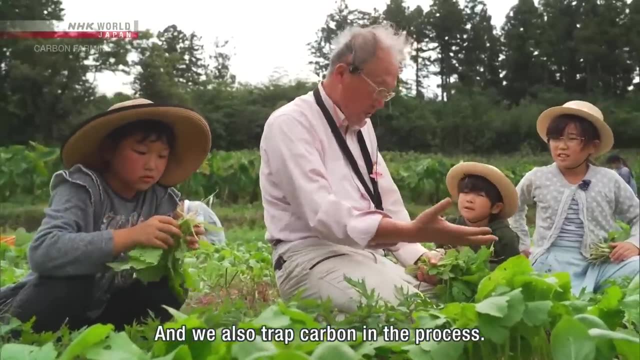 Is it better to take it off by yourself? It's delicious anyway. I do it because it's delicious And I do it because I can eat healthy food. Then, naturally, CO2 can be fixed, Rather than looking for a scientific and special way. 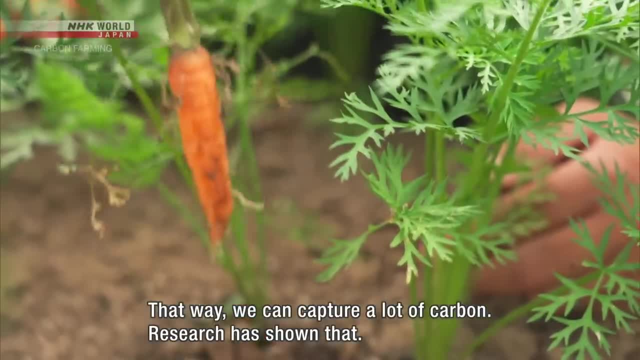 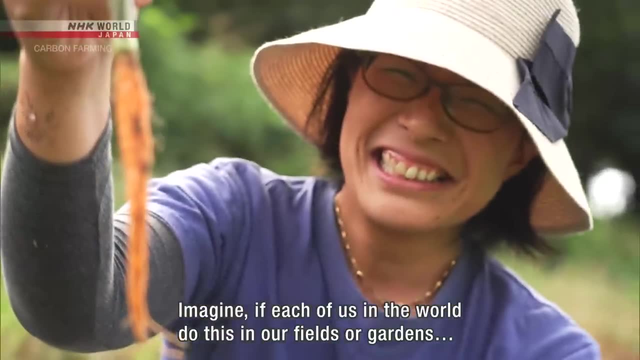 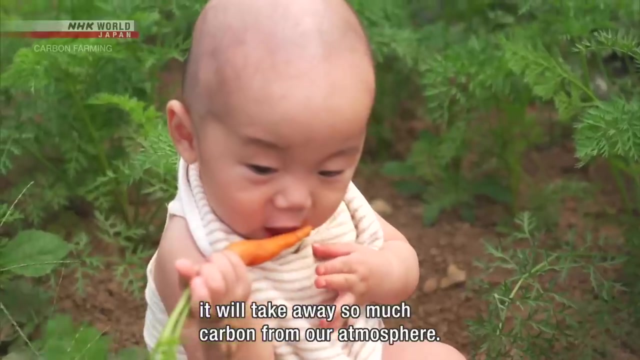 as before, if the earth is full of microorganisms. we know that a lot of CO2 can be fixed by research. When each and every one of us, even the smallest ones, do it in our own fields, it will be a huge amount of CO2 for the whole world. 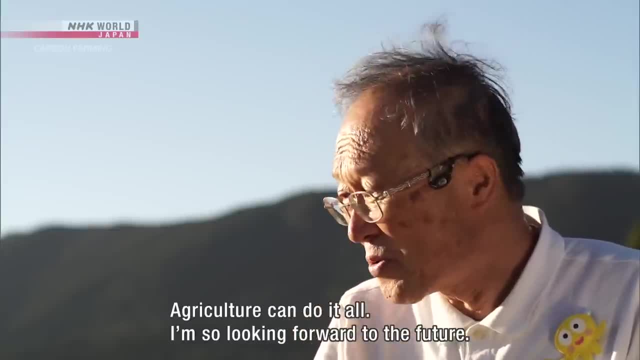 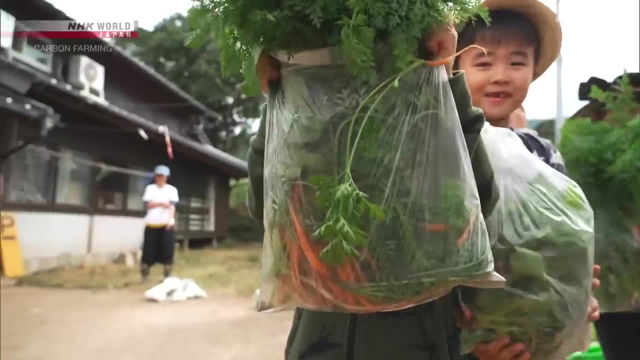 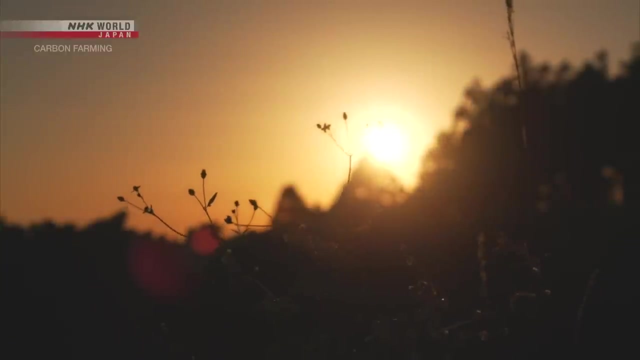 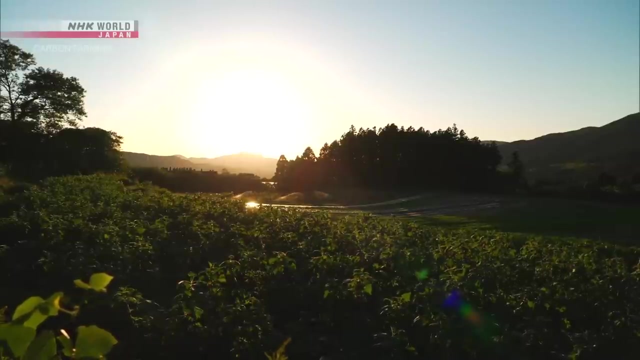 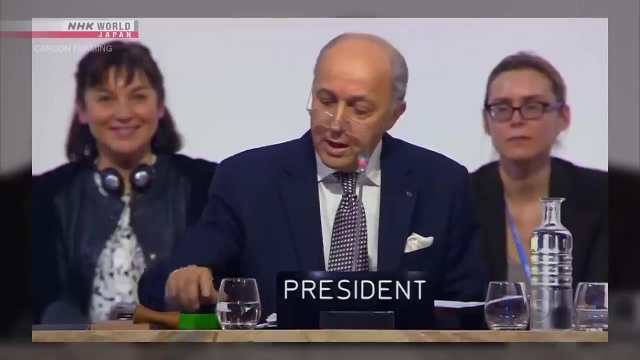 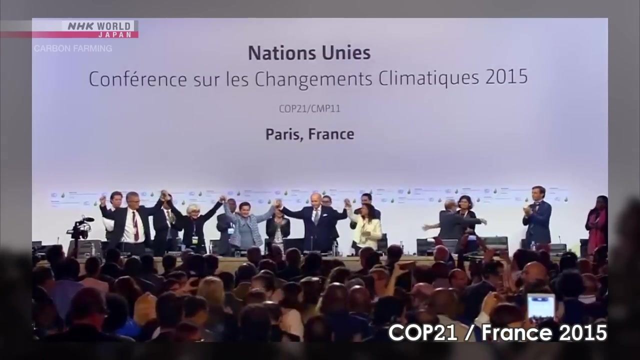 Everything will be fine in agriculture. I'm really looking forward to the future. PART 1: L'accord de Paris pour le climat est accepté. Soil rose to the international limelight. at the 2015 Paris Climate Conference, The French government proposed: 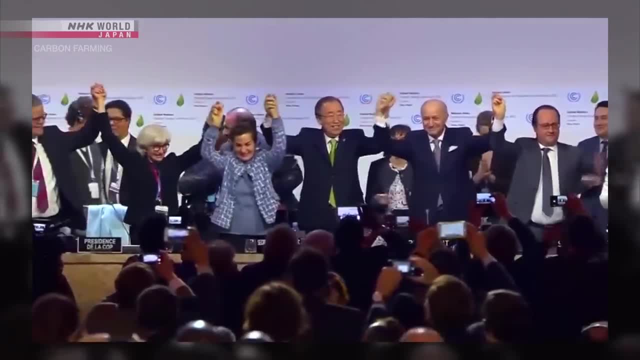 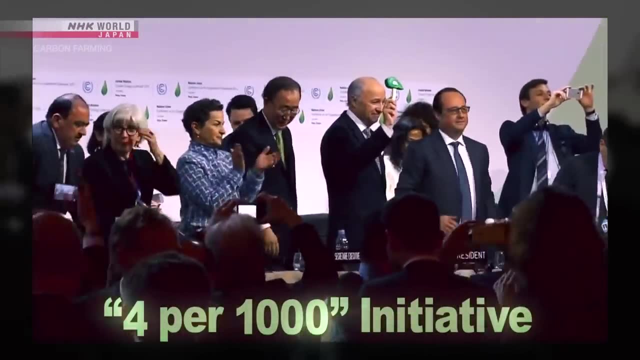 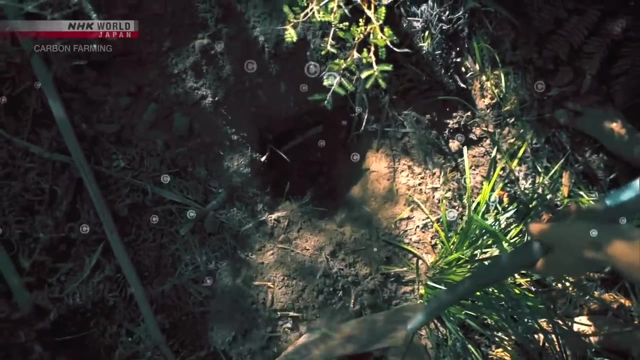 a plan to reduce our carbon emissions. it's called the four per mille or four per thousand initiative. by raising the amount of carbon stored in the earth's topsoil by 0.4 percent annually, or four parts per 1000, we can offset the 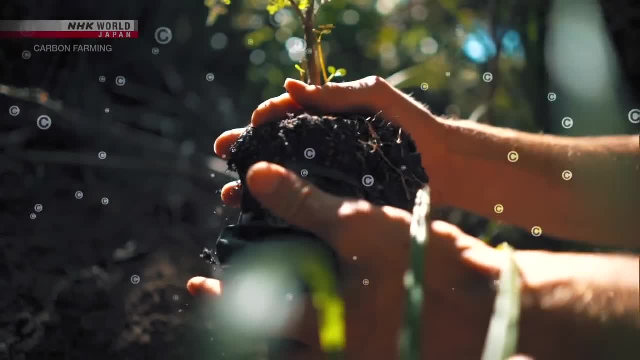 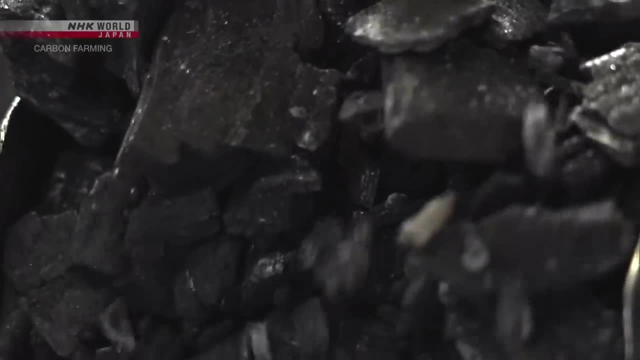 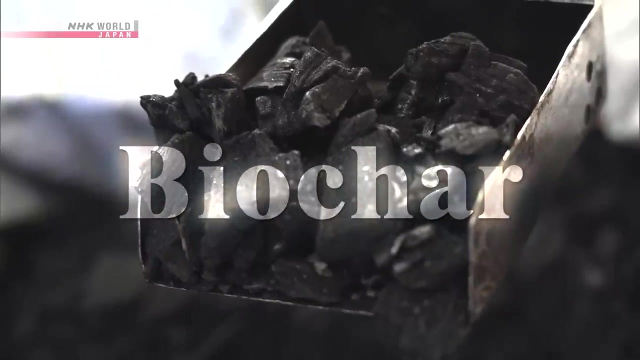 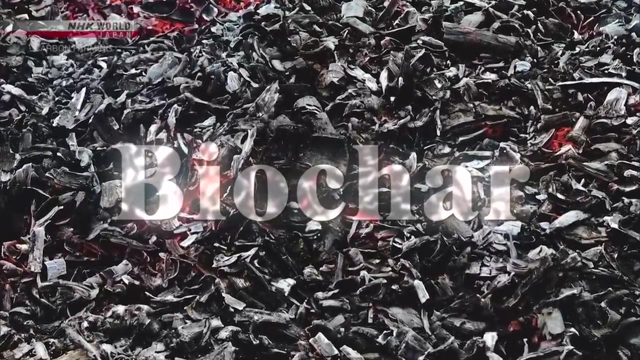 increase in the amount of carbon in the atmosphere. that's the idea behind the initiative. in achieving this goal, people are looking to an age-old material called biochar. it's a type of charcoal made by burning biomass like wood and bamboo. it's used mainly in agriculture. 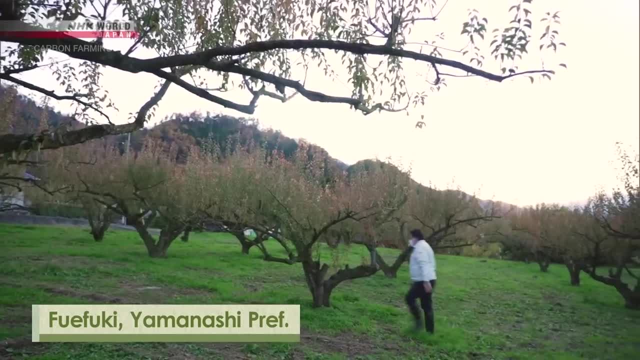 this farm in central Japan actively uses biochar as a source of carbon. for the production of biochar in the atmosphere, it's a type of charcoal made by burning biomass like wood and bamboo. it's used mainly in agriculture. this farm in central Japan actively uses biochar as 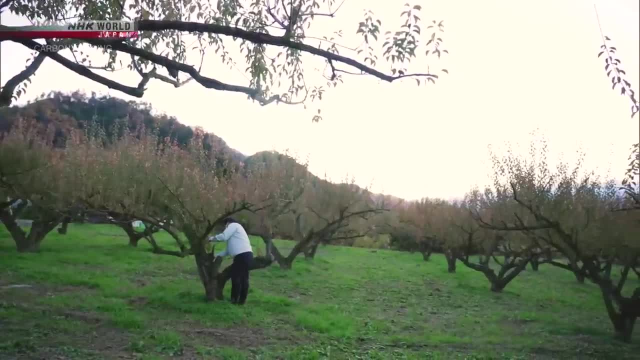 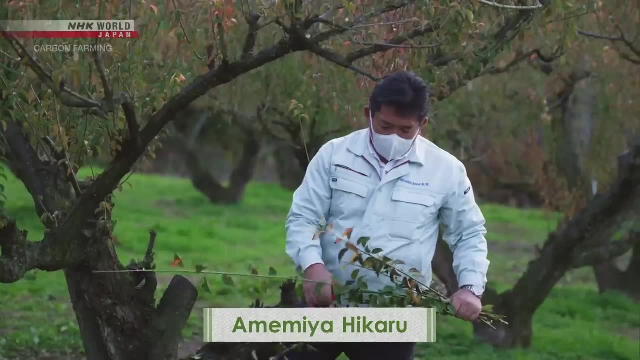 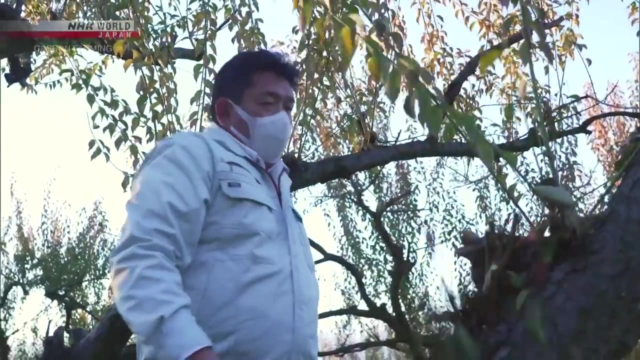 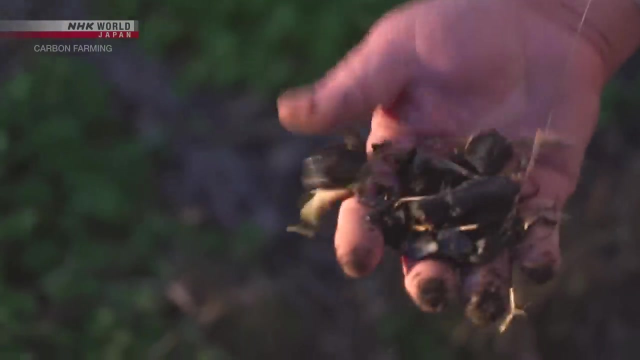 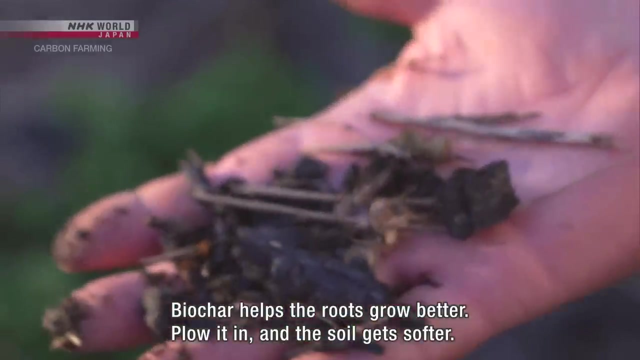 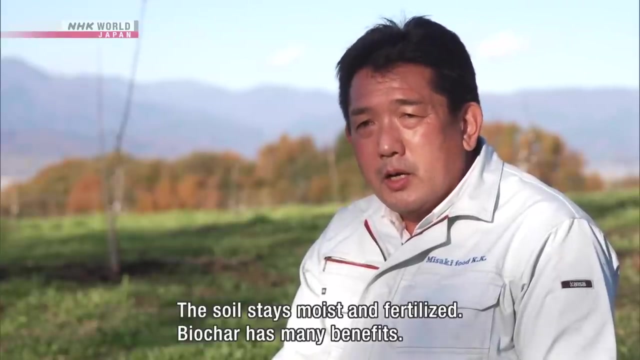 biochar. Amemiya Hikaru is a fruit wholesaler. he and his colleagues have been growing Japanese plums and persimmons for 15 years. they've been employing biochar to improve the quality of the soil in their fields. quite often it has been��mentation and fazla of soil wilted in the past. 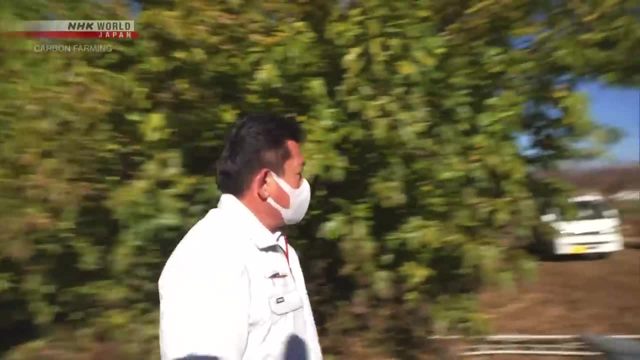 but many do not know how to recover the autoc怎mo are affected easily. The limp vídeos that Amemiya hosts show his work include videos of hoeing and showing how to reap burstingcast cause by being able to throw plants. just you need of a little effort. 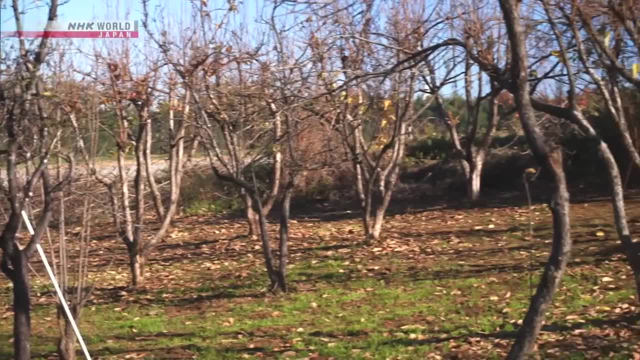 Each year. his work runs quickly, and this area seems to have get better too. Amemiya rents abandoned orchards and revitalises the soil using biochar. Amemiya rents abandoned orchards and revitalises the soil using biochar. Amemiya rents abandoned orchards and revitalises the soil using biochar. 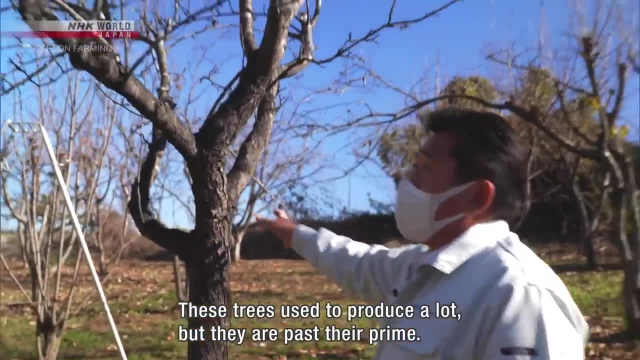 He's an identificator of plants that can't actually grow into himself. He's an identificator of plants that can't really do business. Amemiya vielse the trees, but he manages to grow them from scratch. This is a tree that I've been harvesting and doing my best to grow. 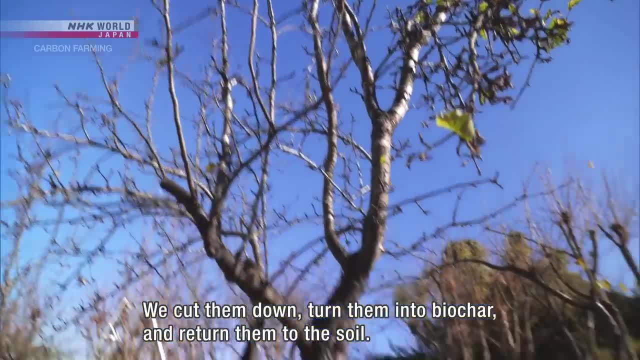 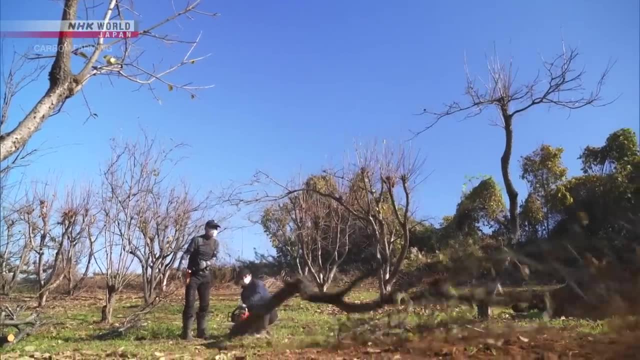 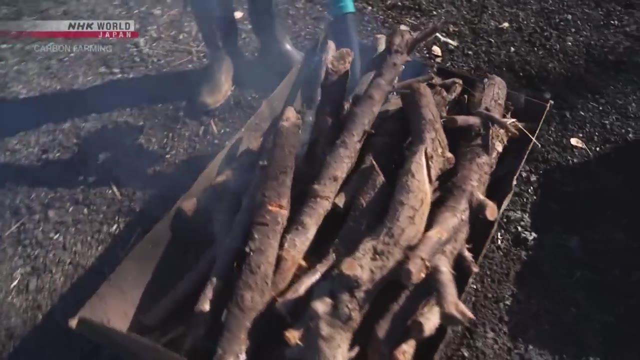 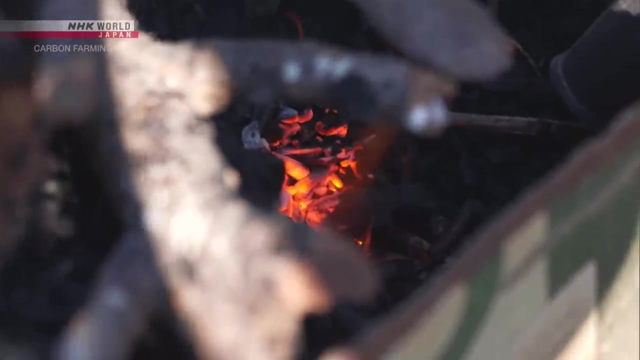 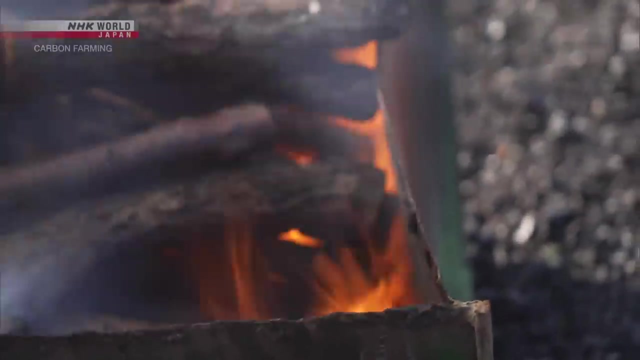 It's a tree that I've been harvesting and doing my best to grow. He waits for about one year for the chopped wood to get dry before turning it into biochar. Trees take in carbon from the atmosphere to grow and extend their trunk and branches. 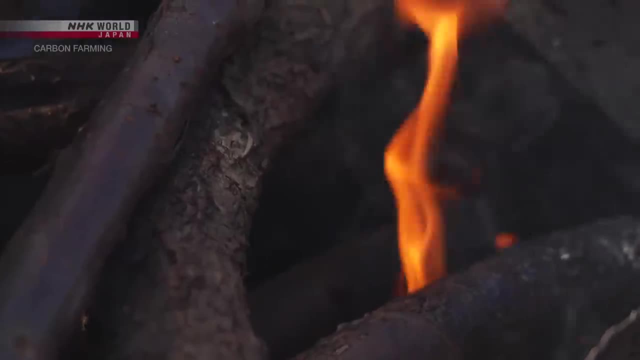 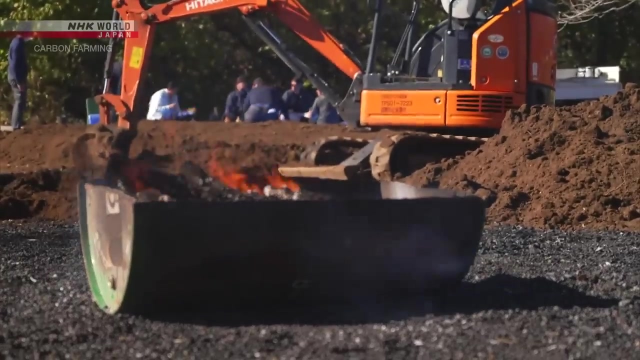 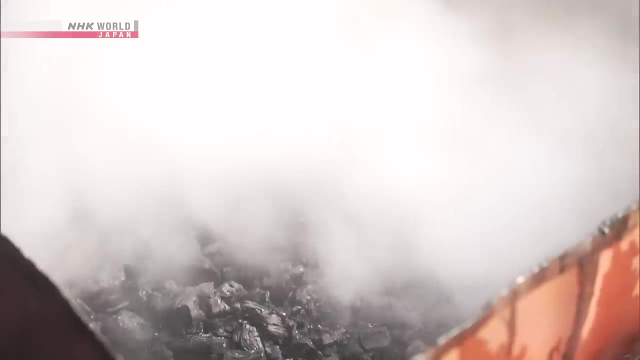 Trees take in carbon from the atmosphere to grow and extend their trunk and branches. By turning them into biochar, the absorbed carbon can be locked in for 100 to even 10,000 years. Before the wood is completely burned, water is poured over it and the biochar is ready. 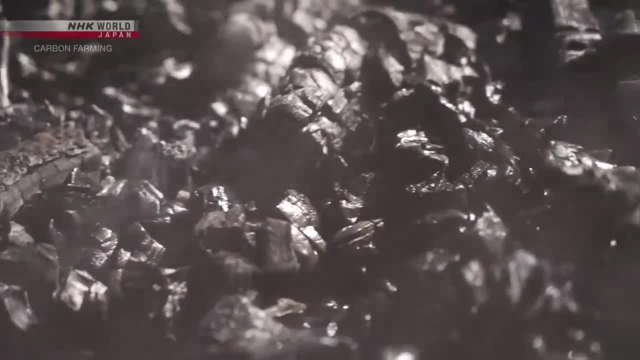 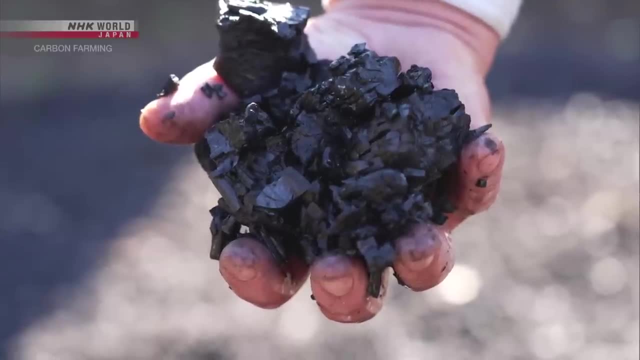 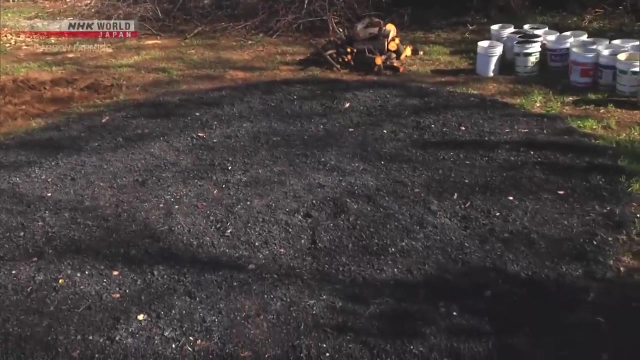 Before the wood is completely burned, water is poured over it and the biochar is ready. Before the wood is completely burned, water is poured over it and the biochar is ready. Burying this biochar will trap atmospheric carbon into the earth. 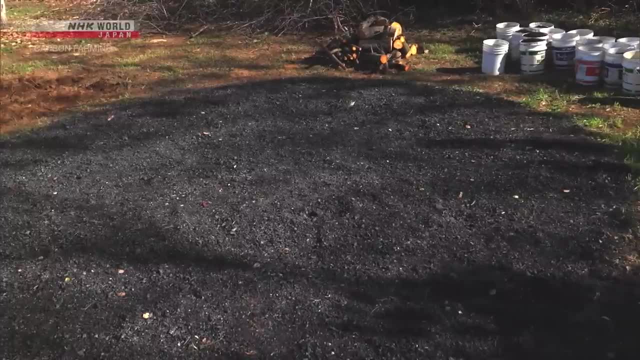 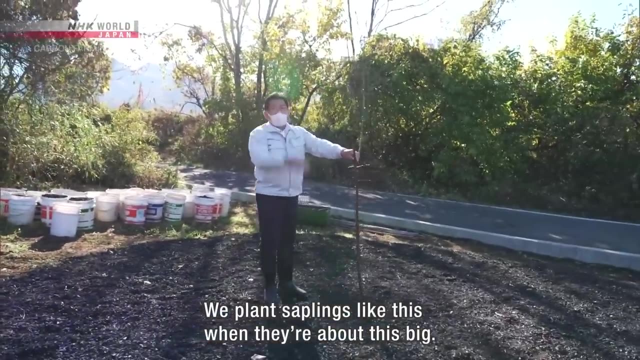 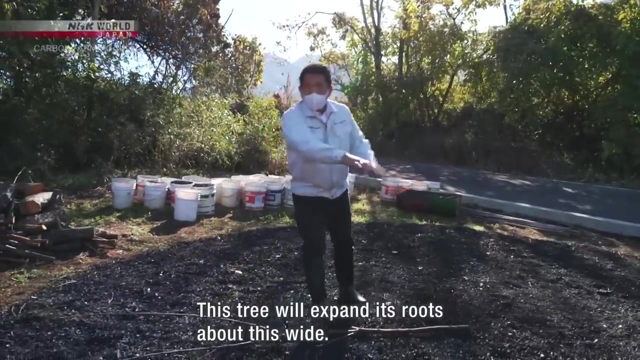 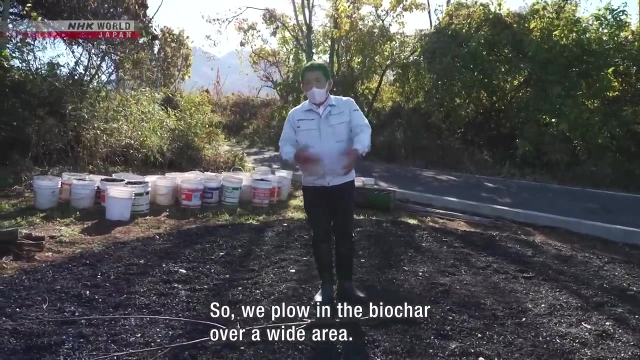 and help regenerate the soil. at the same time, This will allow the biochar to expand to the entire surface of the earth. This will allow the biochar to expand to the entire surface of the earth. After 5 to 10 years, the biochar will have a lot of fresh wood. 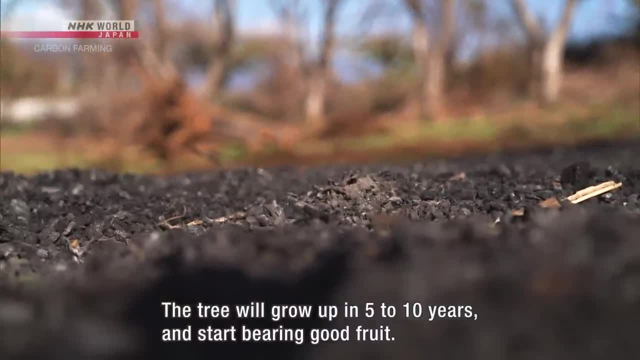 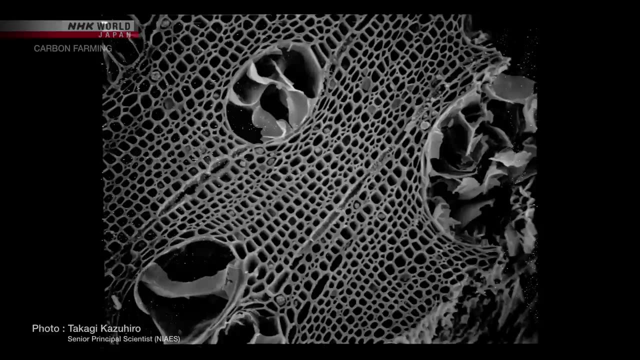 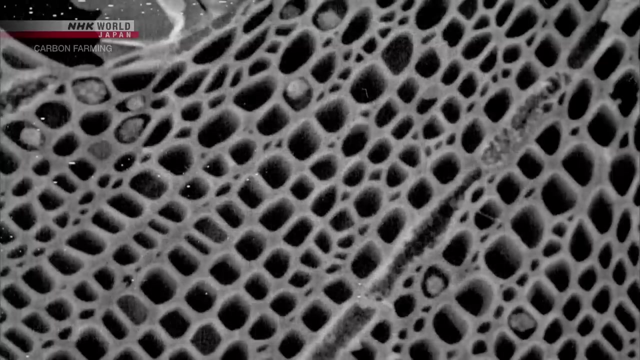 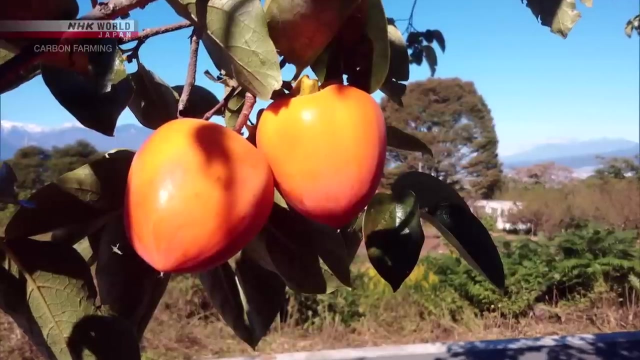 After 5 to 10 years, the biochar will have a lot of fresh wood. Biochar's ability to improve soil comes from its porous structure, which excels at both storing and draining water. Old trees are often thrown away as waste, but Amemiya makes sure they are given a new life. 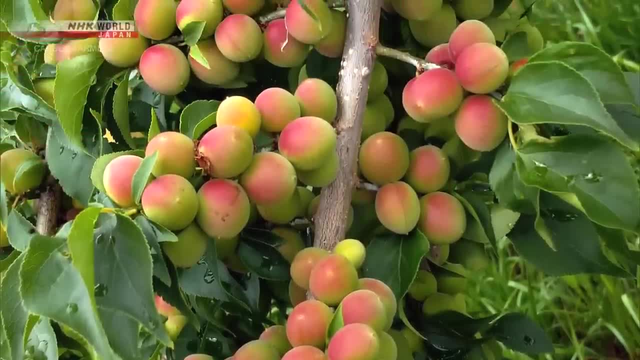 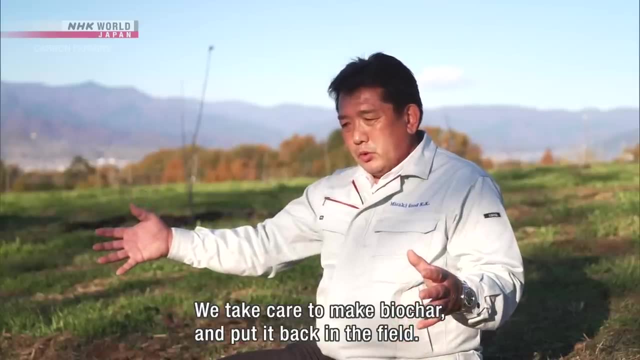 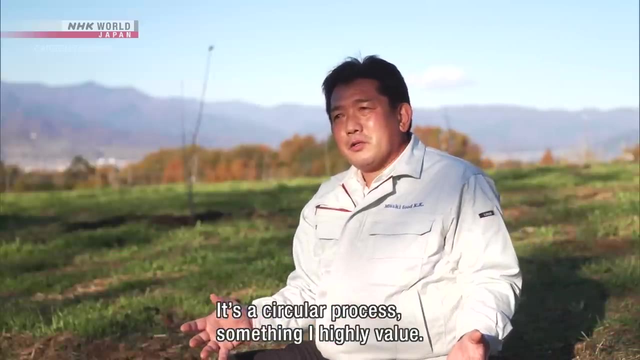 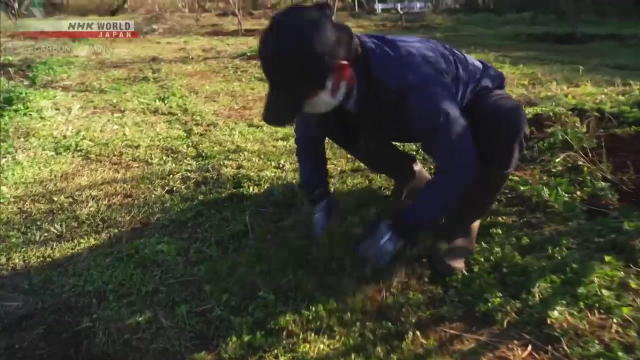 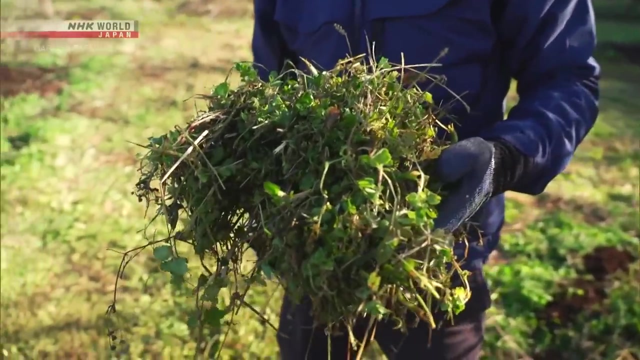 His fruits are very popular for their shape and flavour. But it's not just biochar. They remove weeds and use them to fertilise the soil. They also use compost. But it's not just biochar: They remove weeds and use them to fertilise the soil. They also use compost. 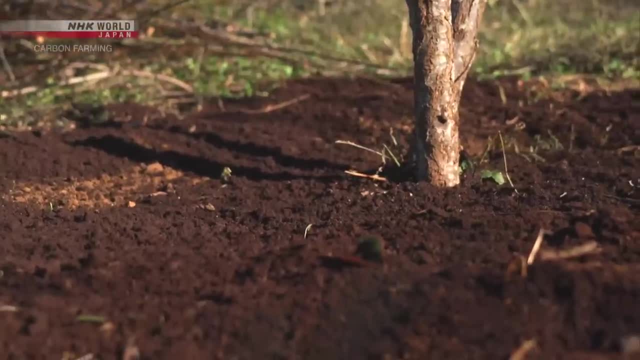 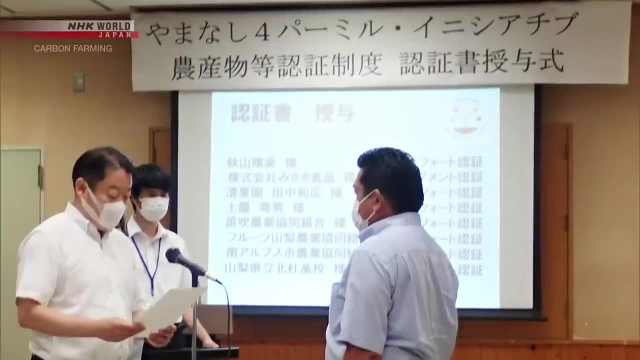 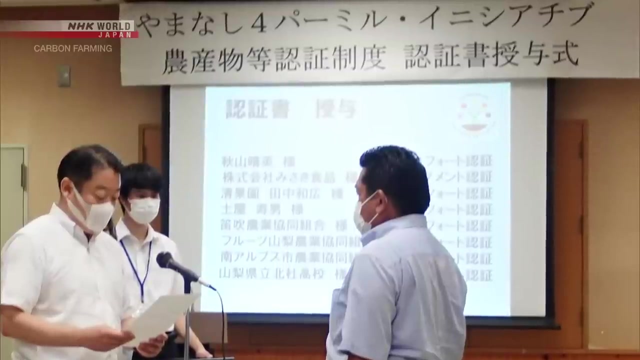 And all kinds of other farming methods to store carbon in the soil. He and his group have won recognition for their contribution toward a carbon-free society. Yamanashi Prefecture has certified their farm products under its 4 per 1,000 initiative. 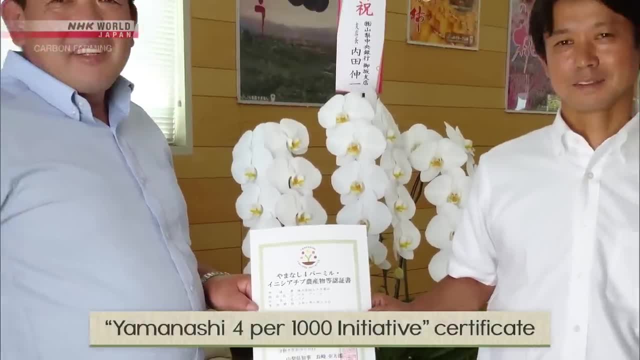 To receive this certification, they had to trap at least one tonne of carbon in every hectare of soil. However, there are other numbers that mark the Identification Classic. these cars are the most popular in Japan. in that respect, Yamanashi Prefecture has certified their carbon-freearentail République in 2020.. Now N personneness is no longer a part of Nj recognition. They have lived for many years in this land, But Nj is the one to move my focus to Japan. My current job is a good cat in the sky. The Nidis clean. 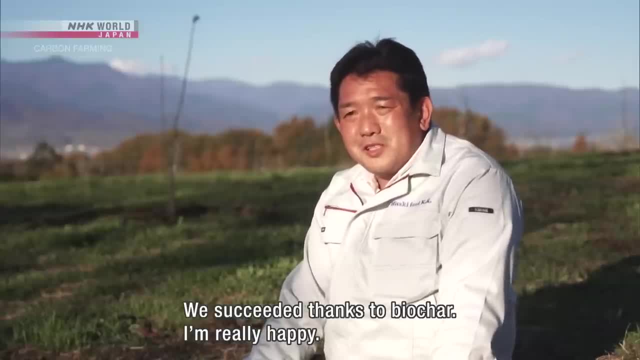 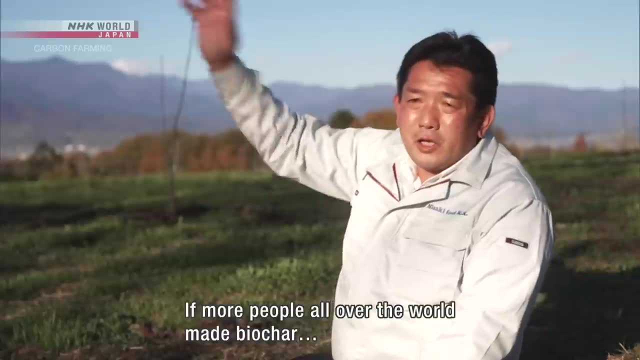 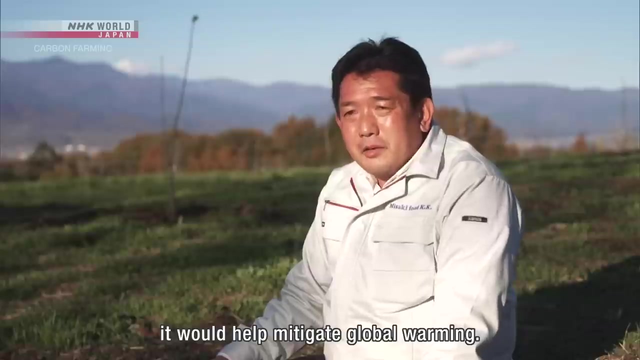 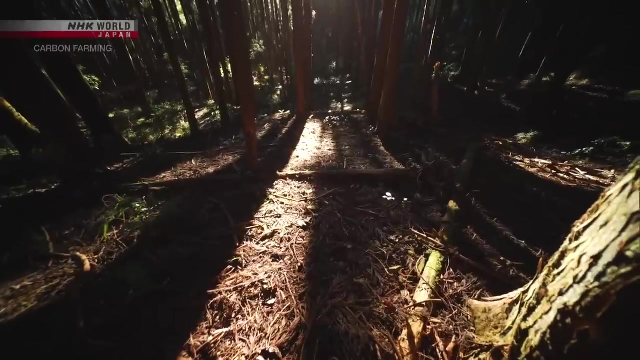 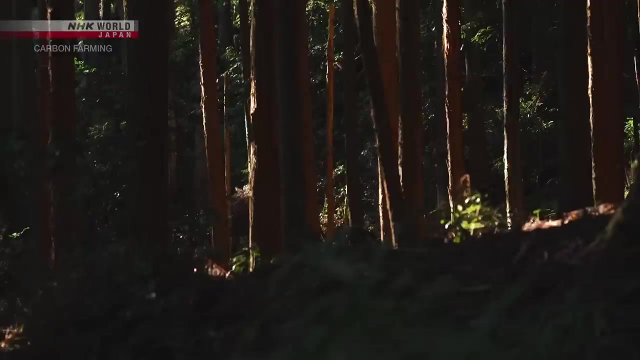 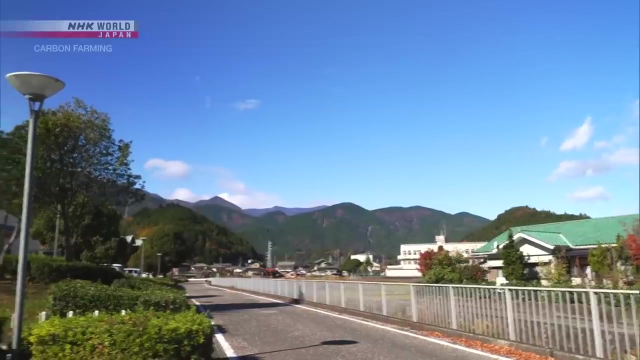 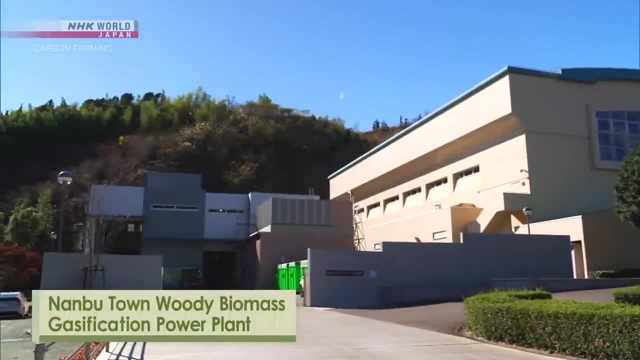 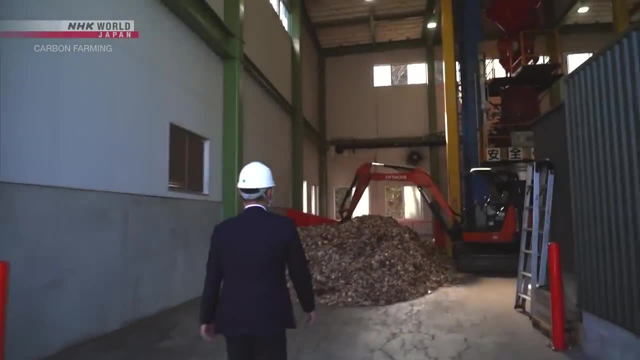 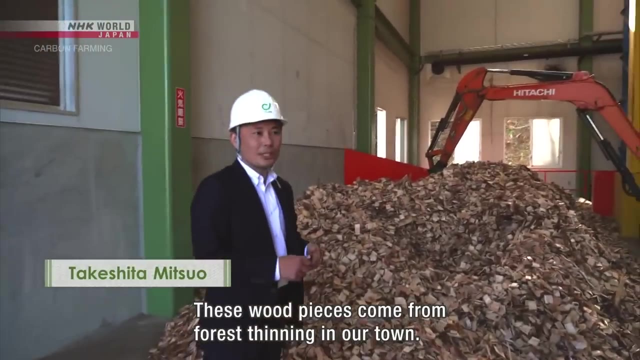 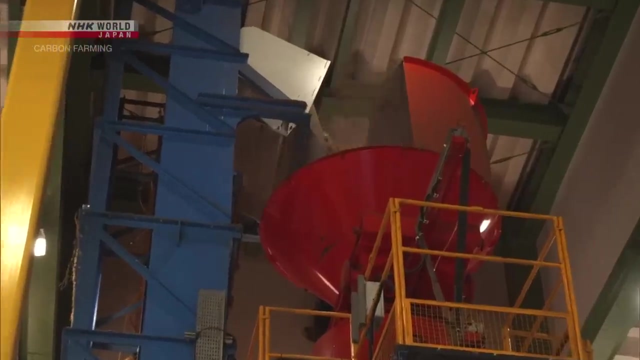 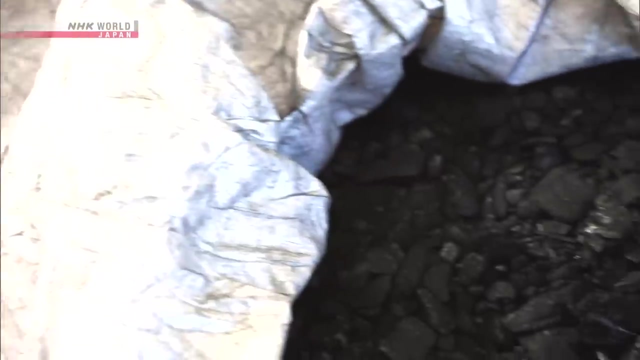 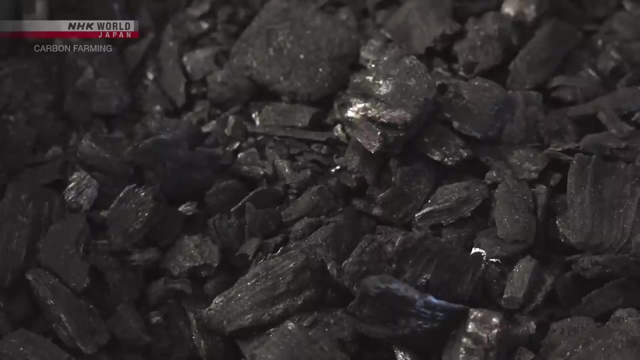 power plant. lumber from forest thinning is used to generate electricity. it started its operation in May 2021. they hope to harness the energy needed for local consumption. burning wood for power generation creates biochar as a by-product. at first, biochar was nothing more than industrial waste. its disposal was extremely costly. 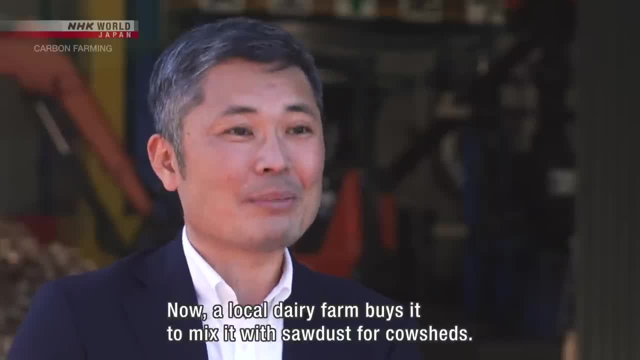 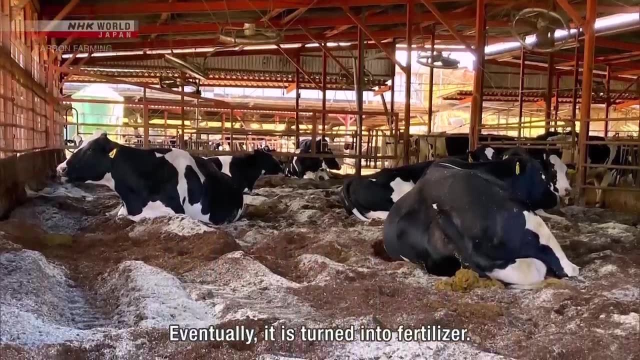 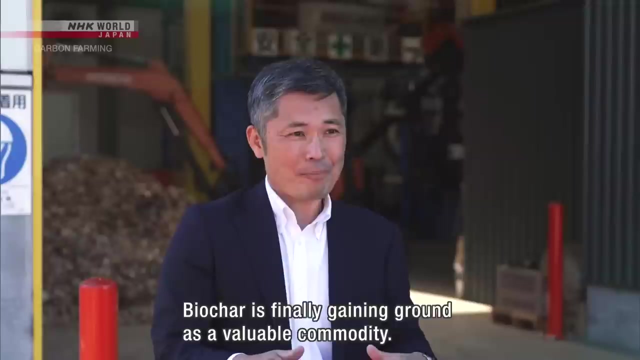 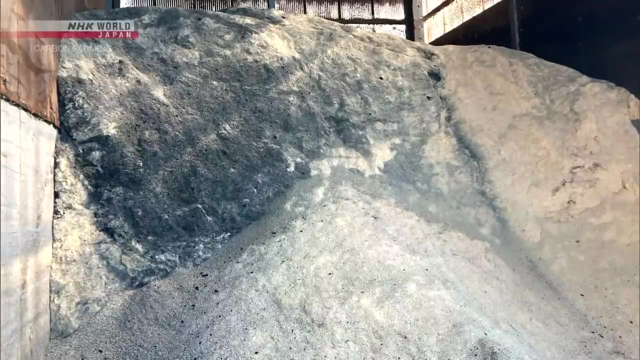 牽引もised タイナノファーマーすべてのフォトページで いるものにも関心がある. biochar provides extra income for the dairy farmer and the fertilizer could in turn benefit other farmers. フォトソファーマーが増えたために バイオチャーは今後多くの財産を生産したり増えたりなるが で全部の財産を加えながら 財産を生産しているための財産を生産の財産的な財産は失敗します。. 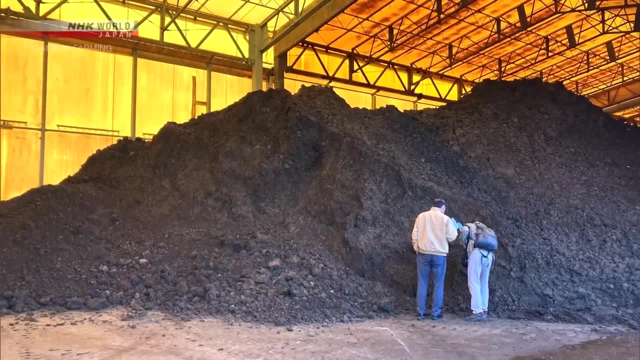 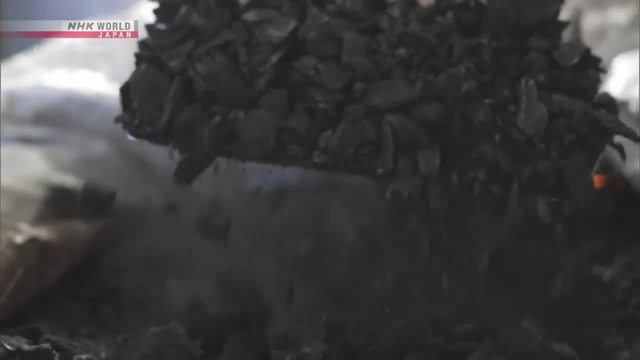 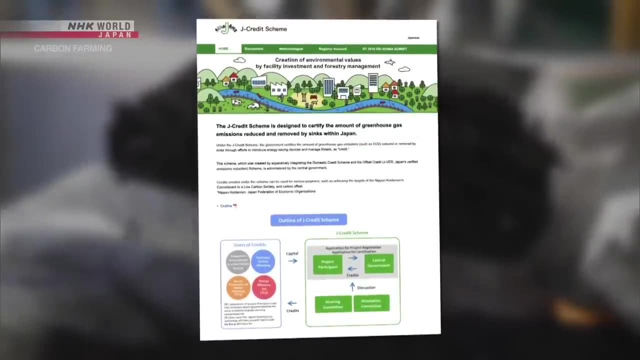 biochar provides extra income for the dairy farmer, and the fertilizer could, in turn, benefit other farmers. Once thrown away, biochar now creates a local circular economy. What's more, a new tailwind is helping to further promote it. Japan became the first country to certify biochar as credit to offset carbon emissions as part of its J-Credit scheme. 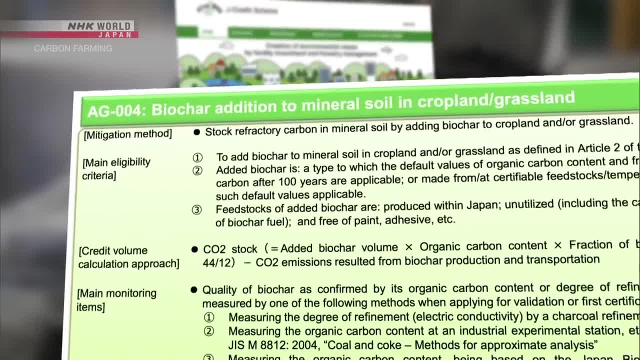 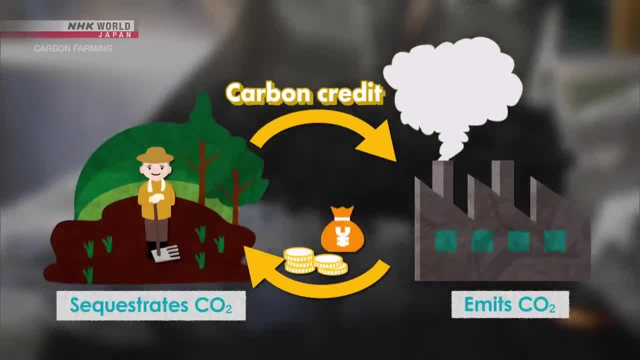 The credit can be traded on the local and global carbon exchange market. Farmers can use biochar to sequestrate or remove carbon from the atmosphere, the amount of which can be turned into credits to sell to companies that are looking to offset their emissions. 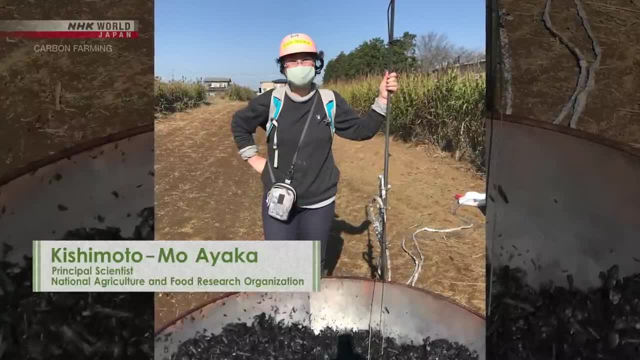 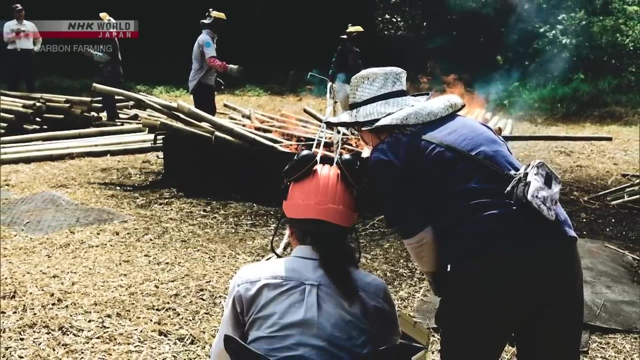 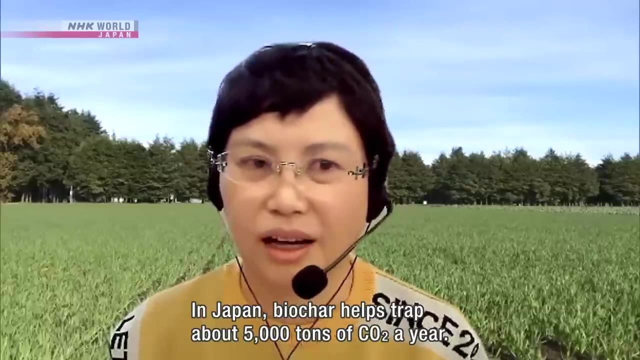 Kishimoto Mo Ayaka is a biochar researcher. She says the credit scheme will create a virtuous cycle that benefits both biochar-using farmers and the environment. I think that the amount of CO2 on the national level is about 5,000 tons. 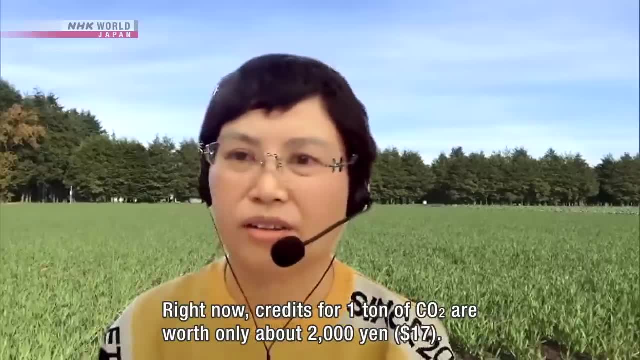 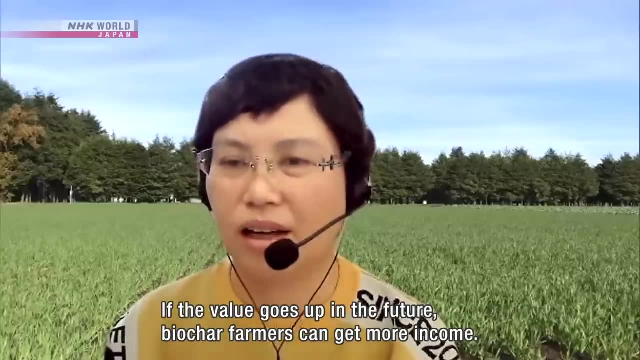 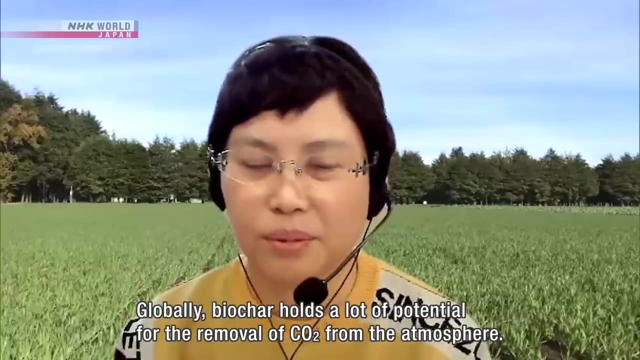 In Japan we use about 2,000g for 1 ton of CO2.. In the future in order to increase the value of the credit, I believe that will benefit the farmers most. How much potential is there in the world? There is a standard 0.3 to 2.1 trillion yen, That's about 3 billion yen. When you go that far, you can't do it anywhere. When you go that far, you can't do it anywhere. 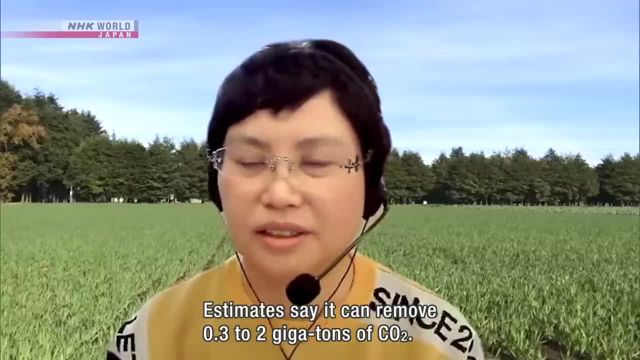 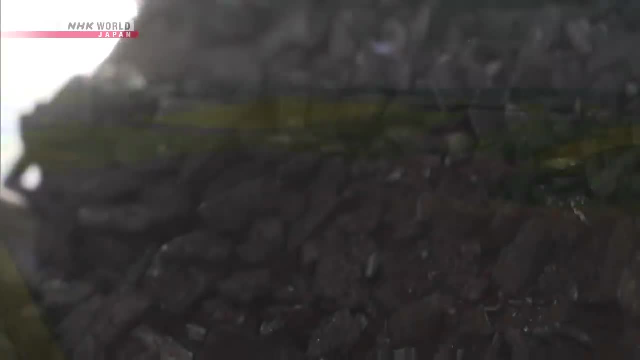 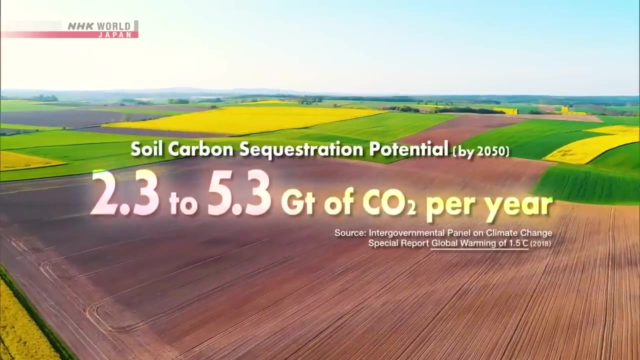 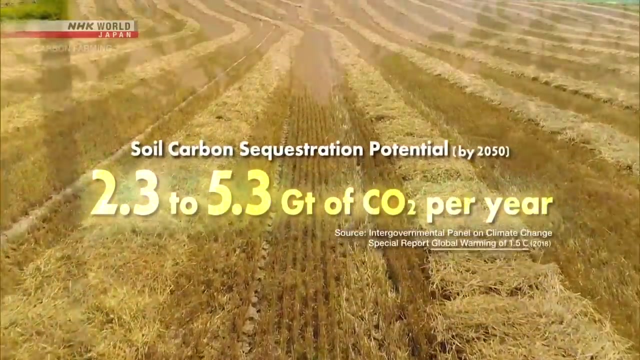 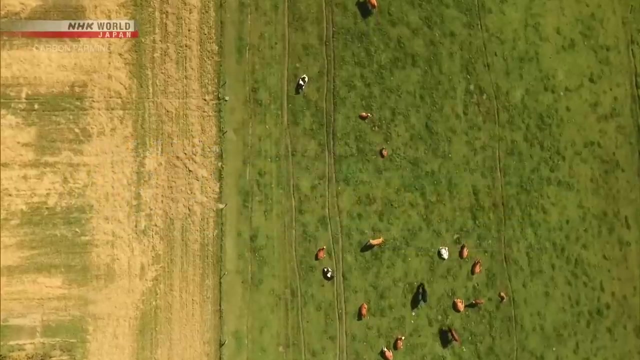 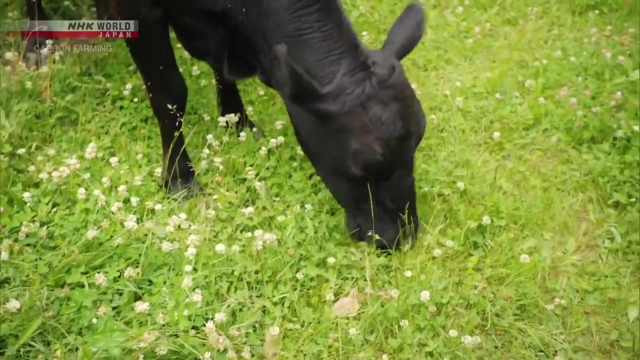 The IPCC reports that the potential amount of CO2 that can be captured and stored or sequestrated in soil is estimated to be over 2.3 gigatons per year by 2050.. As we aim for a carbon-free society, hopes are heightening for the possibilities of agriculture. 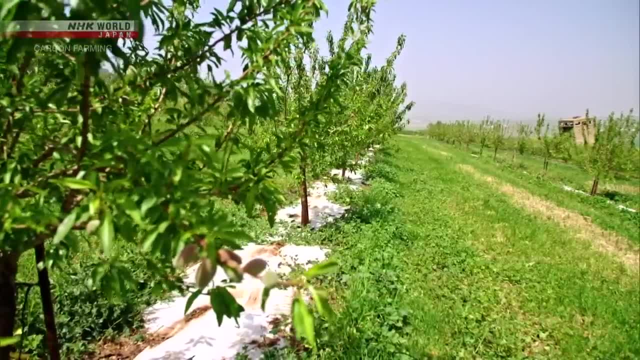 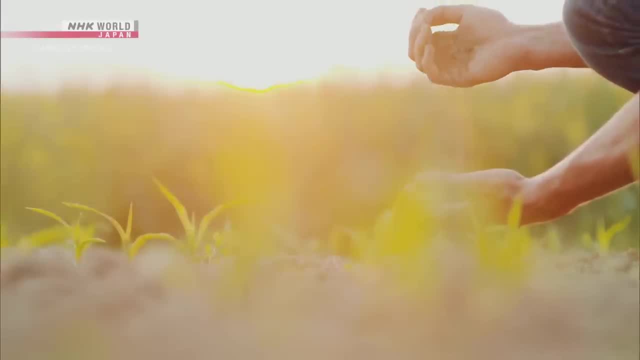 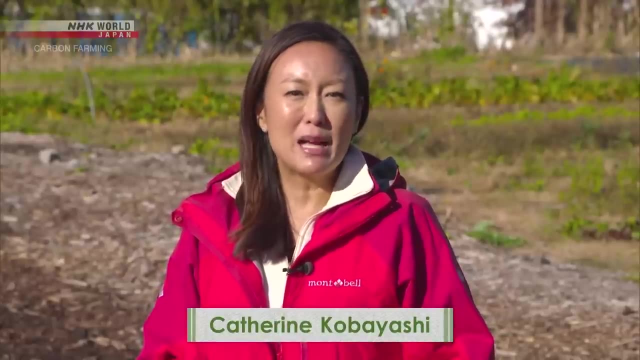 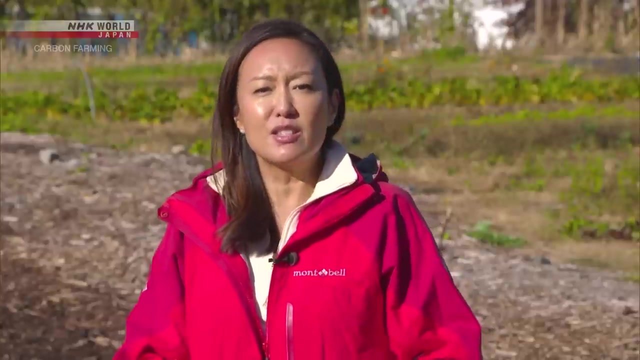 and carbon farming is bound to birth new trends for the future. People are blazing new trails toward a more verdant future. The farmers we met say our current way of living disrupts the workings of the natural ecosystem that sustains us. Consider this: there are nearly 8 billion people in the world.